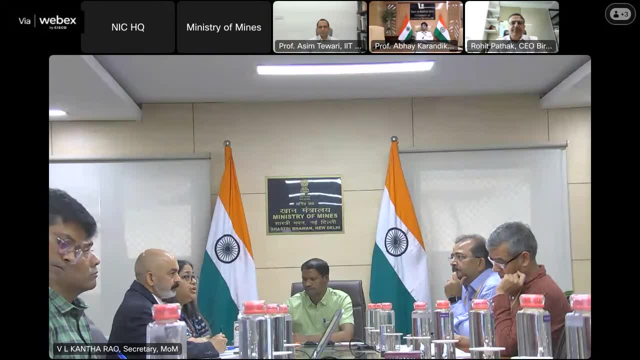 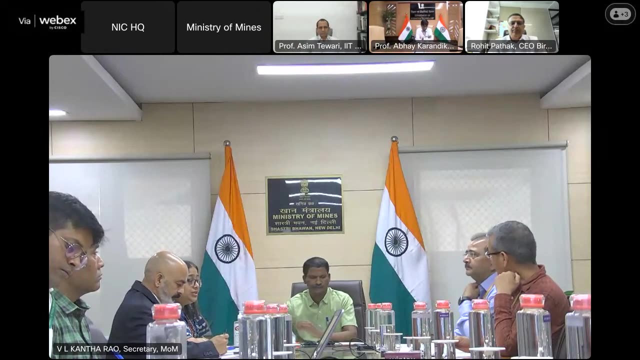 who have been dealing with the startups in the mining sector for their experience sharing with us. We are also having on board with us today the two startups who have been funded by us in the in year under the SNT prism scheme and I hope that this scenario will provide a good opportunity for 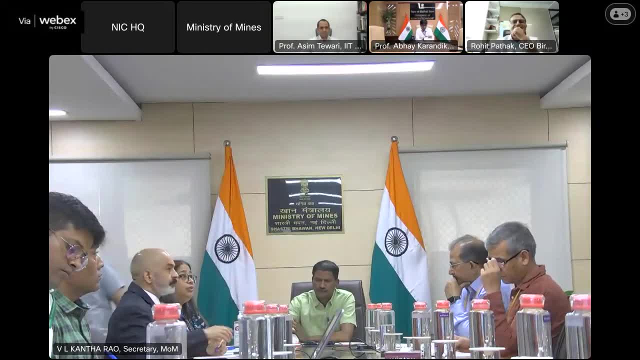 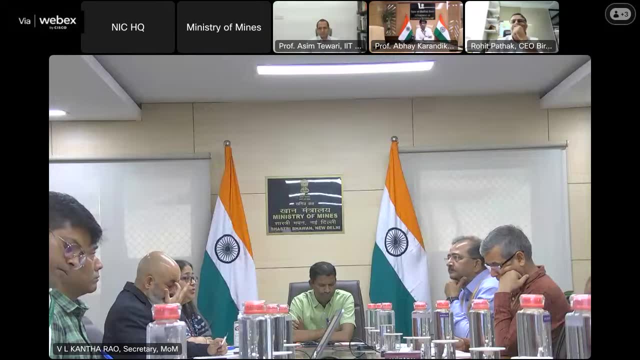 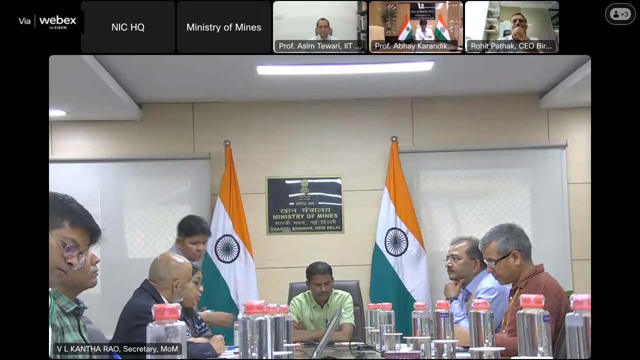 all of us to deliberate further on the issue. I would request all to be connected in the webinar we will be having the- we are having the polls- and where your responses to the same would enable us to take this initiative further. Also, the chat box is open and you can send your messages on. 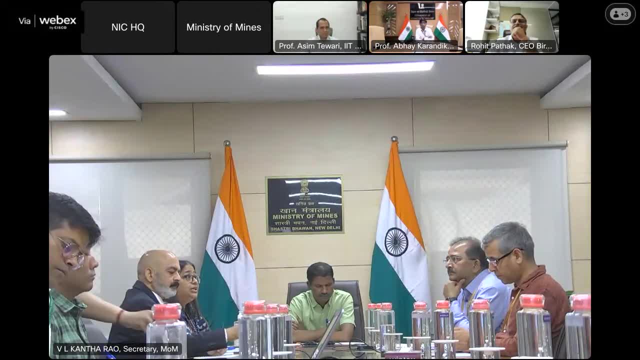 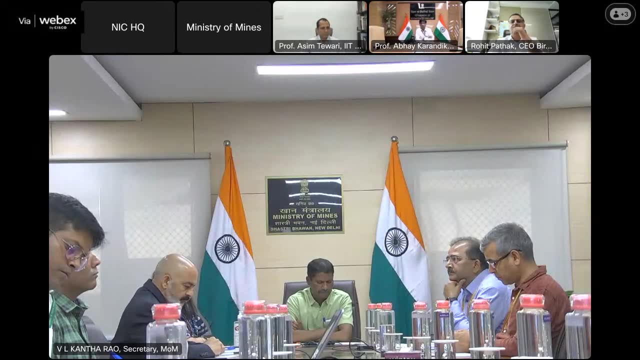 the chat box, though at the end of the session there will be a question and answer session, but in between, in case, if you want to ask something, please write it on the chat box. we have our experts sitting there to respond to it With these words. I would request our secretary to please. 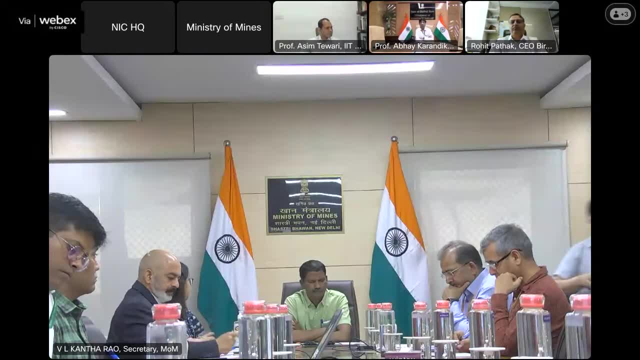 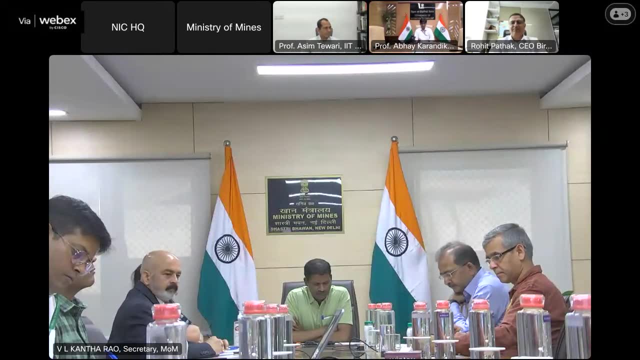 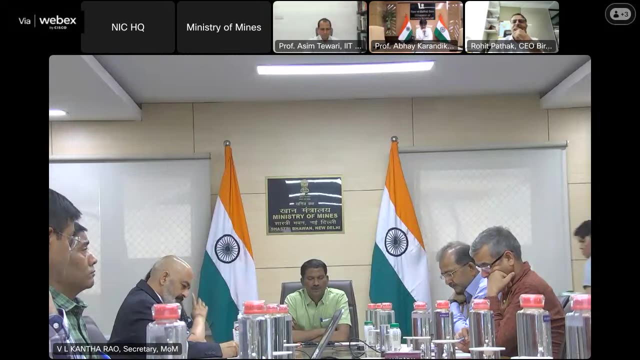 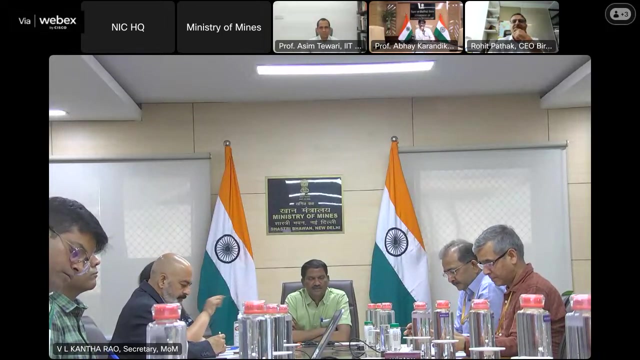 open the the stuff welcome. Thank you very much. I want to welcome all the participants for the mining startup webinar today and, most importantly, I want to especially welcome the chief guest of today's webinar, professor Abhay Karandikar, who is extremely busy today and I'm so. 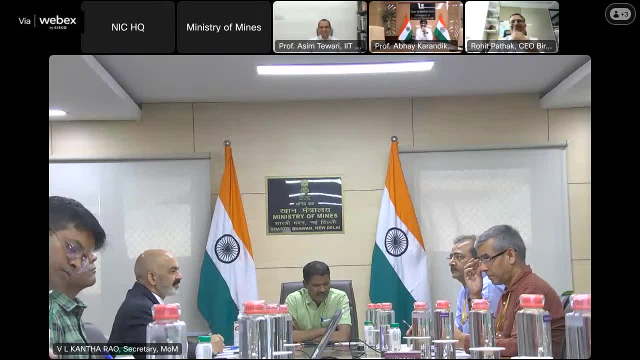 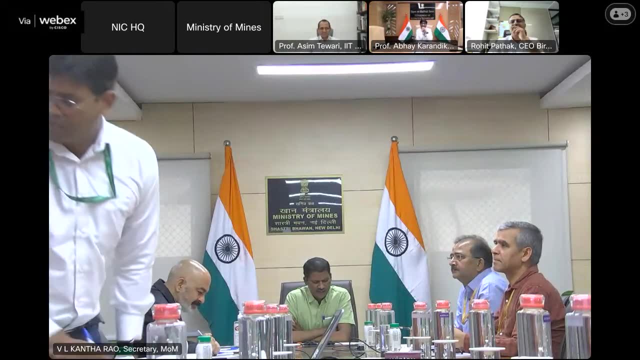 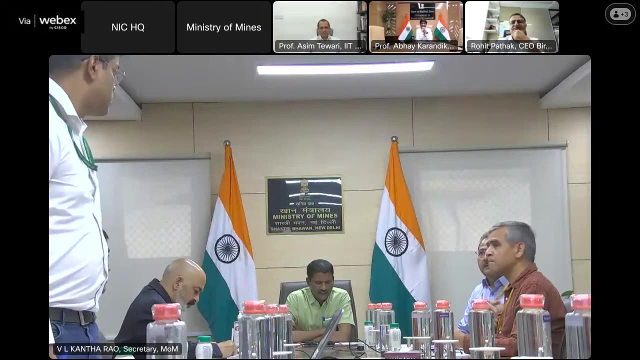 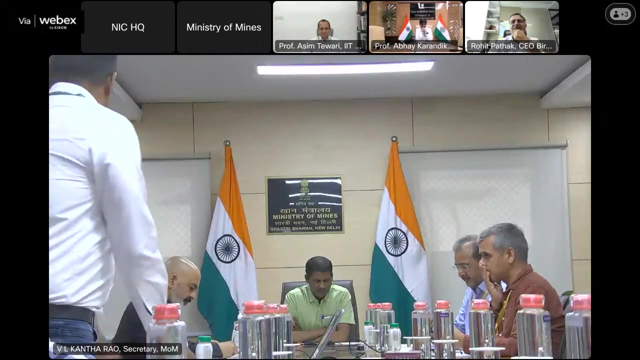 happy to you know, see him smiling and ever smiling. who has given us time today to be part of this. I had the opportunity to work with professor Karandikar for the last one and a half years while I was in the telecom sector, but now in this, when he has moved from. 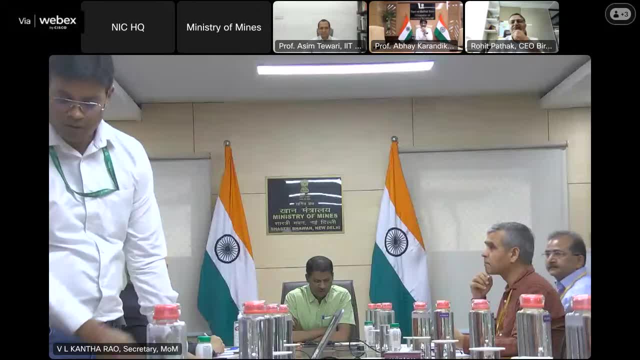 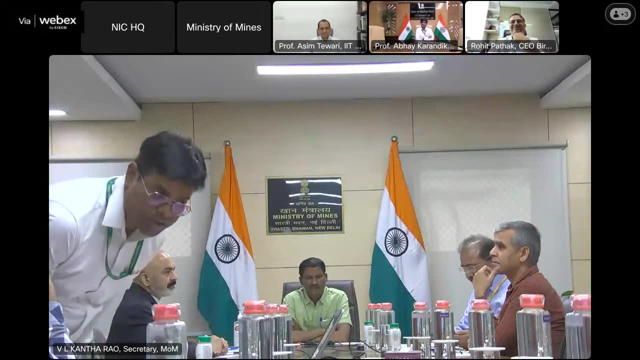 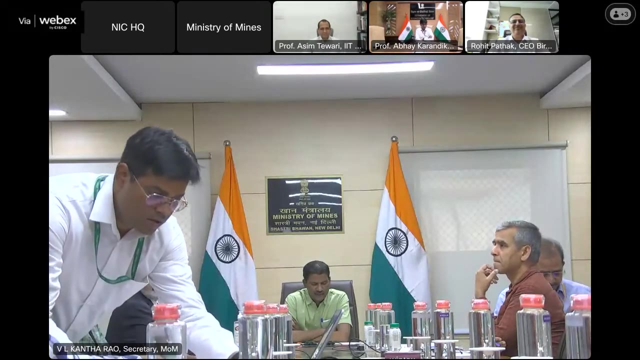 IIT Kanpur to DST and I've moved from telecom to mines. it is again a different kind of interaction with a lot of scope and opportunities that he presents. I am so happy that professor Karandikar is going to give us the inaugural address today. 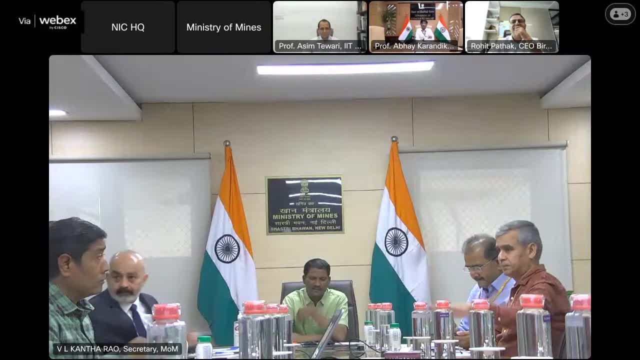 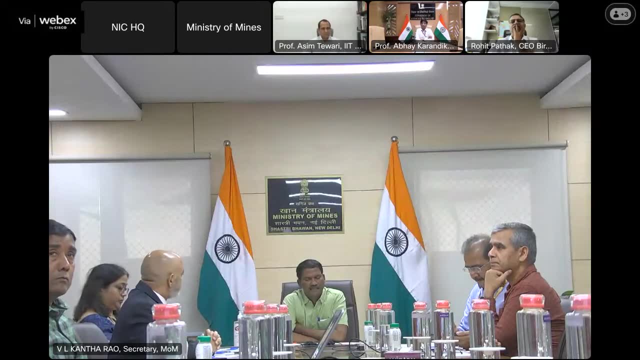 the idea of having this seminar, the idea of having this seminar through a webinar mode, is that more and more people can be connected. they need not travel all the way here, and I am told about 200 people are registered for today's event, most of them startups. 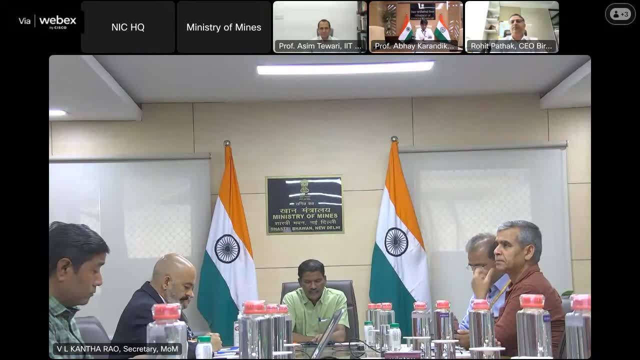 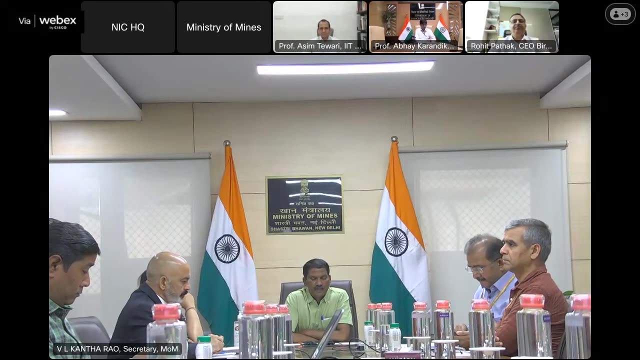 startups. It is a good indication because startup companies have not heard of mining sector much. We made a small beginning this year in trying to attract startups into the mining sector by giving them some funding. For the first time we have given funding to six startups. Till now we have been doing a lot of innovative work through the R&D organizations. 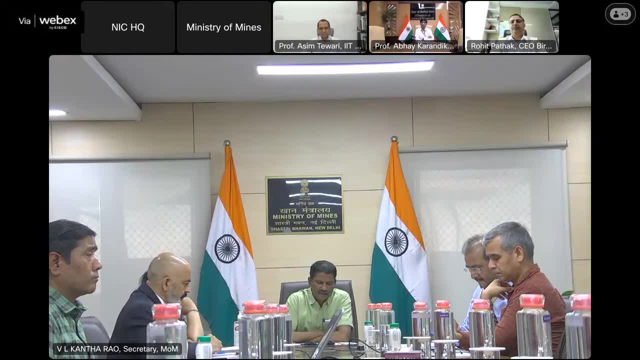 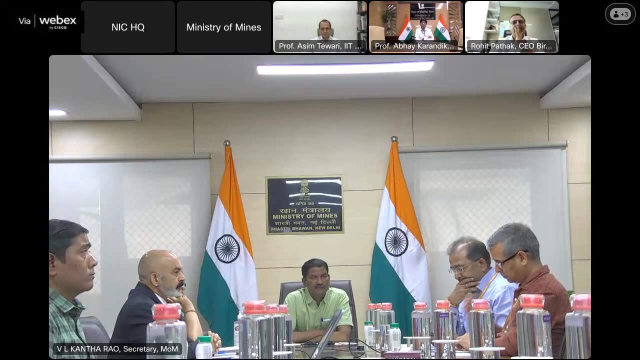 of the Government of India, like the CSAR labs and institutions under our own ministry, like the Aluminium Development Center, so on and so forth. But I am sure you will get to hear something from the startups also in today's seminar. They will talk about the 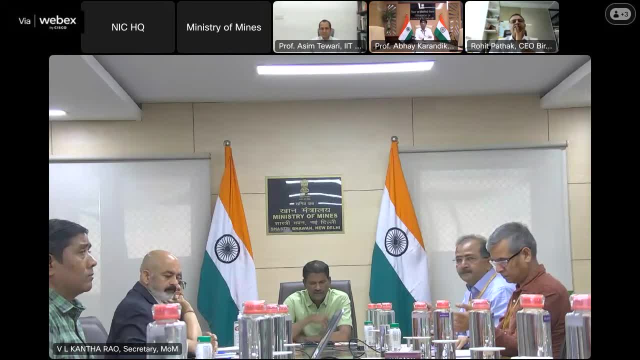 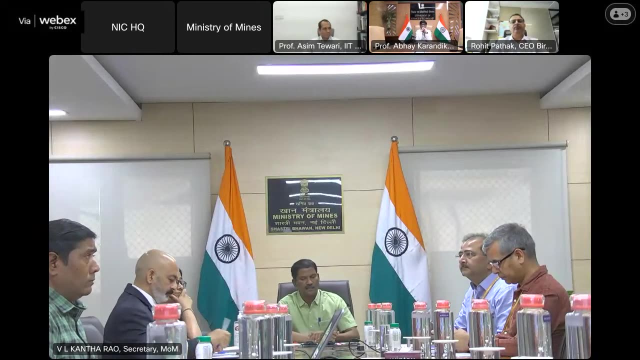 story. They will talk about their experience. Now, having started the introduction of startups in the sector, we planned to increase the scope and the funding for startups this year. Therefore, we issued an advertisement, a call for proposals, for which, as Majay has mentioned, 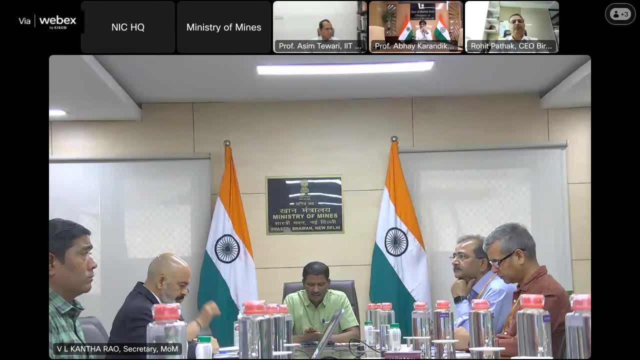 the last date is 30th of April. We want to reach out to those who want to participate in the cyber industry. We have been working on this issue since the very beginning, So we are looking forward to working with you, Thank you. 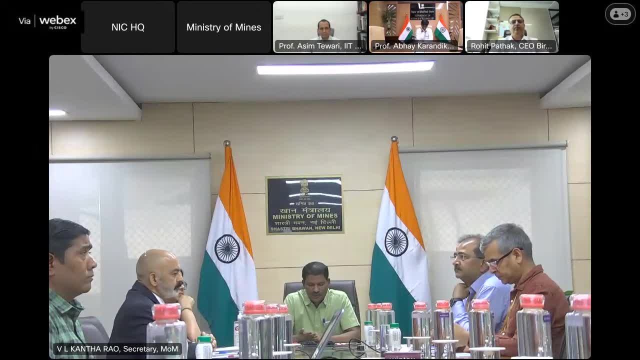 more and more startups through the academic institutions, through the incubation centers, and to the startups directly through webinars like this, And Professor Karandikar has assured us that he will help, through the network of institutions that are under his ministry, to reach out to incubation centers. 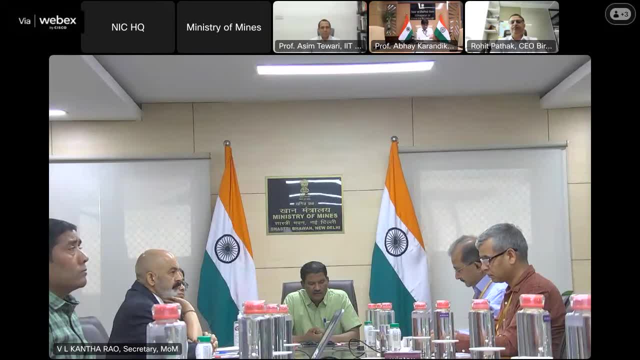 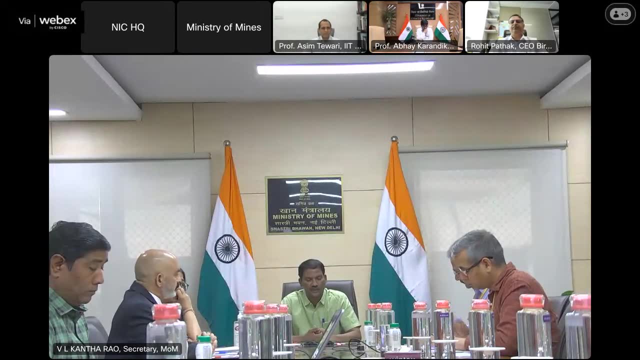 and startups for requesting them to look at this sector, which is considered a very traditional sector, but now it is changing. with the coming in of the importance of critical minerals, the processing of critical minerals, the recycling of some of these minerals, It is becoming a very, very important. 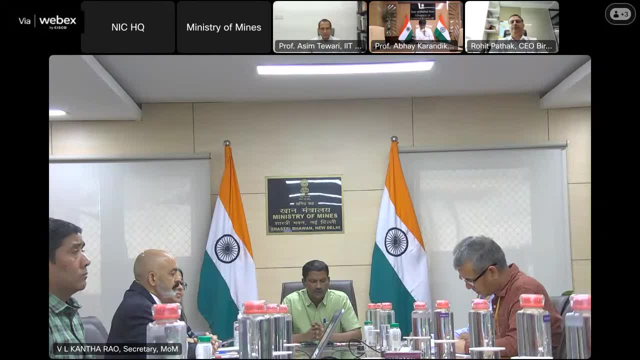 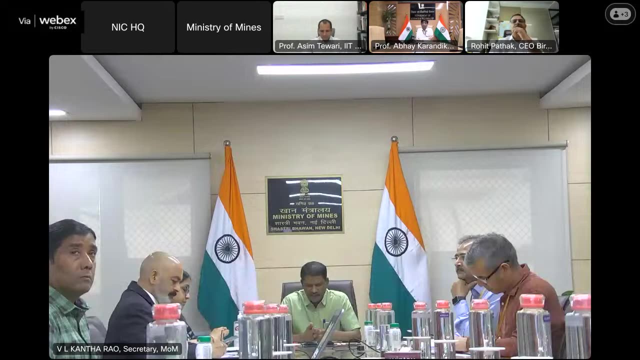 sector of future. So, with this idea, I would request all the participants in today's seminar to explore new opportunities, ask a lot of questions and see what are the areas in which they can venture into. In fact, some of the industry leaders. 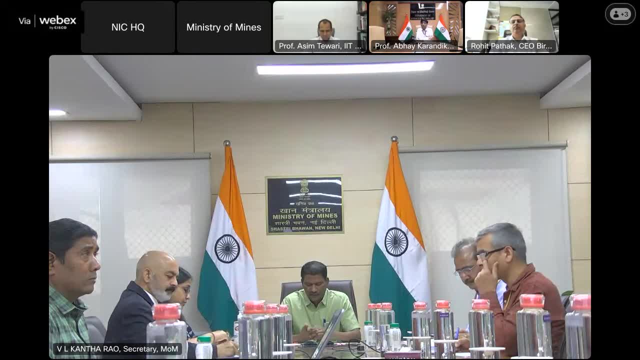 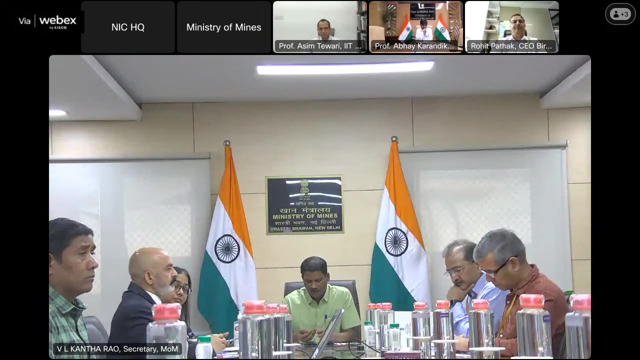 are also participating in today's seminar where they can actually talk about the problem statements. You can start working on this problem statement. In fact, one of those statements which my ministry has, or those again have some clear has, is actually the processing of geological data. we have vast amount of 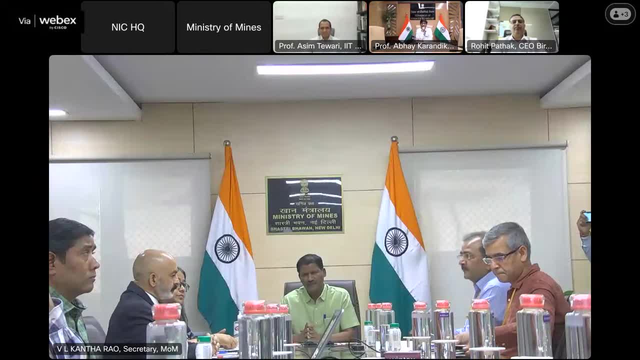 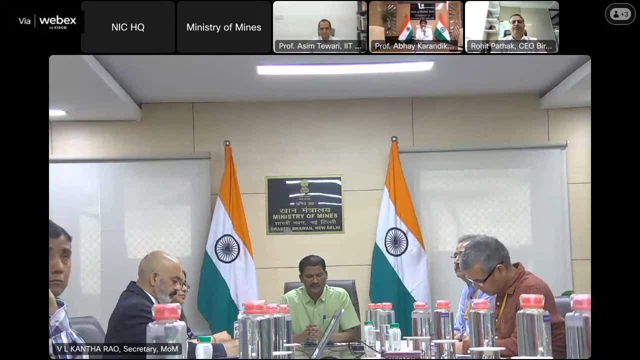 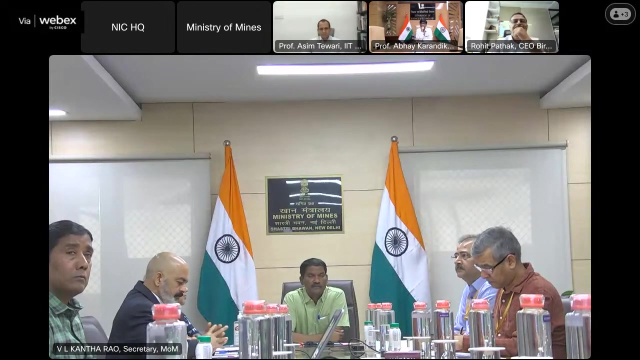 geological data for all the 33 million square kilometers- 33 lakh square kilometers of India's land and also another 20 lakh square kilometers of offshore area. all the data needs to be analyzed to find good inferences as to where the mineral can be found. so in this context, secretary DST has also said: 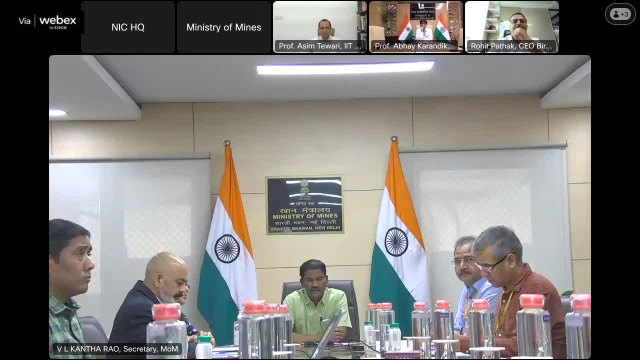 that we can do some kind of a hackathon. he had good ideas on that, so we will be doing a lot in the coming time in doing innovative work in the mining sector, starting from data analysis to actually processing of the minerals found under the earth and under the sea. so let us 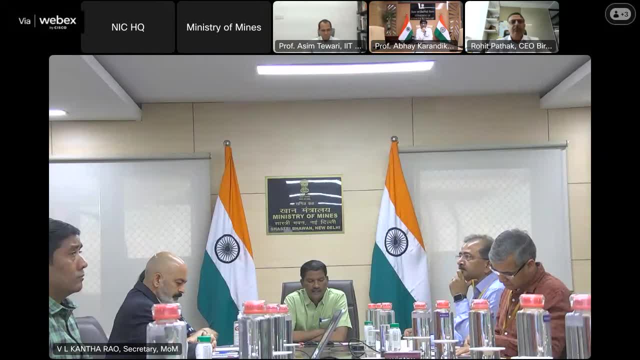 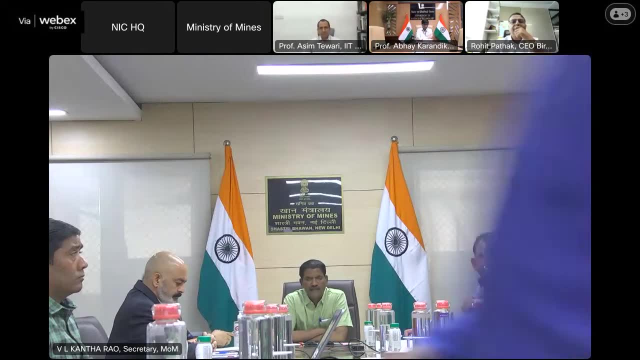 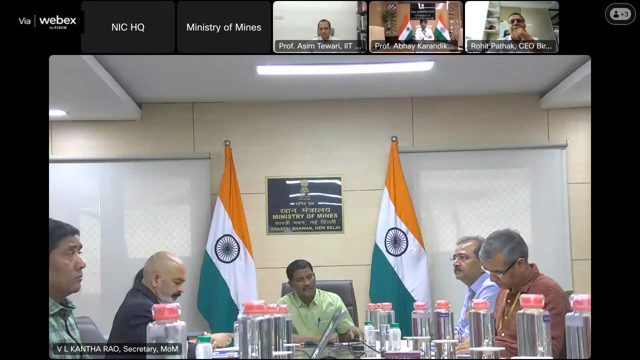 go ahead and move on to the next slide. make use of the opportunities that are coming up and also make use of the support that the government is planning to provide and submit good proposals by 30th of April and make sure that we are all part of the 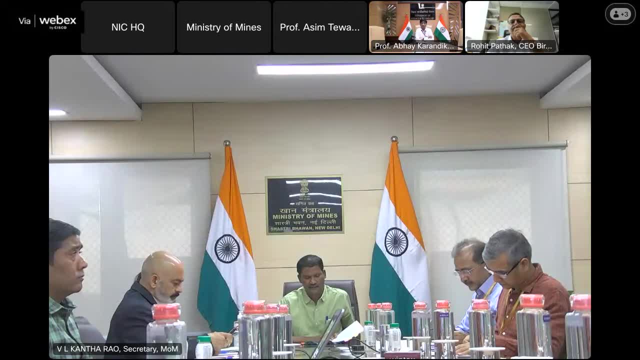 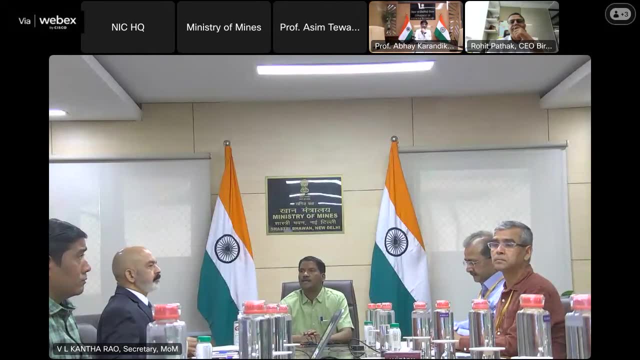 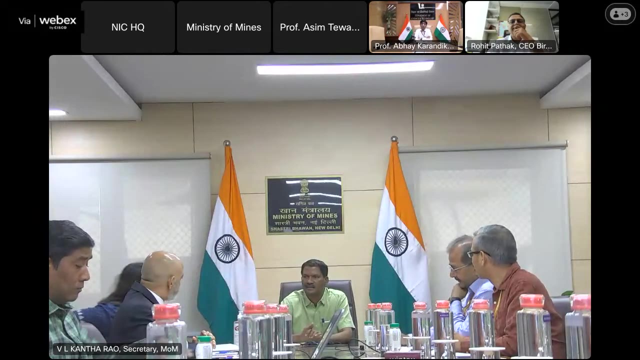 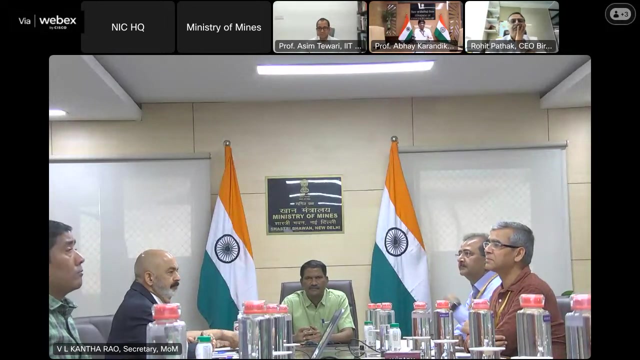 the journey for an Atmanirbhar Bharat in the mining sector. thank you very much. thank you, thank you. no, no, I now request Secretary DST to please inaugurate the seminar. thank you, thank you very much. I think, Mr Kantar Rao. I think. Secretary. Ministry of. 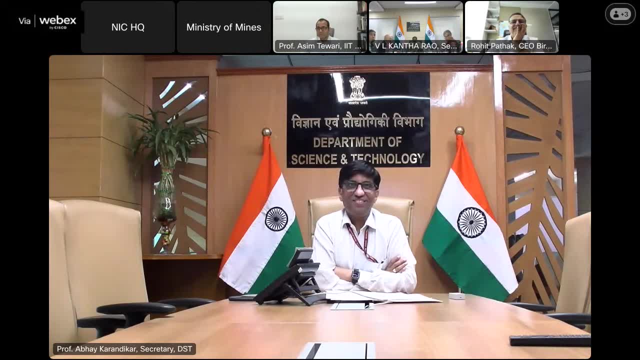 Mines, all the colleagues in the Ministry of Mines, my other distinguished colleagues from academia who have joined. I see Professor Asim Tiwari from IIT Bombay and other participants from industry and startups. Let me first begin by congratulating the Ministry of Mines for taking a very, very important 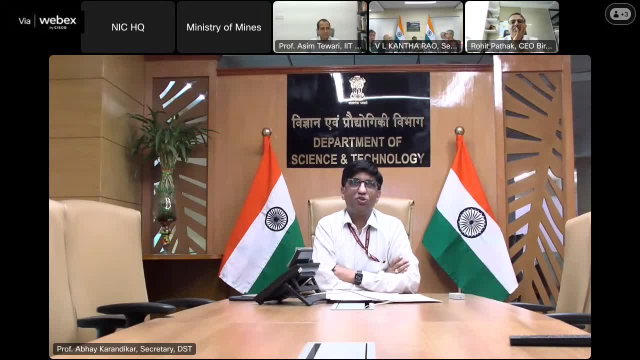 and a much-needed step to support and nurture the startups in the area of mining. And I mean this is really a laudable effort because, as I think Mr Kantarov mentioned, that mining has been considered as a very traditional area in India. 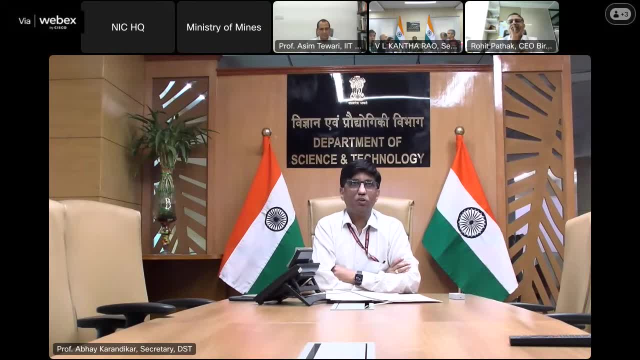 but elsewhere also, There has been a significant use of technology not only in the process of extraction, separation, chemical processing, et cetera, but also in data processing and computational material science as well. So there is a huge possibility of developing a startup ecosystem in one of an important area of the deep tech sectors. 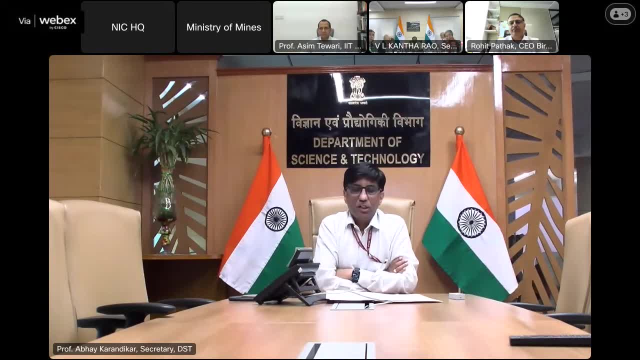 that is, you know, very critical minerals. The department of science and technology has been playing a critical role in nurturing the startup ecosystem. We have been setting up incubators and centers of excellence across all the academic institutions for the last several years, Since year 2016,, when the government of India had launched the startup India initiative. 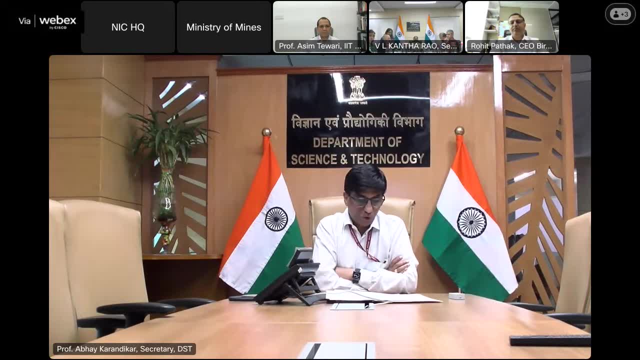 the Diese, The DST has set up the scheme called NIDI, which is National Initiative for Developing and Harnessing Innovations, And under this NIDI umbrella scheme there were many programs like NIDI Prayas or NIDI Centers of Excellence and NIDI Startup Support System. 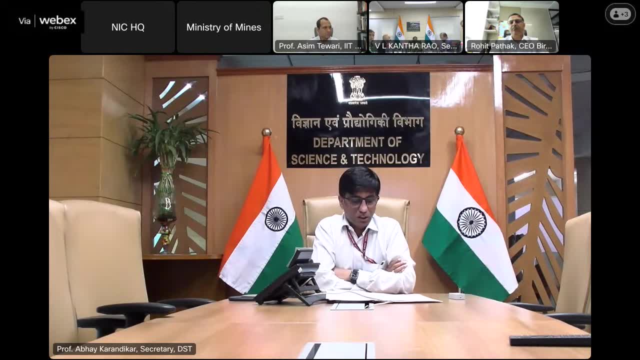 And overall, I think over the last six, seven years NIDI program has supported 12,000 startups in almost 170 incubators across academic institutions, which includes IITs and IIC and IIITs and so on. Now, as you know that India has emerged, the third largest startup ecosystem in the country, 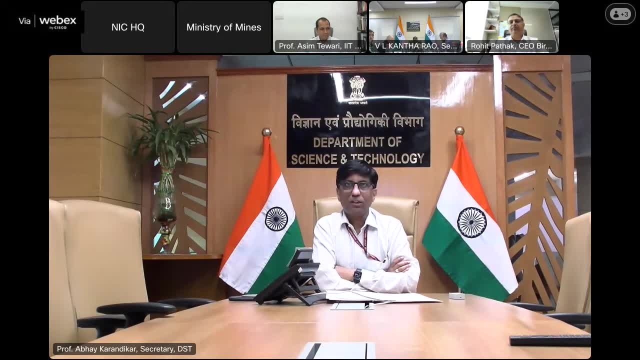 there are more than 1,00,000 startups, almost 1,20,000 startups. However, only I think, 7,000 to 8,000 startups are in the deep tech area, And one of the important deep tech area, I believe, is exploration and processing in. 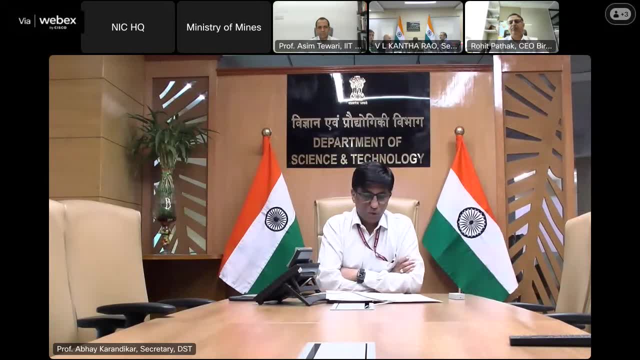 the sectors of critical minerals. And critical minerals, as you know, play an important role in many sectors, particularly like in clean energy transitions or even battery materials. for you know, for you know, for electric vehicles. India has, in fact, clean energy targets. you know, if you look at it, either in the 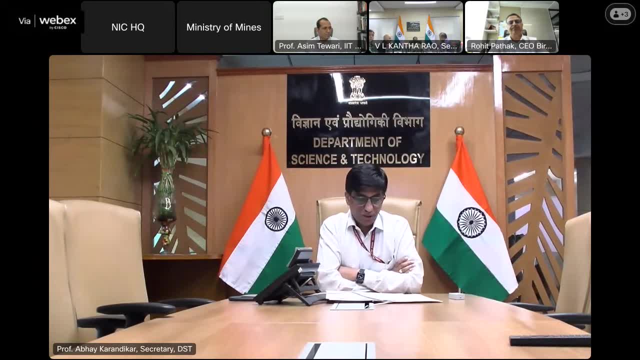 form of electric vehicles or in the form of the renewable sectors. the demand for these materials are actually quite significant. Now, rare earth elements are also very crucial strategic material for the country. India in fact has the world's fifth largest- you know- rare earth mineral. you know energy. 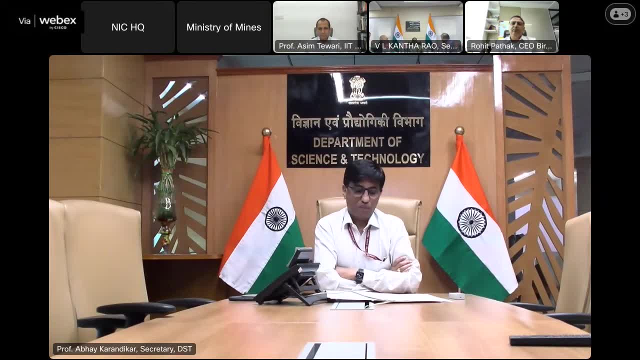 industry And that's a big deal And that's a big problem. So, you know, the US has a very high level of energy reserve. However, the process of extraction, separation, as I mentioned, and then converting them into metal alloys has been traditionally, you know, found to be very cumbersome, has been using 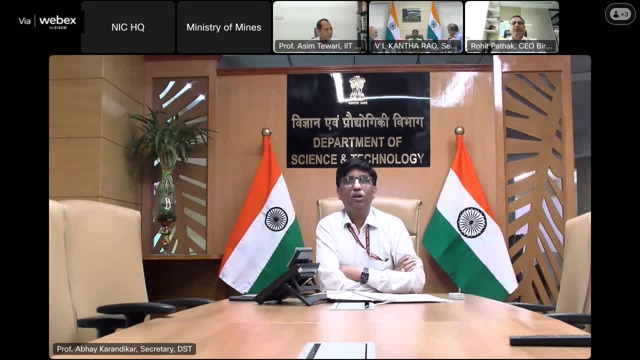 you know hazardous technologies And I think there is a need for innovations in these sectors to have, you know, environmental friendly, non-hazardous, you know technology which can be developed indigenously. Okay, Uh, at the same time, I think we also need to give emphasis on the computational material science, the use of new technology such as machine learning and artificial intelligence, And I see in the program, uh Professor seems to worry, is, uh, you know, going to give a talk in this area? 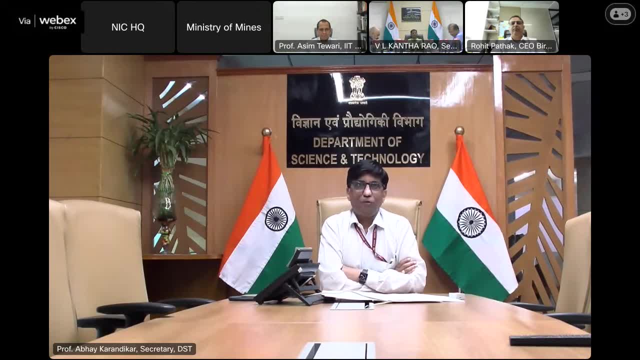 So I see a significant opportunity for the deep tech startups to explore, Um, this entire uh uh field of um uh materials and minerals, uh, you know, to make uh uh not only a national impact but uh uh also really make our country self sufficient. 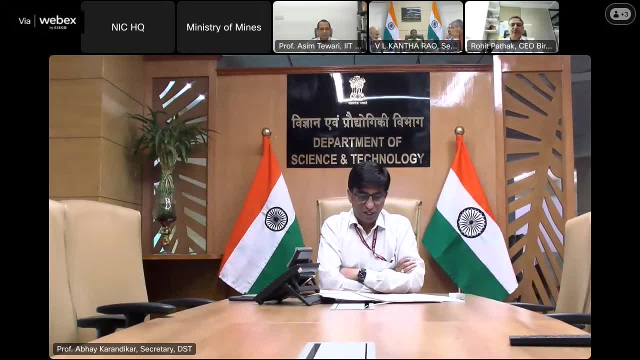 Uh. today we are standing at a pivotal junctions and we are very well positioned to steer our efforts towards the development of indigenous technology Uh, given the fact that we have a very positive and enabling environment. and, in this context uh, I think uh this uh uh supporting the startup scheme uh is uh also forms 1 of the important steps uh of the government uh regarding its commitment to fostering research and innovations uh in the- uh you know- sectors of mining and mineral processing from the Department of science and technology. 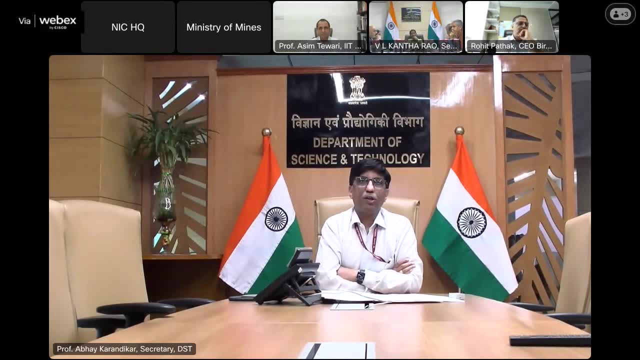 Uh, we would like To definitely explore the possibility of uh collaborating and partnering uh with the Ministry of mines to uh strengthen uh the initiatives uh, which is uh like the prison that is being launched uh today. uh, as I already mentioned, that uh through our centers of excellence and the incubators, we have a large network of incubators and those incubators can actually be tapped uh to nurture uh the startups. 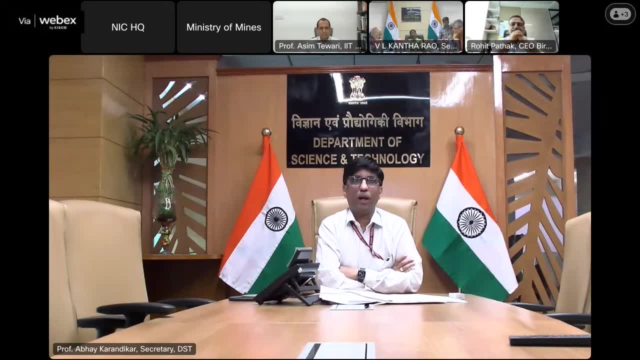 Uh which can be supported uh through this uh prison program, uh our joint focus can be on promoting the startups uh and uh, uh and uh, of course uh we can come up with the areas in which, uh you know uh these supports uh can be done. uh. 1 area which was mentioned by the secretary minds also is the processing of the uh geological data which is available using modern techniques uh such as AI. 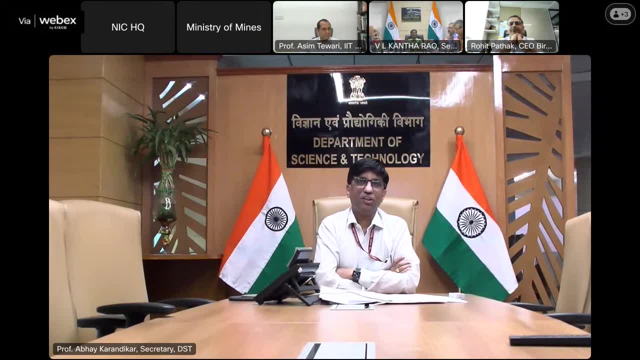 Uh to help in the exploration of minerals, and this can definitely be done uh through the hackathons which can be launched in the incubators which are being supported by in and other universities across the country. We would be happy to work with this program. We can offer our huge amount of sort of an expertise that. 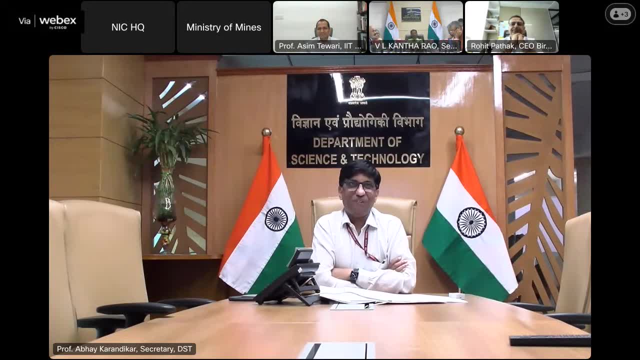 DST has gained by launching similar programs for supporting the startups that, uh, you know, uh, uh, what uh, so that you know the Mistakes, maybe, which were committed by us in the past. uh, you know, as being the initiator of these programs. they need not be uh sort of a repeated here. 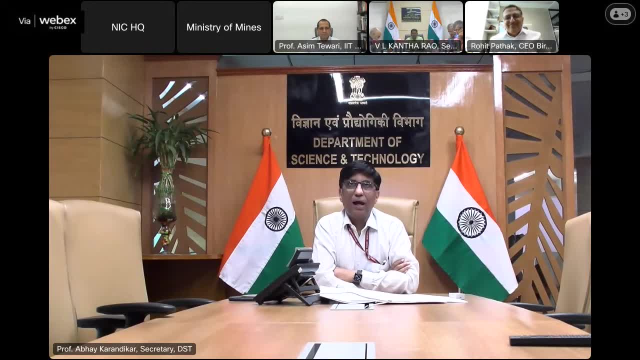 Uh, so we can definitely offer uh those learnings and uh, as I mentioned, we will be happy to work uh with the ministry of mines to see That, how we can spend on and the entire ecosystem of startups in this area. 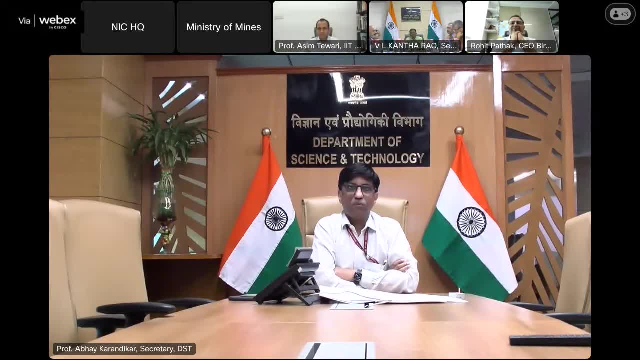 Uh, so once again, I would like to congratulate the entire team of the ministry of mines for initiating this exercise. There is a lot of capacity and talent in our country and I hope we will be able to get a good proposals from. 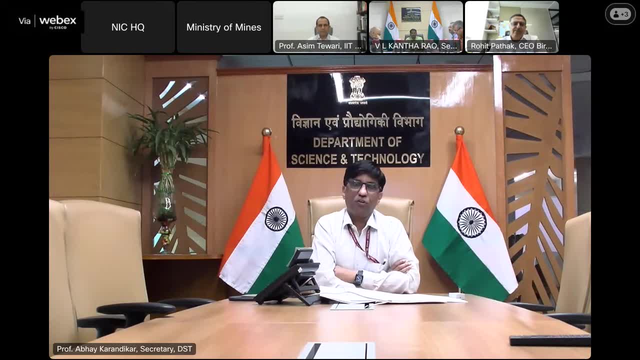 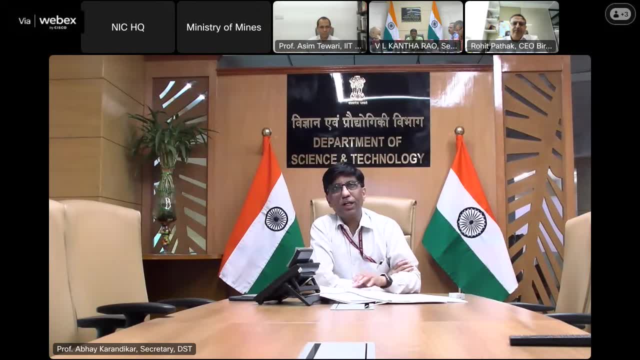 eventually, Uh. so, therefore, I would really urge all the startup participants who are there to uh make use of uh this opportunity which is now being offered uh by uh the government and through ministry of mines, uh to see uh that uh. you know, whatever is the technologies. 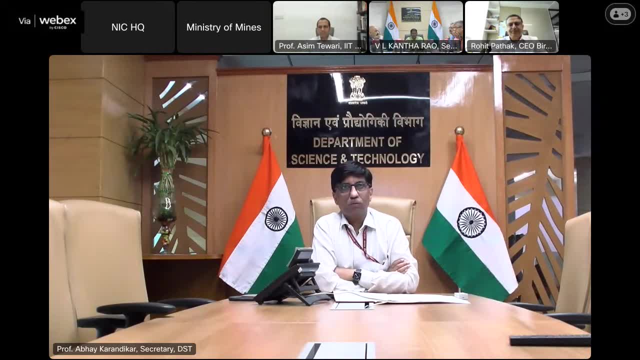 that they are working, uh uh. you know they can leverage this funding, support uh and we can become actually self-sufficient. uh in, uh uh, many of the technologies which either relates to uh mineral exploration, extractions or efficient recycling or developing. 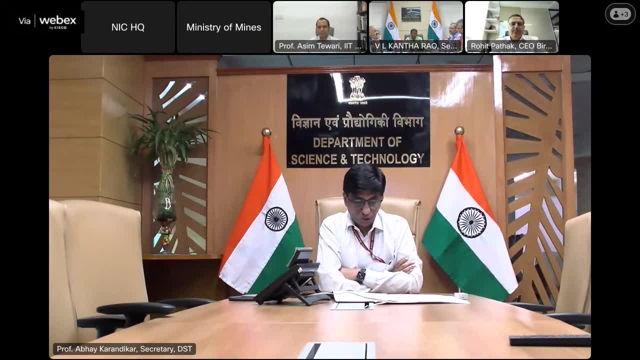 technologies to, uh you know, develop. you know battery storage materials or you know new materials through the computational materials? Uh, you know the, the tools you're using to make sure that, uh, that, uh, you know. 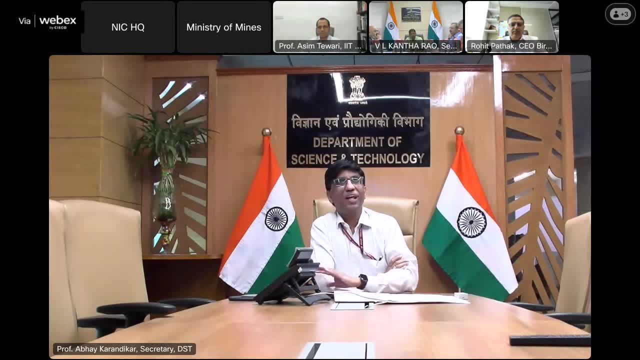 that uh, uh. you know, these are the technologies that will help save lives, uh, and and also help create really best possible uh uh, uh uh. accessible. uhUh uh, uh, uh uh. 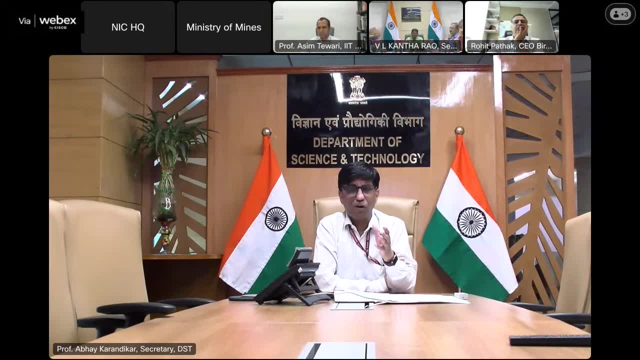 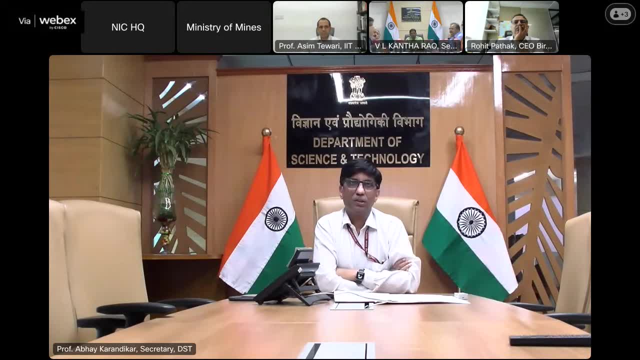 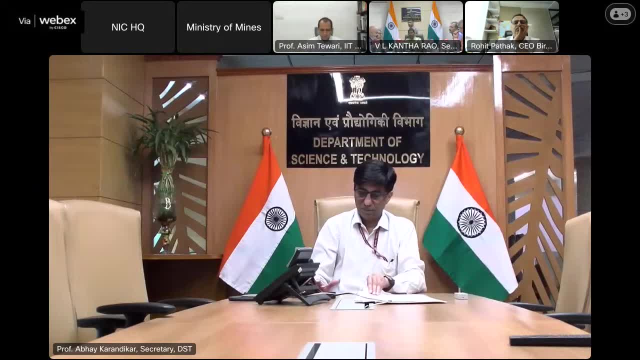 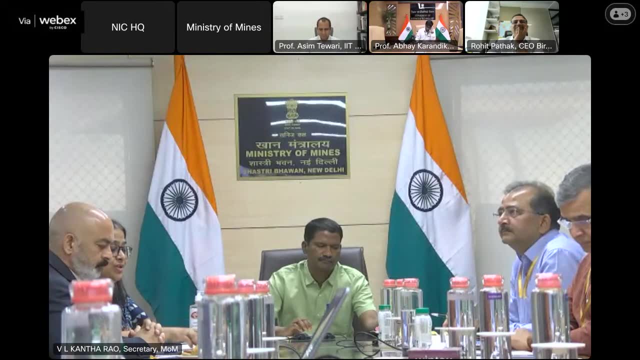 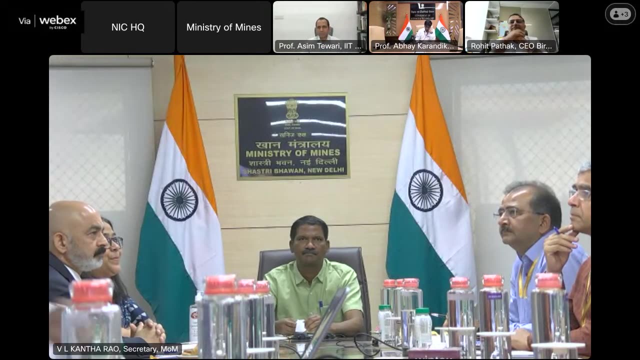 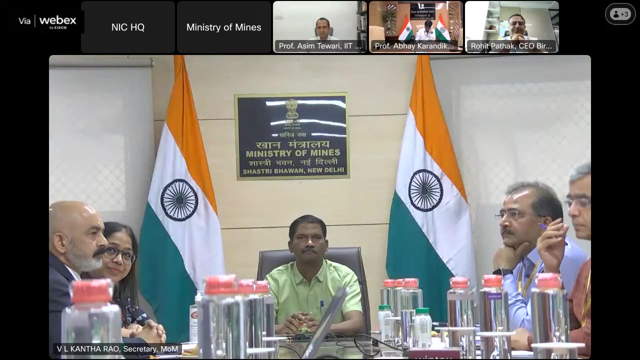 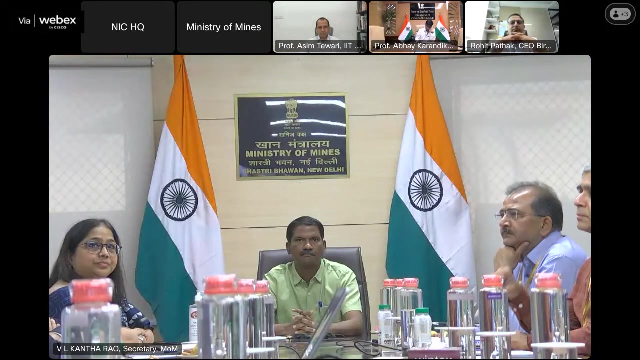 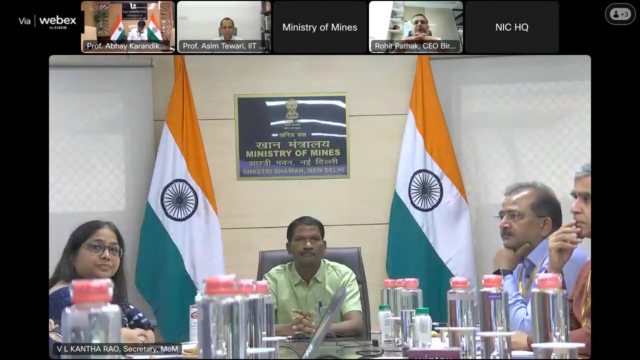 you. Thank you very much, sir, for your encouraging words and your offer to help us in this endeavor. I would request you, sir, that we will be just showing a video clip of three minutes. Please stay connected. Thank you very much. 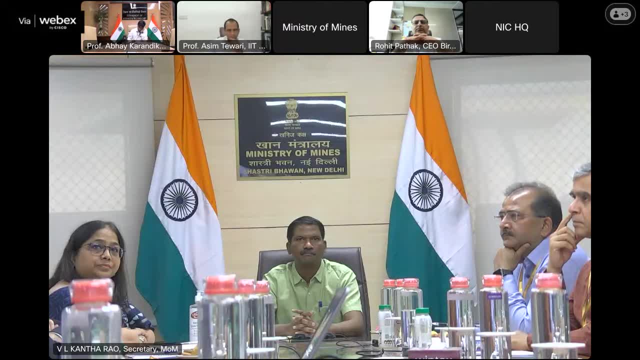 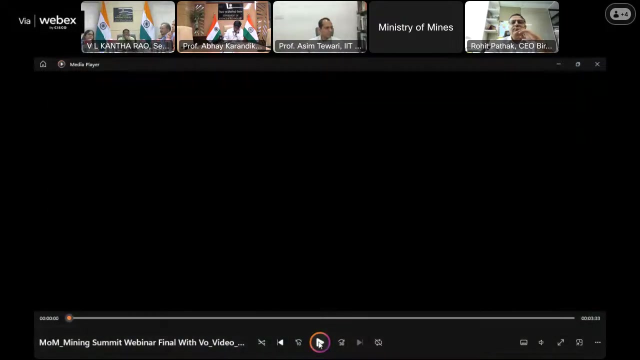 Your friend SIMI評 chit. 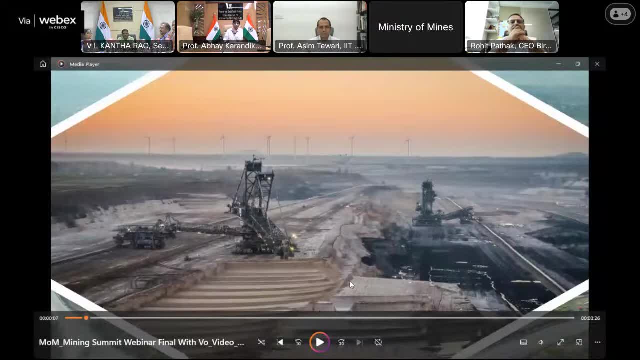 anou fought à la cop 이itor tu và x Constructionstar B Contract & terti orienté, corporation en direction d'impact khare au comportement Crainé et à l'準備 des investiss. translator. qua hold, can you see the video, professor? uh, yeah, yeah, yeah, yeah, i can see audio and video, both are clear. 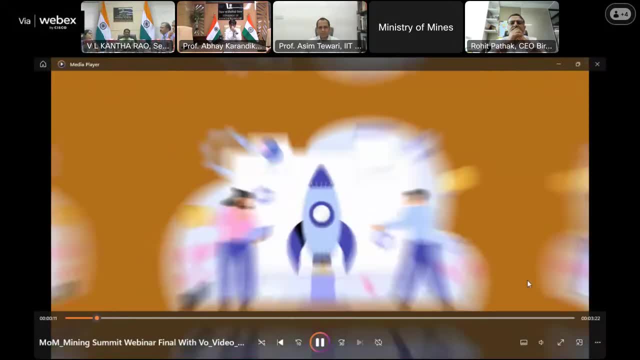 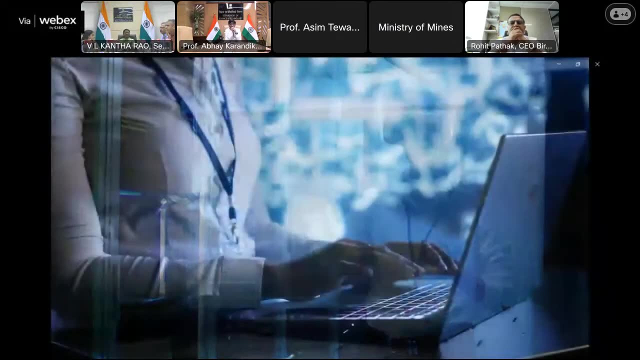 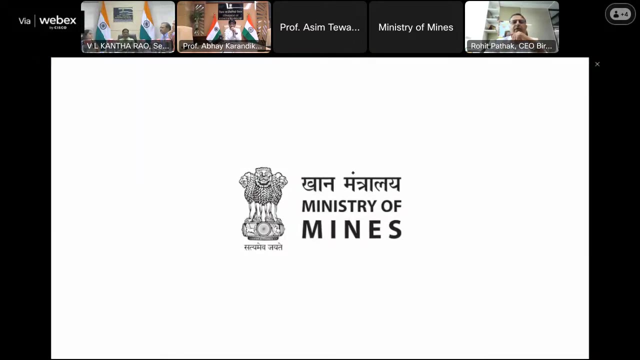 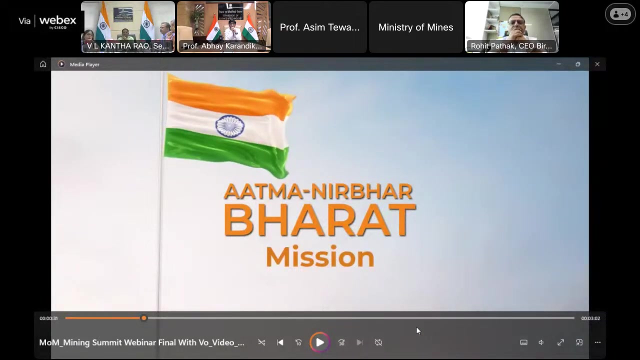 this time the audio is gone. first time you started, the audio was there. now the audio is gone. we'll share it again. it's a small video, we'll just share it again. the first time you played the audio game, so oh, second time i think it didn't come. 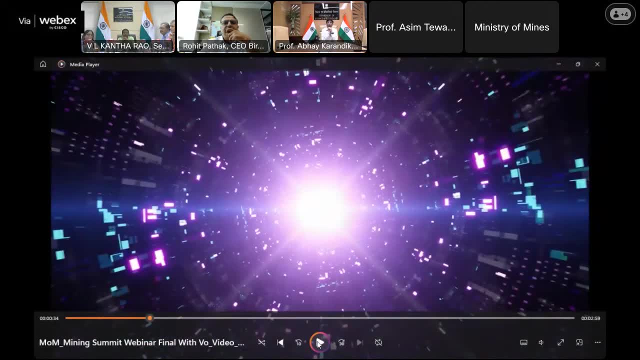 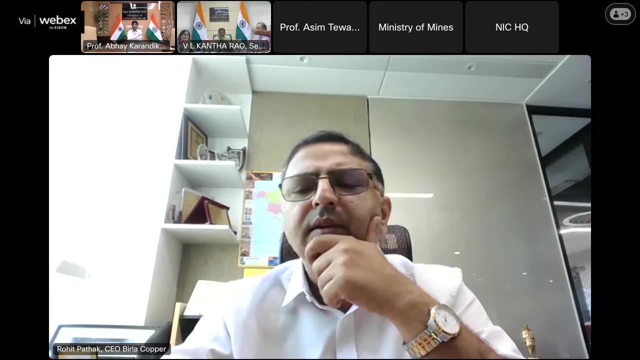 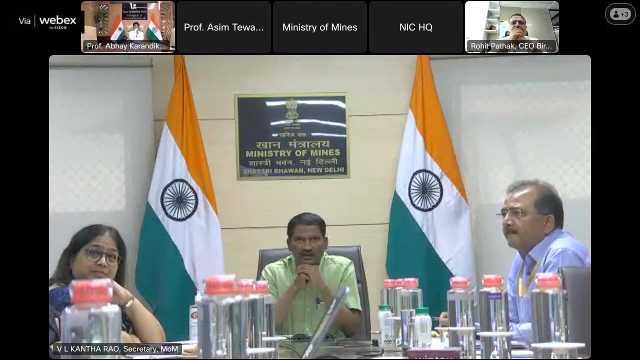 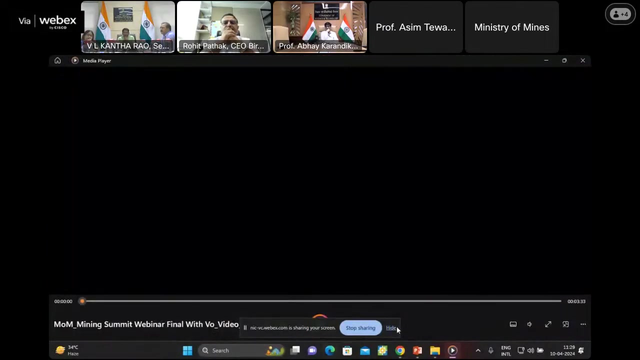 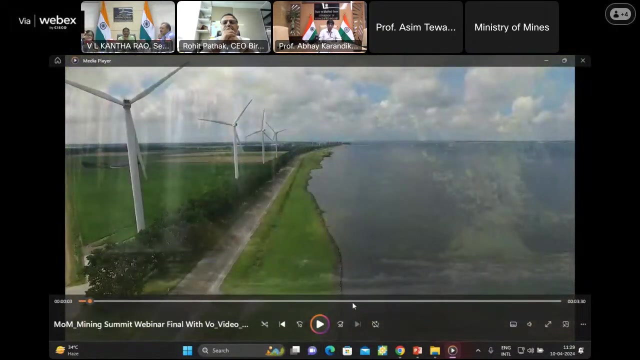 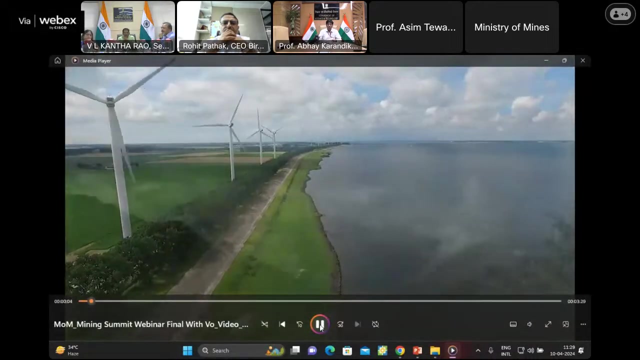 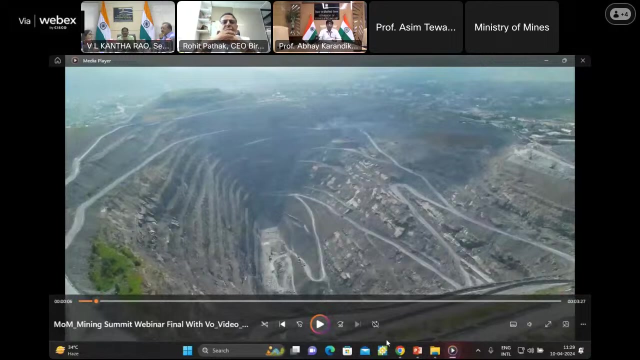 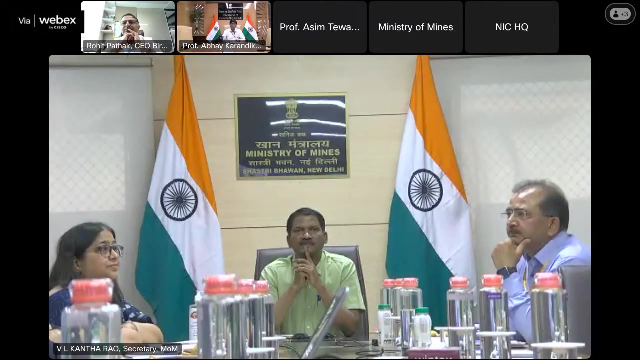 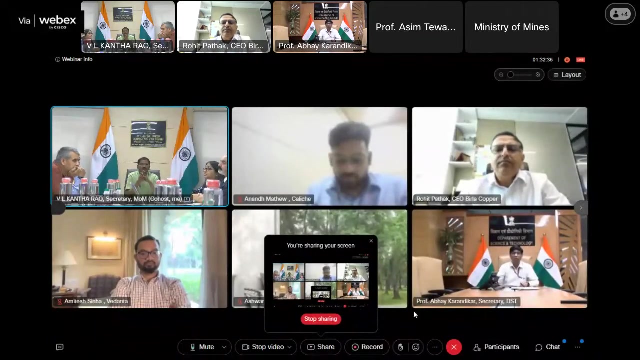 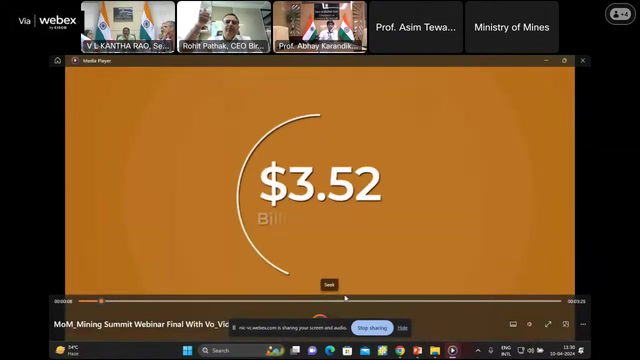 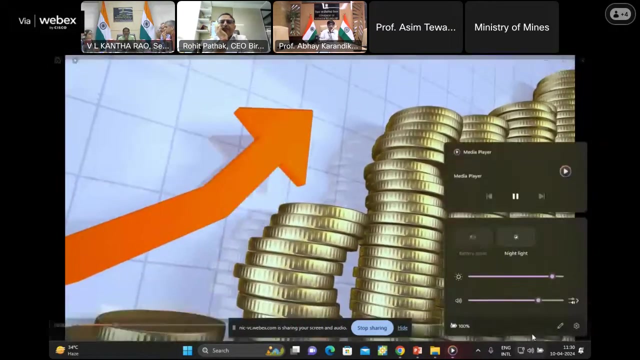 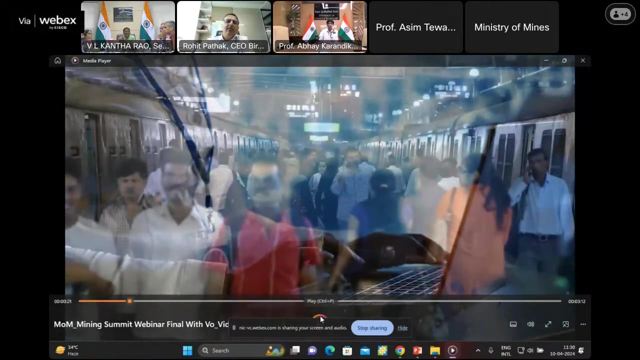 how is it now? is the audio there now? no, no, the audio is not there. is it fine now? is it there now? no, sir, okay, very good, so do you either see the current? huh, this is you're off time, so and this is okay good. growing middle class and a supportive government. and supportive government, Fueled by a record US$8.4 billion funding in 2023,. India's startup ecosystem is experiencing unprecedented growth. This surge is being driven by a young, tech-savvy population, a growing middle class and a supportive 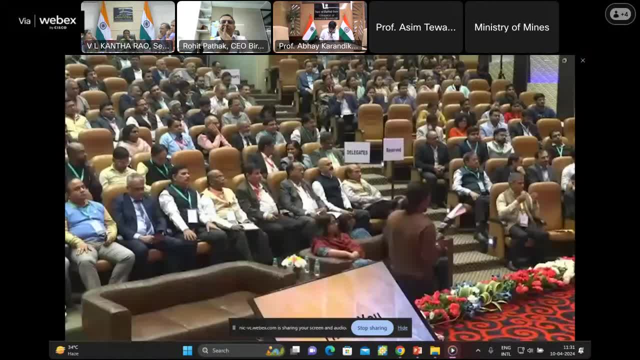 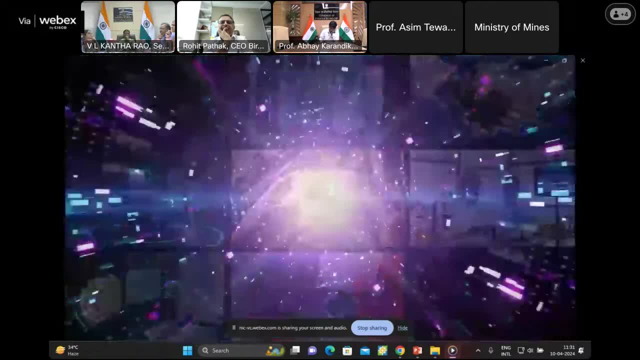 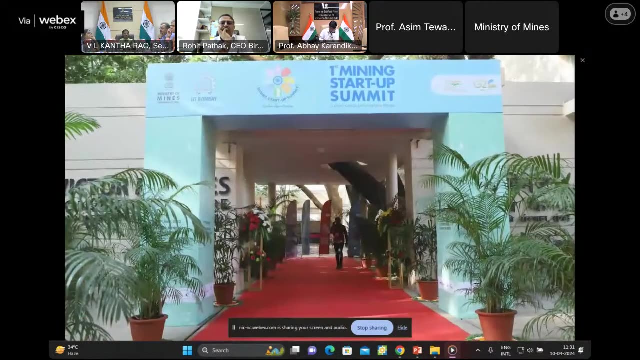 government. The Ministry of Mines is just one example, promoting startups to contribute to the Atmanirbhar Bharat mission of self-reliance. In a bid to energize the mineral and mining sector with fresh ideas, the Ministry of Mines held the inaugural Mining Startup Summit in May 2023, partnering with the prestigious 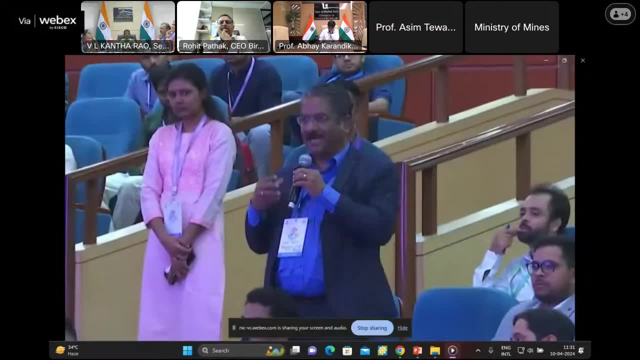 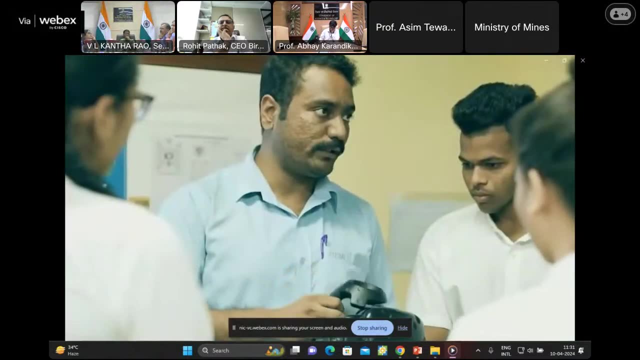 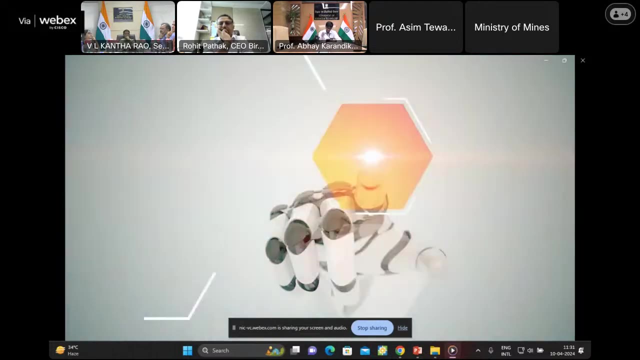 Indian Institute of Technology, Bombay. This successful event highlighted the Ministry's commitment to fostering innovation, Leading them to expand their support to research and innovation initiatives for startups and MSMEs. Further solidifying this commitment, the Ministry released guidelines in November 2023, specifically: 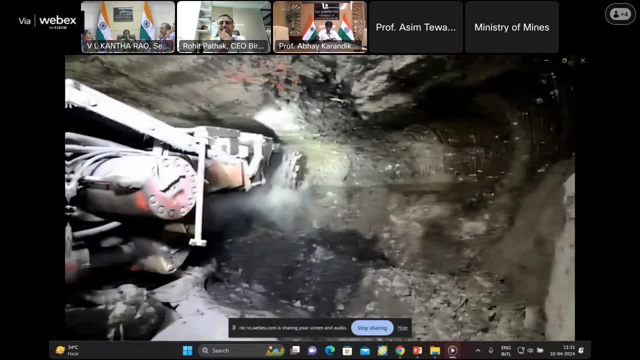 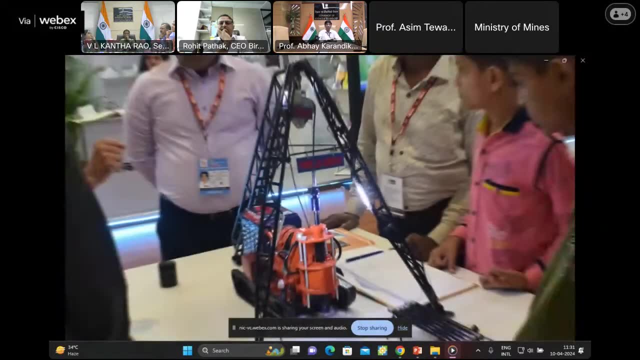 for promotion of research and innovation in startups and MSMEs in mining, mineral processing, metallurgy and recycling sector. To spearhead these S&T prism efforts, the Ministry designated the Devahar Law School, the Indian Institute of Technology Bombay and the Indian Institute of Technology as 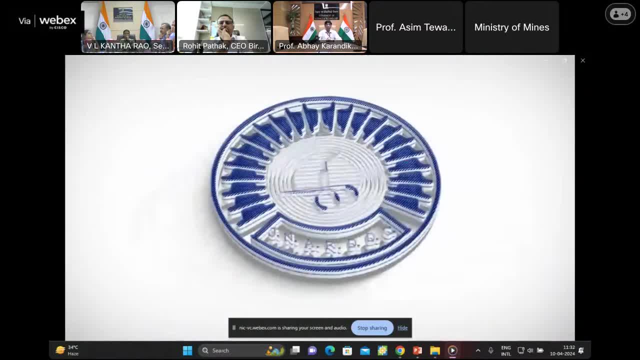 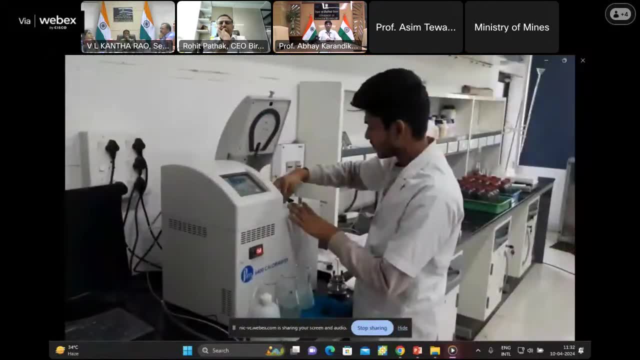 part of the Mining Startup Summit. The Mining Startup Summit will be held at the Nagpur NAL Nehru Aluminum Research Development and Design Center, or JNARDDC, in Nagpur. as the implementing agency, The Ministry of Mines's S&T Prism Initiative offers a unique opportunity for startups. 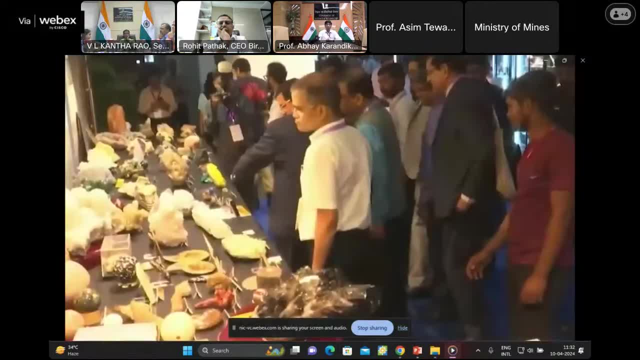 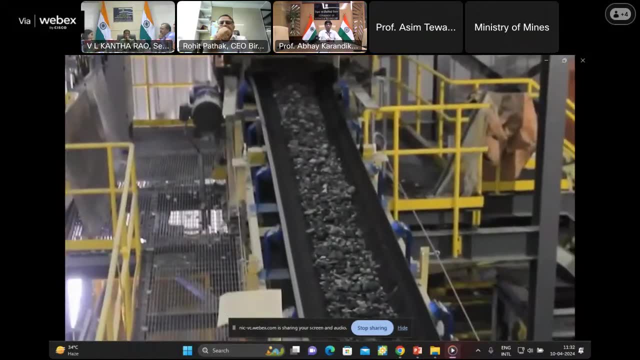 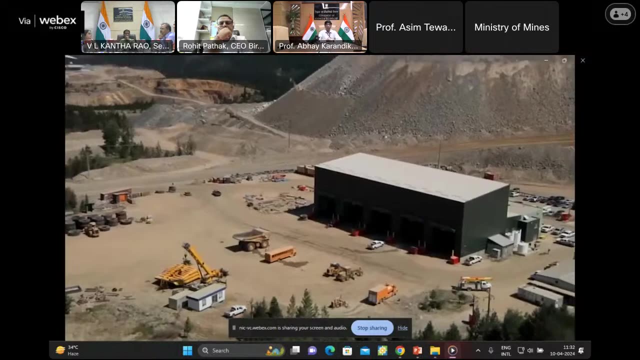 MSMEs and individual innovators. This programme invites proposals for projects up to two years long that focuses on the mineral sector, with a particular emphasis on practical and sustainable solutions for mining and industrial applications. S&T Prism acts as a bridge, providing funding to help. 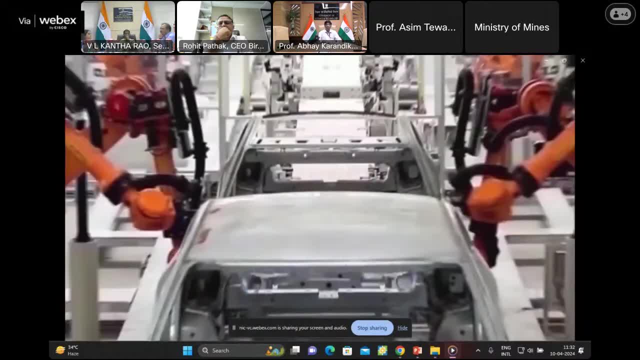 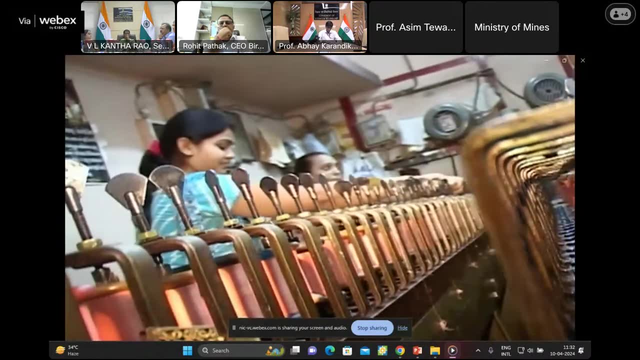 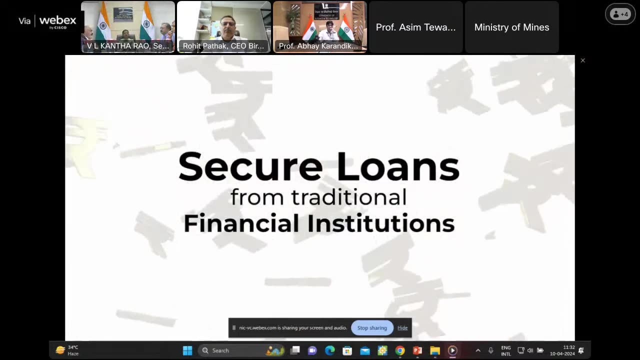 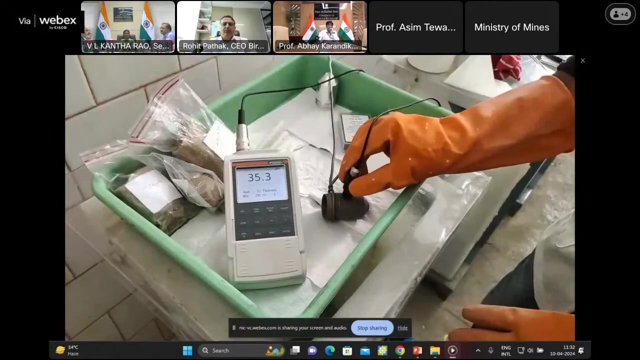 promising idea: transition from development to commercialization. This reduces unnecessary hurdles and empowers these innovators to reach a stage where they can attract investment from angel investors, venture capitalists or secure loans from traditional financial institutions. The Ministry of Mines' S&T Prism program saw strong participation, with 56 startups and MSMEs. submitting proposals. After a rigorous evaluation process, five impressive ventures were chosen based on the significant milestones they achieved during the program. In a ceremony that was held this March 2024,, these five startups received well-deserved financial grants totaling INR 6 crore to further develop their business. 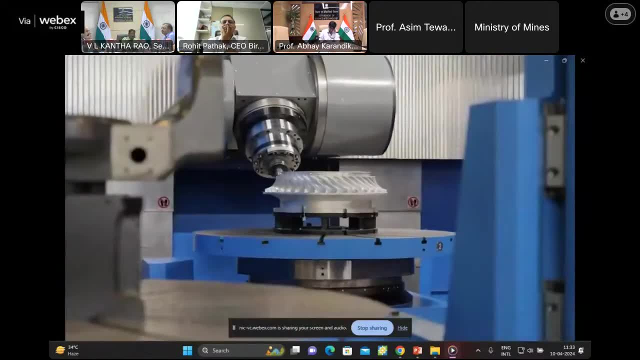 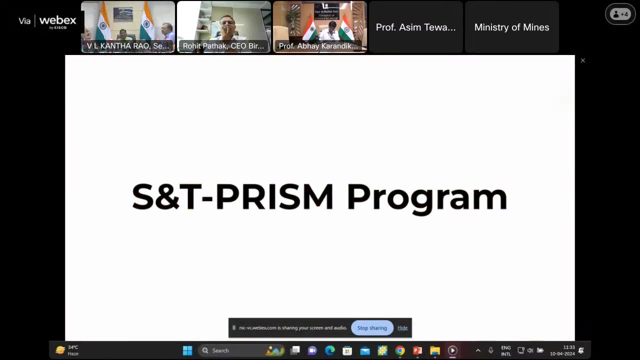 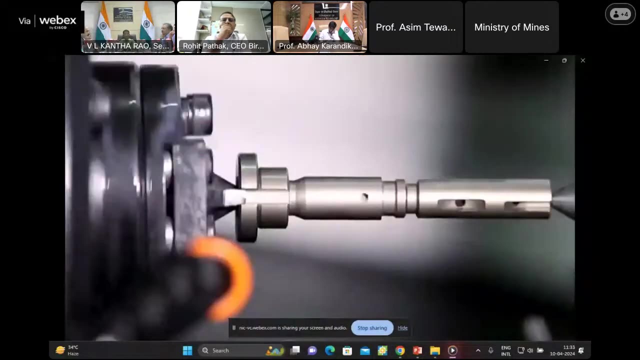 To fuel their innovative journeys. come join hands in Nation-Building with a call for Vixit Bhalan. Don't miss out. Applications are now open for the S&T Prism program run by JNAR-TDC, offering grants to startups, MSMEs and individual innovators in the mining sector. The deadline to submit: 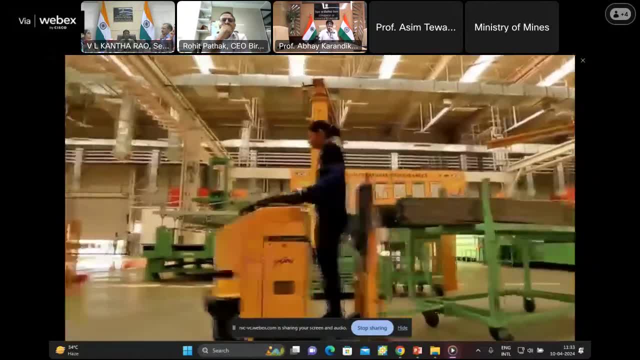 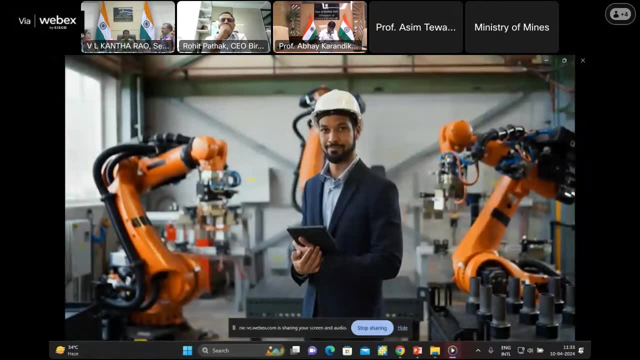 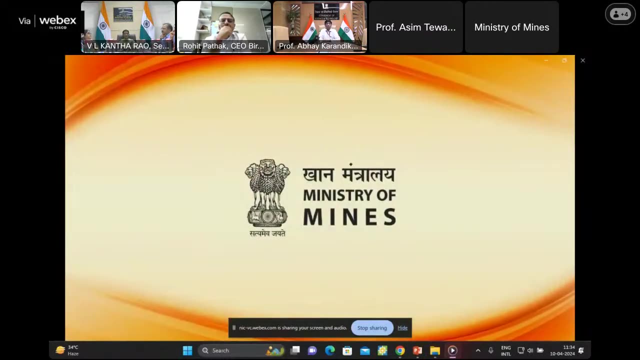 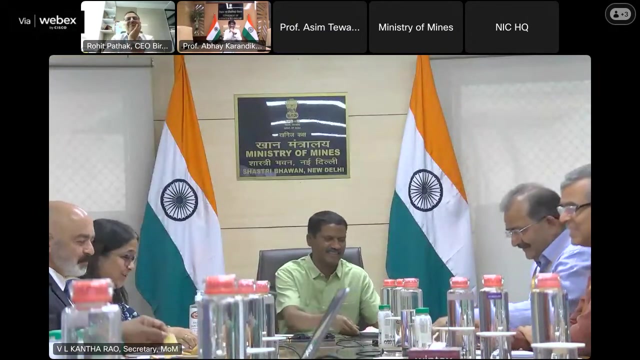 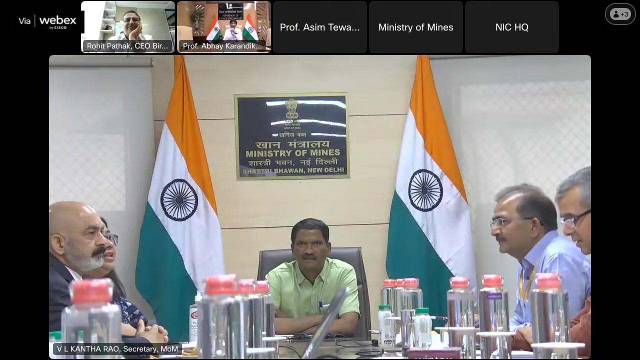 your proposal is fast approaching, so apply by April 30, 2024.. For constant таwns of investment, Data, More for dynamic solutions and Mozhabib. We thank DST Secretary Aditya for taking the time to come here. Thank you, I thank for taking time out to be here for our akhirah session. 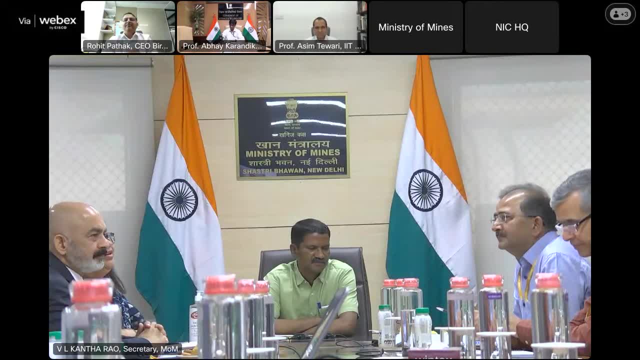 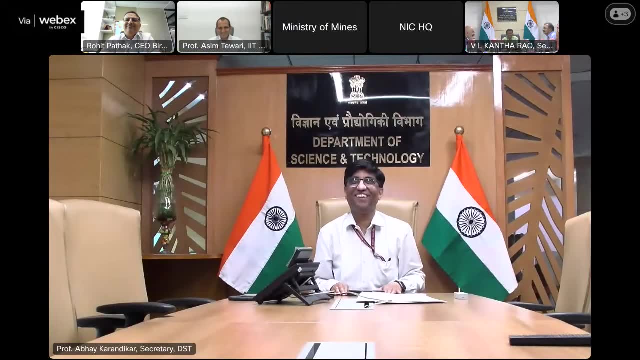 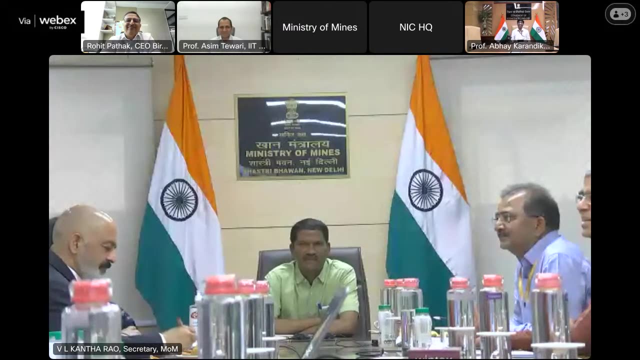 ă uh to be here for our encouragement. thank you very much, sir, thank you, thank you. i need to leave because i have another program going on. yes, sir, we know that you have taken out so much time for us. thank you very much. thank you, professor karandika. thank you, thank you, thank you. 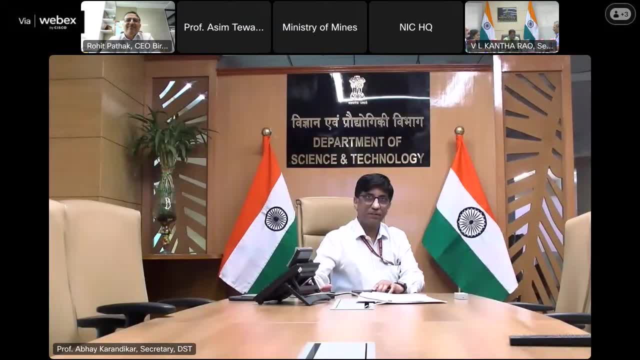 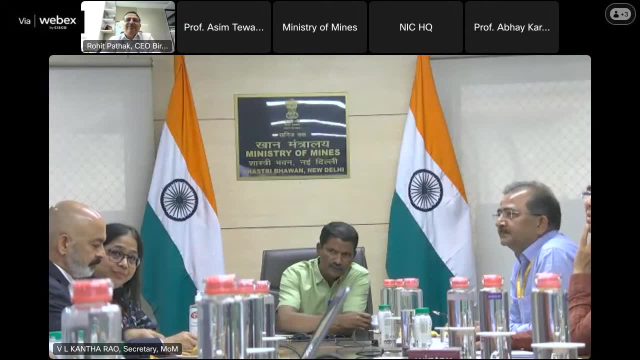 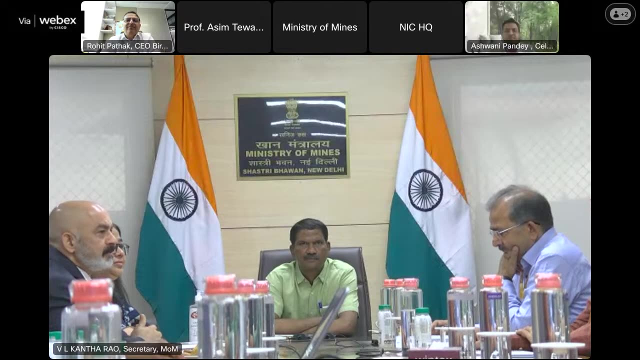 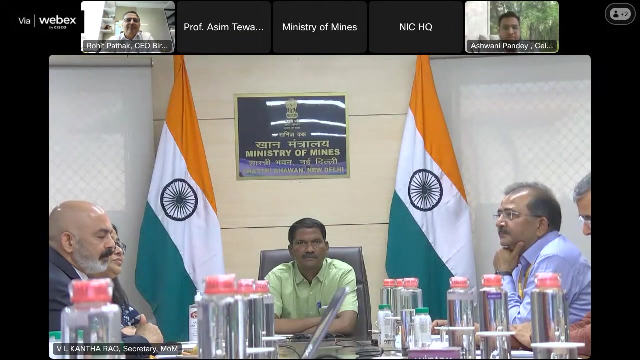 now i request uh dr agnihotri to give a presentation on smg. good morning, uh. let me welcome shri kantarauji, secretary ministry of mines, to this mining webinar, and also the participants on who have joined this webinar. i thank you all for sparing your valuable time and to be part of this program. 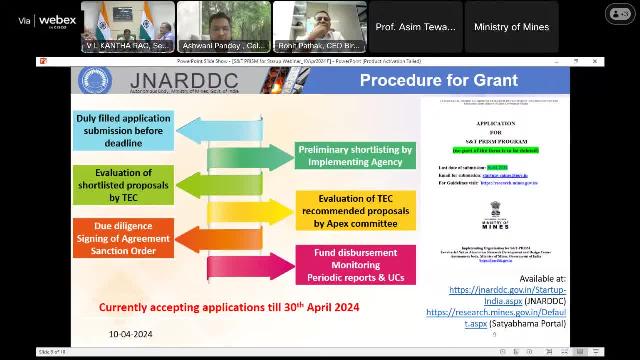 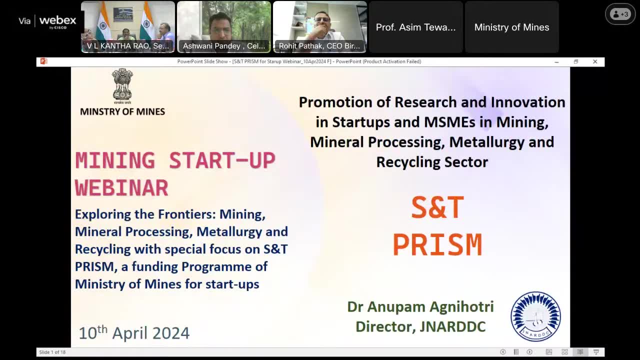 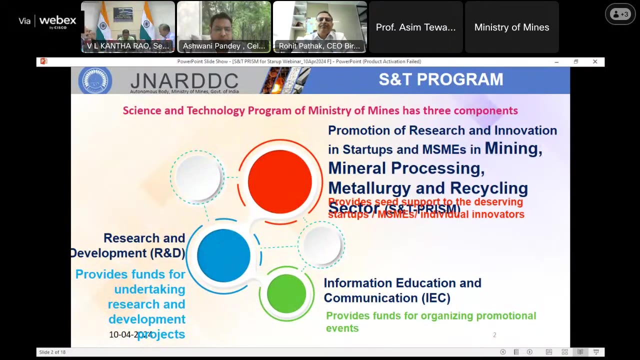 to very first slide. so i'll be just talking in a nutshell about this snt prism scheme, which covers their startups basically in the area of mining, mineral processing, metallurgy and recycling sector next, please. so if you see the science and technology program of ministry of mines, it has got three components. 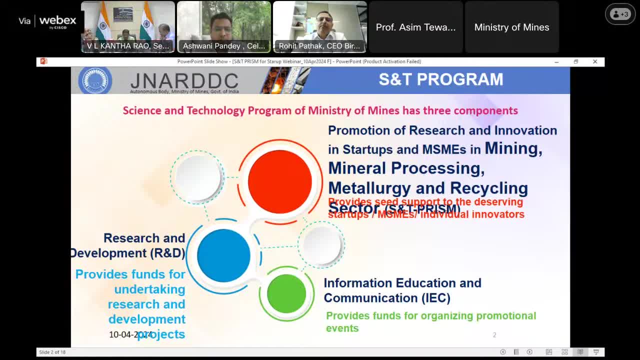 one is research and development, which provides funds for undertaking research and development projects. this rnp program is a program that is being developed by the ministry of mines and the component of snt scheme of ministry mines has two riders. number one is the proposals are to be to develop something above trl level up to trl level 7.. second rider is the proposal. 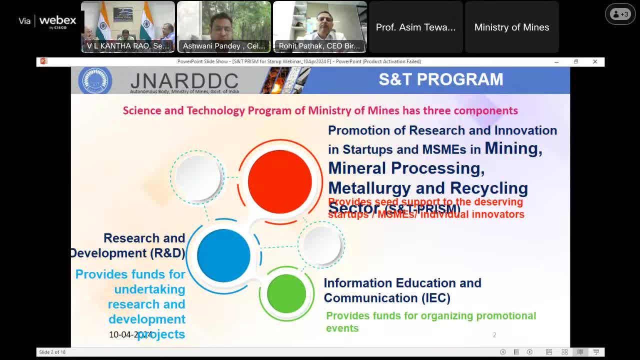 should come along about 20 funding from the industry to authenticate the importance of the proposal submitted. second is, what we are here for today is the promotion of research and innovation: mining in startups and msmes in mining, mineral processing, metallurgy and recycling sector. there is a complete guideline on. 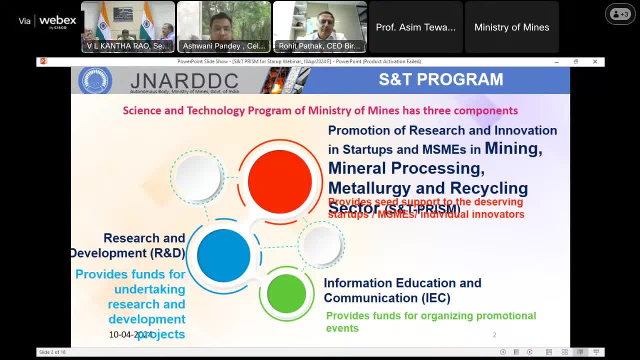 website of ministry of mines for this particular components, the one rider, which i like to share with you here also: at least 25 percent funding should be from own or from the other support for the for the submitted startup proposals. third is information, education and communication. this is: 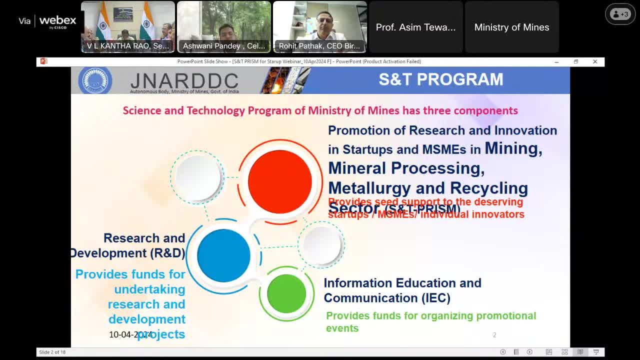 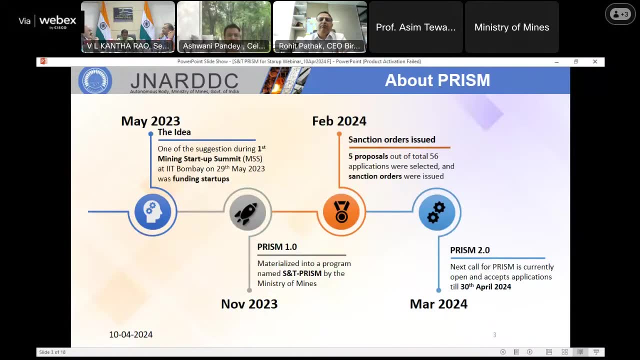 a scheme to promote the promotional events, like conferences, seminars, and this is for national as well as international promotional events. for national, the funding provided is about five. next, please now coming just to how this prism scheme started. it was sometime in may 2023. this parida has already shared. there was a mining startup in mumbai where it, it was felt, 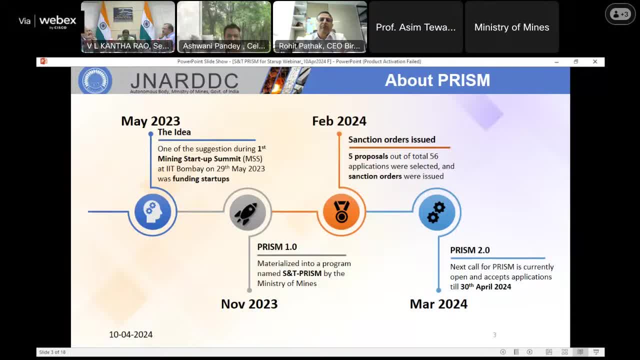 that, although we have got 113 unicons, but most of them are in it or a software industry, it was thought of having a deep tech sort of a startups and there was a requirement to push this and this is where it started and we had this scheme launched somewhere sometime, on 15th november that is. 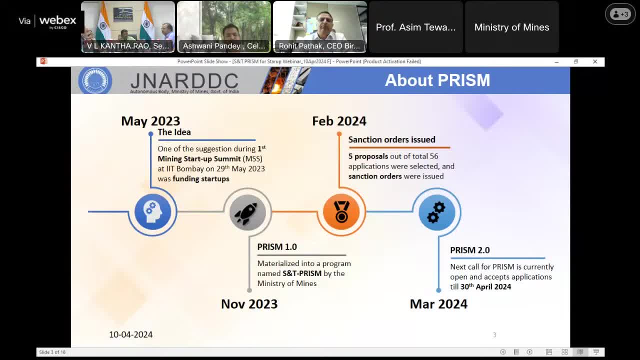 known as we call it, prison 1.0. so let me share with you the prism. all this scheme got gati and shakti only after shri uh, our, our secretary c kantaraji, joined ministry of minds. i mean, took the charge of ministry of minds. and let me also share with you that my engagement with ministry 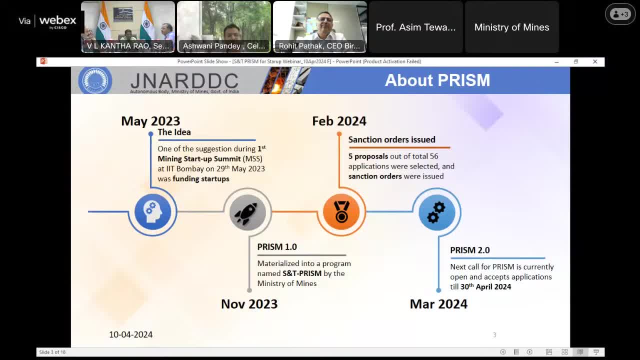 of minds. for last more than 30 years, i have never seen a secretary who is so inclined towards the research and development, science and technology. it's because of you, only this, this and february 24 c- i i added gati for that. can you believe that? 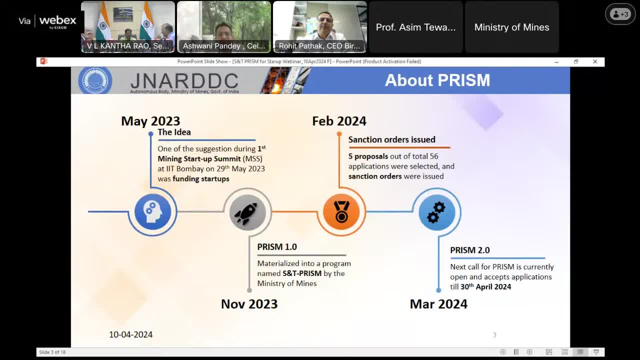 two and a half months, the scheme was launched and the sanction letter were awarded to the through these five startups, out of which four were in deep tech and one was related to the software for for developing the re program. so this is how it started. now the the sanction letter were given. 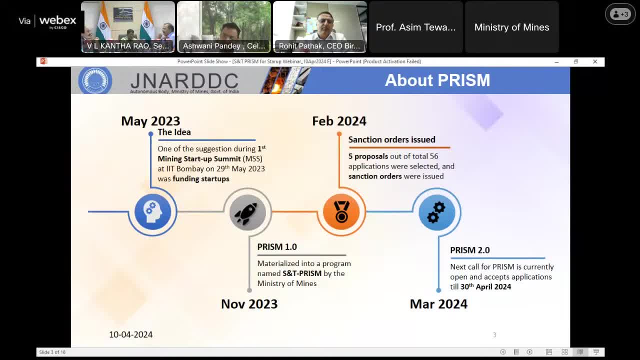 on 29 february and the second, prism 2.0, was launched on 1st march 2024. so that's the gutty this program is having, and this is there for till 30th of april. so i request all of you to be a. 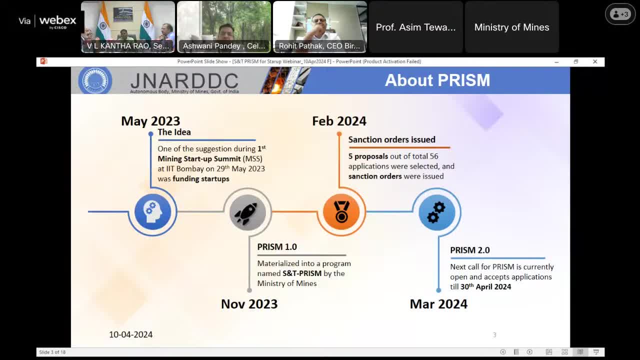 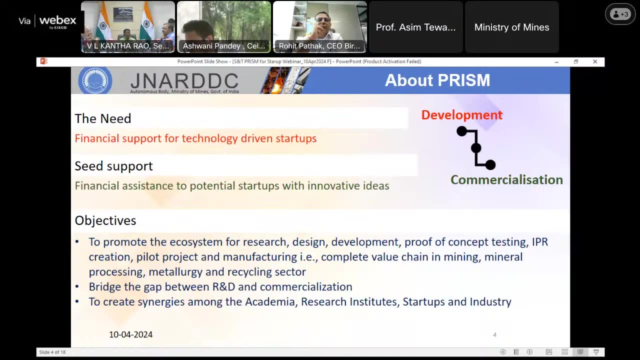 ambassador for this particular program and promote this event. so we have good amount of budget this year for the startup program, so please, uh, promote this event and convey the message. next, please list just about the first prism is a scheme from development scale stage to the commercialization, the need i mean. if you see the industrial revolution 4.0. 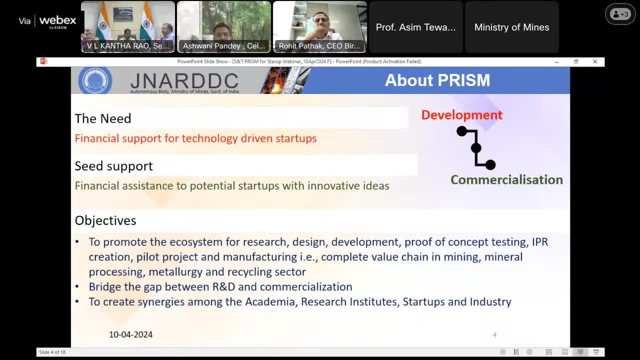 it is more of a talent base when, when there comes to a talent, there is always a shortage of the funding. so it was thought there has to be a financial support for the talent- talent in the area of mining and metallurgy. so financial assistance for potential startups with 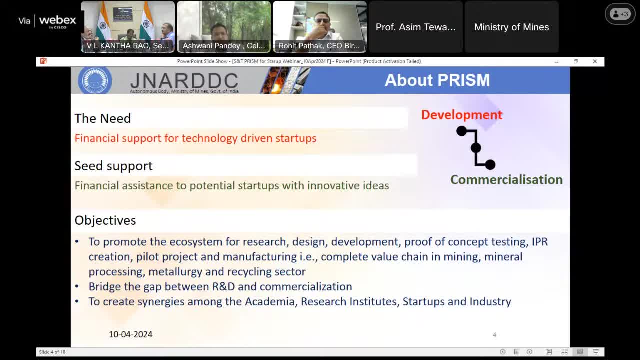 of course it has to be a kind of a out-of-box thinking: innovative ideas to promote the ecosystem for a complete value chain in mining and metallurgy. objective is also to bridge the gap between r? d and commercialization, because it is felt that r? d is happening in silos and commercial people. 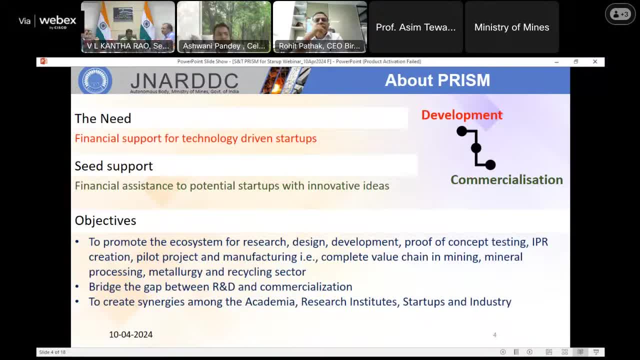 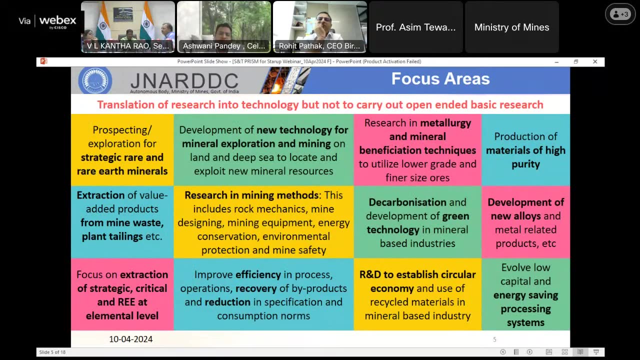 already working on that. so have a connectivity between them. this program is there and, of course, to create a synergy among the academy, research, startups, industry and the incubation centers existing in the country. next, please. so these are the focus areas, like translation of research into technology, but not to carry out open-ended basic research. so here the rider, one more rider which 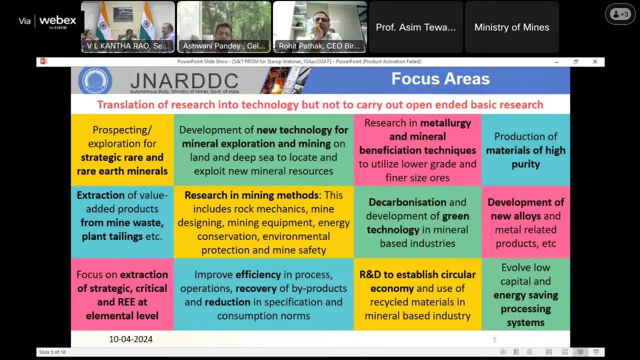 i can recall for the startup is you have to start from trl level 3.. at least you should have a proof of concept for the process, product or a service from where this pro, this startup, can be financially supported. so what ministry of mines is looking for? prospecting, exploration of strategic rare earth elements, as you know that? 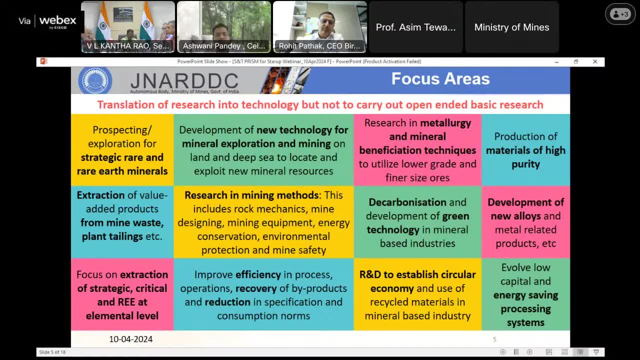 success of a climate change program is going to depend on the, on the renewable energy, is going to depend on the evs, and these critical minerals are going to play a very important role in that. so this is this time. the focus is critical minerals for the startup scheme, then development. 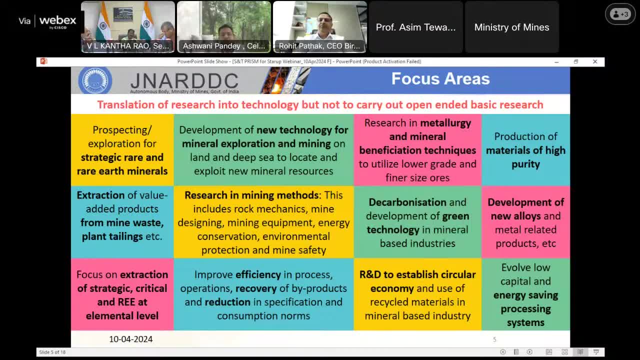 of new technology for mining and exploration. mining, it has to be different from the existing ones. research in metallurgy and mineral beneficiation: as rightly professor karandikar said, we are fifth largest, but getting it out in the elemental form is is is a big task, then. production of materials of high purity. this 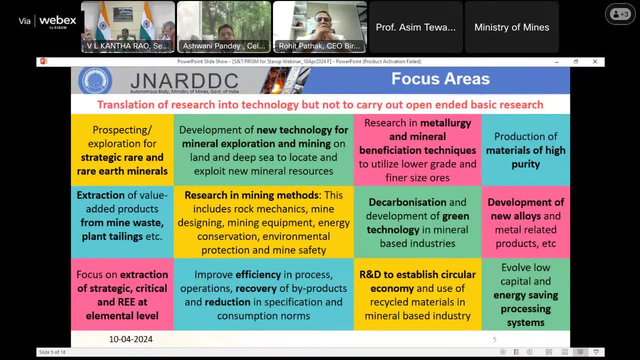 is what we are. the country is importing presently. so if we have to become at mirabar, this has to be pushed. extraction of value-added products from mine waste: a circular economy concept has to be applied and more and more startups will be supported in this area. research in mining methods: 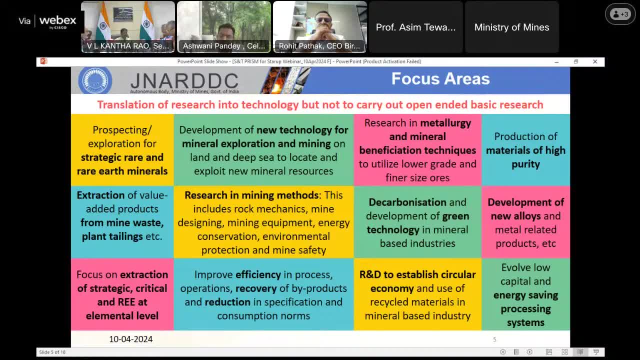 development of the mining equipment. also, decarbonization and development of green technology for success program. climate change, success program for india to become a carbon neutral by 2070. this is an important focus area. development of new alloys and metal related products: here what we have to see, we have to see a replacement of the import materials, whether it's 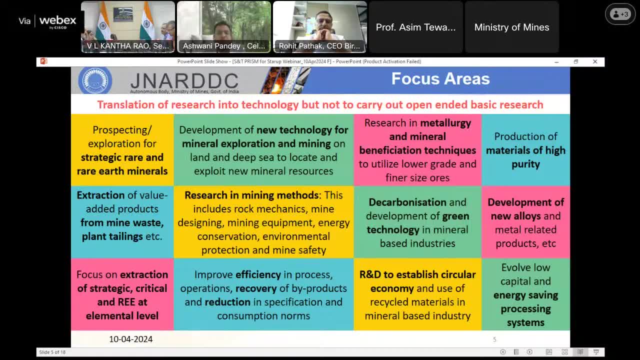 alloy or the metals. focus on extraction of strategic and critical in the elemental level, worrying about the application. once you have an elemental level, the, the strategic minerals it will find the application by itself, of course, improve the efficiency and the recovery and reduction of the existing processes. rnd: to establish circular economy and use of recycled 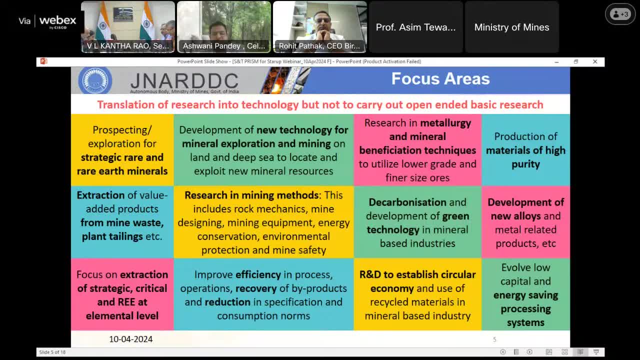 material- this is going to be the success story for a developed india by 2047- and, of course, evolve low and capital energy saving processing system. the less energy, better the climate is. this is the concept, what we are promoting. next, please now talking about the budget and financial support. up to two crores is the financial 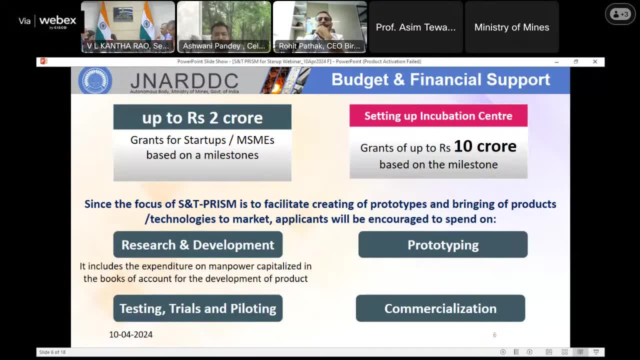 support for the grants of startups and msme based. it will depend on the milestone. actually, if it's a startup, the limit was 50 lakhs but if it would exceptionally good and meets the criteria of ministry of mines for the startups, it can go up to two crores. then setting 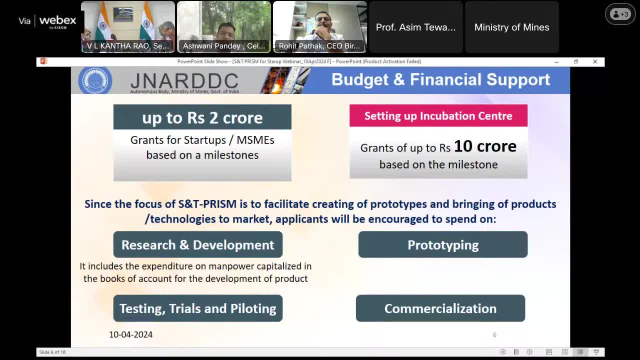 up an incubation center. the grant of 10 crore will be provided ministry of wines and we are working on developing the guidelines for the same now, since a centiprism is to facilitate the creating prototypes for this. we have got four different sections which will be encouraged for. 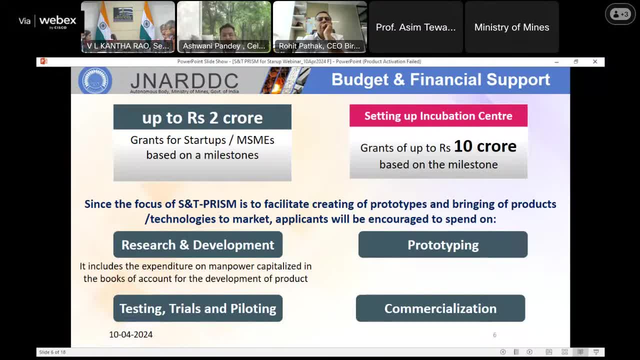 this financial support. one is research and development, other is prototyping, testing trials and piloting constellation. here i'll like to share with you that we presume that a lot of research and development has already gone in up to tier level three, so there should not be much demand. 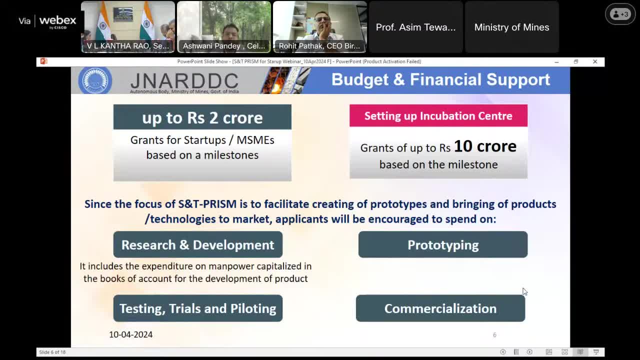 when it comes to research and development, it should be more focusing on prototype testing, trials and piloting and commercialization. so that is a kind of a catch in your proposals to be submitted in the startups. uh, yes, some part of the financial support can go to r&d, but not the major one. 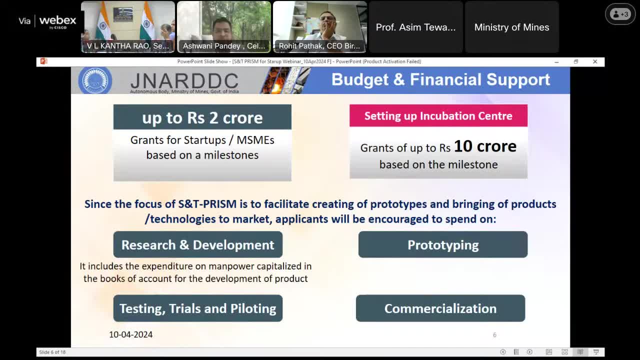 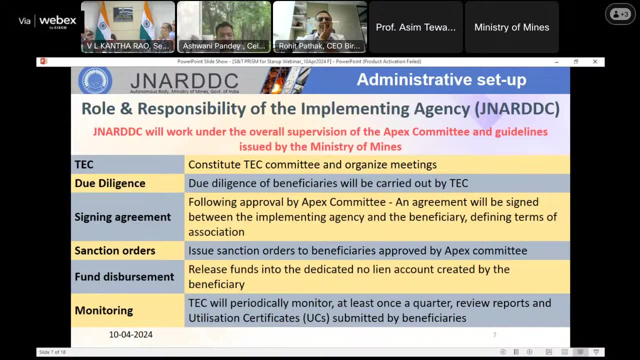 if, if you require a major r&d support, you can go to the r&d, research and development component of the science and technology scheme of ministry of minds next. please then the administrative setup, role and responsibilities as indicated in the video, was given to jna rdc, that's jawaharlal nairu alumni research, development and design center. 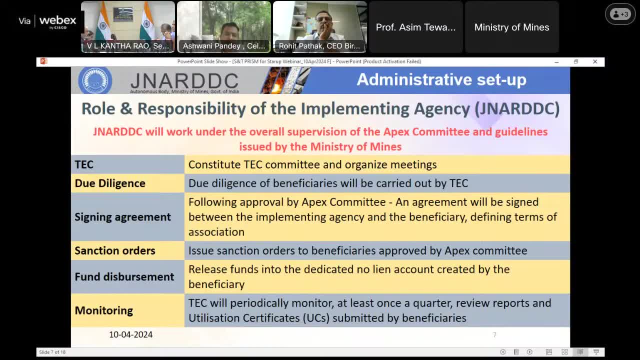 the responsibilities of implementing agencies is to constitute a tec committee which keeps which keeps co-opting the member as per the requirement, as per the proposal submitted, and organize the meeting. due diligence of the beneficiaries will be carried out. this will be in terms of- i mean in terms of the legal, financial and commercial due diligence has to be there. signing of agreement. 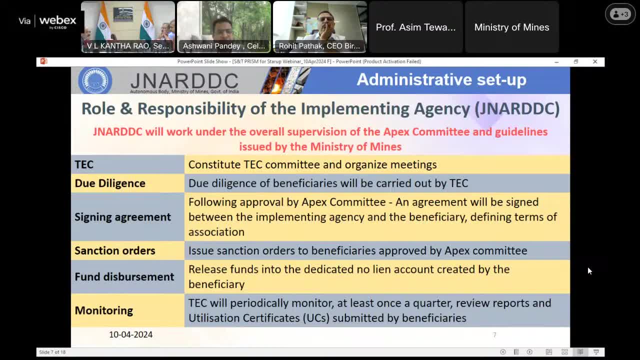 following approval by apex committee, which our secretary is a chairman for, that agreement will be signed between implementing agencies and the trees. sanction orders will be issued to benefits approved by apex committee and, of course, after the due diligence and the final disbursement will be there and there will be a monitoring on regular basis. it may be quarter, it may be monthly. 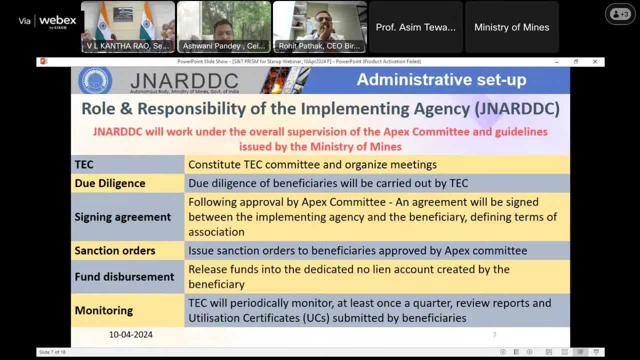 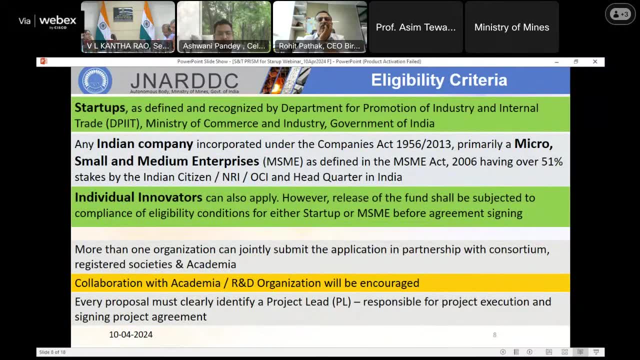 depending depending on the progress made by the startups and the utilization certificates submitted by them. next, please, eligibility criteria. i think there are three categories in which the application can be submitted. one is startup as defined by dp it. it has to have a turnover less than 100 crores or it can. 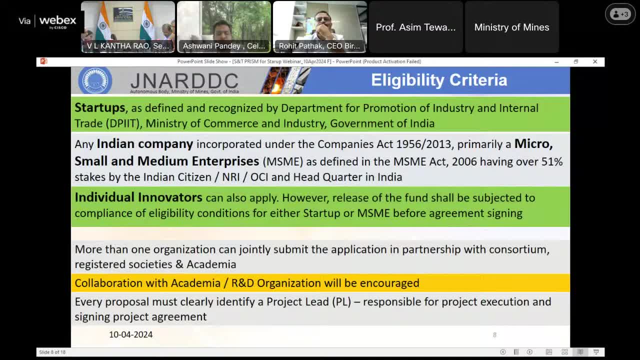 be a msme. a micro has to be a turnover less than five crores, a small enterprise has to be a turnover less than 50 crores, and the medium one has to attain念over, less than 50 croresips if you are a lucrative вс ng. and a combination of the dan Louoka and a combination of the dumping in character for this internship to be implemented on a monthly basis. has change of the implementation of 57 evaluation, its change in terms of charge for the neden of change, that is, with within it. 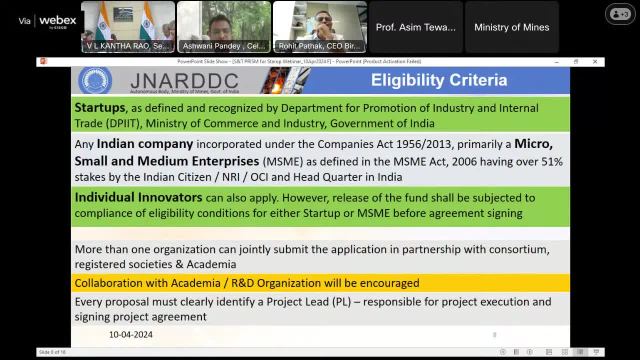 over less than 250 crores, as defined in the msme act 2006. and the third category is the individual innovators, who can apply directly, but they have to have a compliance of eligibility conditions, either matching with a startup or msbs, before agreement is signed. and yes, more than one. 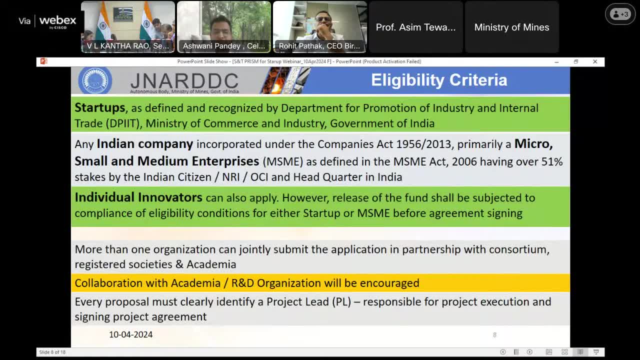 organization can jointly submit the application in partnership with consortium registered societies, academia, so that flexibility is also there. so collaboration with academy and r? d programs will be encouraged. every proposal must clearly identify a project lead who will be the nodal for communication, responsible to for the project execution and signing the other project agreement. 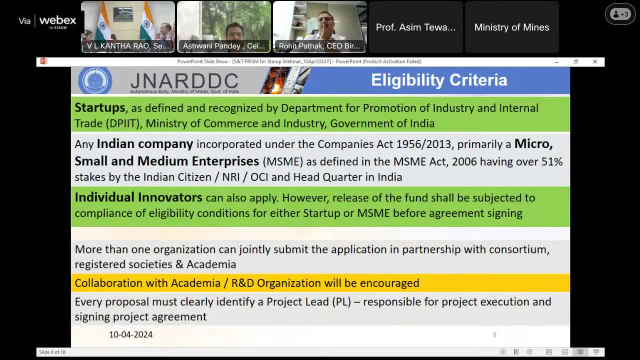 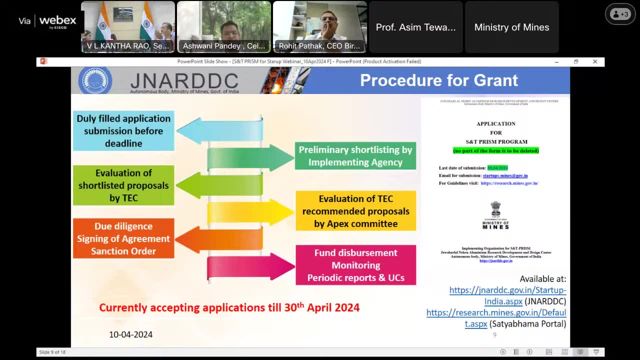 so this is the eligibility criteria for this, and we also prefer that this startup should be attached to one or other incubation center which are already existing in the country. next, please, procedure for grant is like duly filed application submission before the deadline. this time, the deadline is 30th april 2024, and then there will be a preliminary. 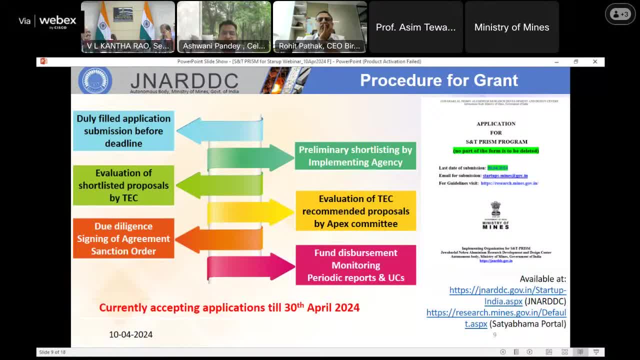 shortlisting by implementing agencies depending on the criteria or the guidelines given by ministry of mines. uh, depending on that will be. i mean there will be two levels: scrutiny at tc level. second will be evaluation of shortlisted proposals by tc, where a physical presentation will be made by the shortlisted startups. then there will be a evaluation of tc recommended. 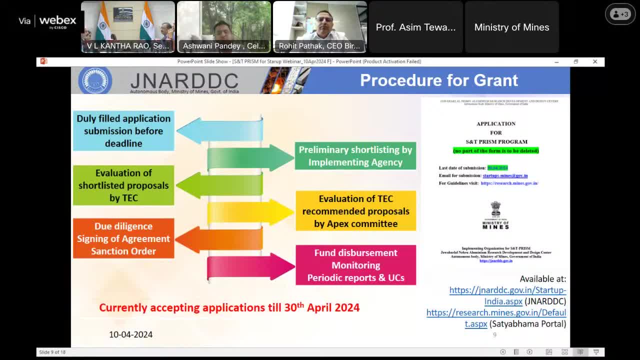 proposals will be assessed by apex committee. after that the approved proposals, there has to be a due diligence sign, then signing of agreement and a sanction order. then there will be fund disbursement depending on the milestones. there will be regular monitoring of the startups and periodic reports and uc are expected from the spark. startups currently accepting obligations is still 20th. 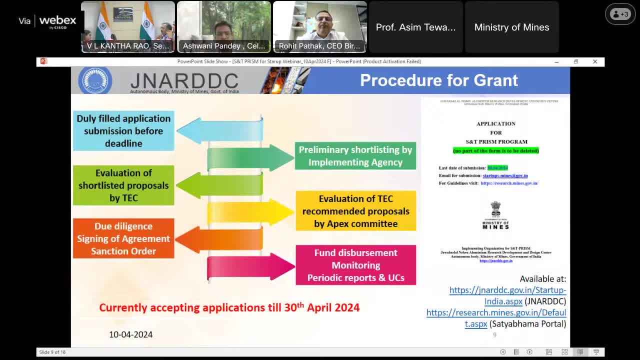 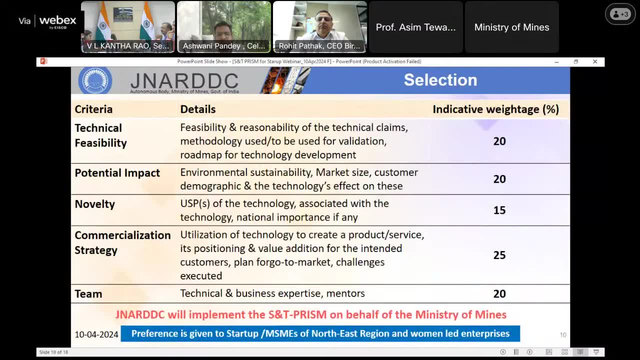 april 2024 and you can see the two links provided here where you can download the applications. next, please, selection criteria. there are five criteria which has been put in the guidelines. one is technical feasibility, potential impact, novelty, commercialization strategy and, of course, how strong the team is. technical feasibility: yes, the idea has to be novel and idea has to be at trl. 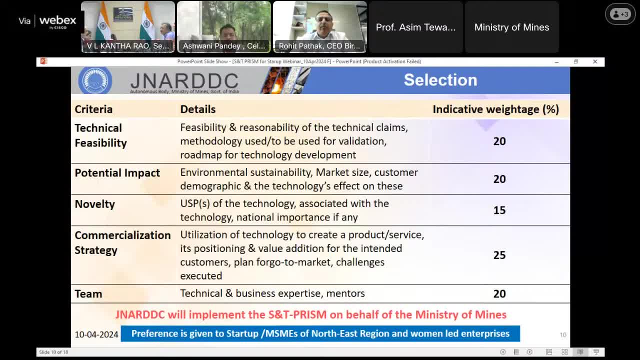 level three and above. that is, having a proof of concept, whether it's a process, a product or a service, then potential impact, environmentally sustainable. it should be like if you talk about the waste utilization: by using the waste you should not create another waste- so that concept has to be there. the market size, who are the customer, demographics- this all has to be well. 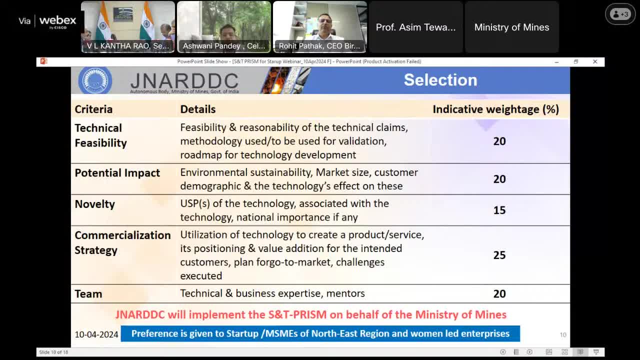 listed in your proposal, novelty, usp of the technology, how it is different from the existing one or it is at all a new one. then commercialization strategy is how we are going to promote the product process of the service in the coming years, after the two years are over, and, of course, the kind of 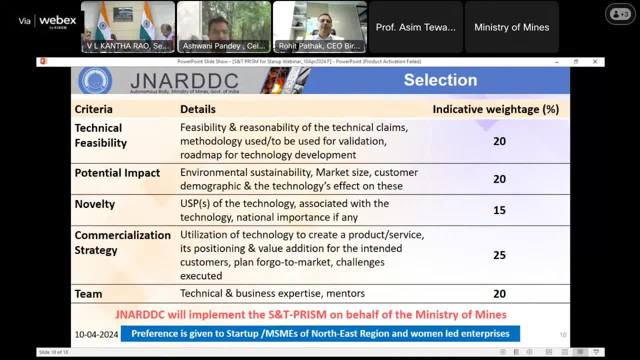 experience and expertise the team have when it comes to technical and big business expertise. who, who will be the mentors for this then, actually will implement the snt prism on behalf of ministry of mines? and here the good thing is like: the preference will be given to the startups from. 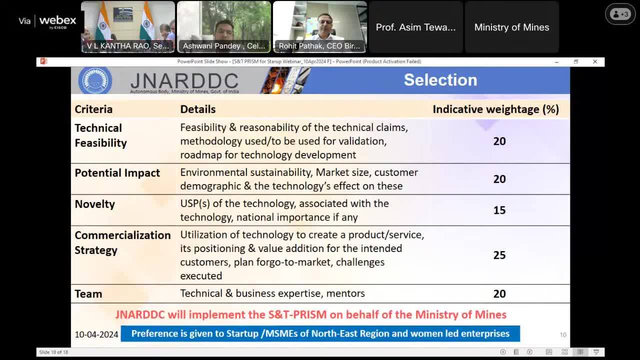 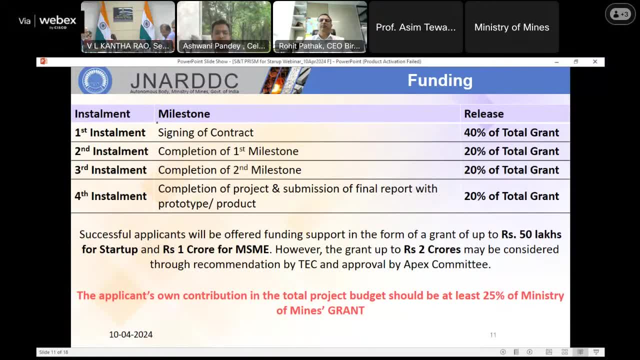 the northeast region and, of course, women led enterprises. next, please, funding of the startups. as i showed in the previous slides, two crore is the maximum funding and first installment will be after signing the contract and, of course, the due diligence, the 40 of the grant will be released. uh, second and third installment, it all depends on the milestone. if 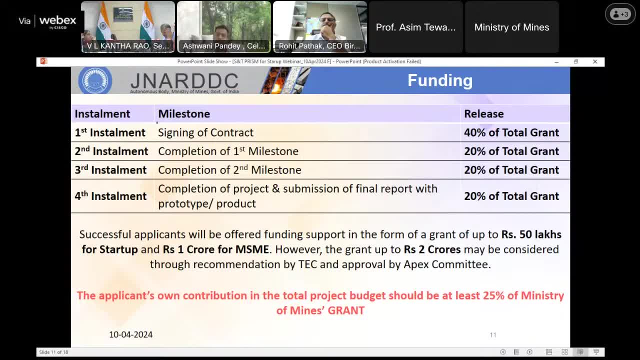 there are more number of milestone, then this 40 will be divided among those milestones for the budget distribution and the last installment will be divided among the budget distribution and the last will be twenty percent of the grant will be provided on completion of project, submission of final report with the prototype product given to us, as i told you, the grant. 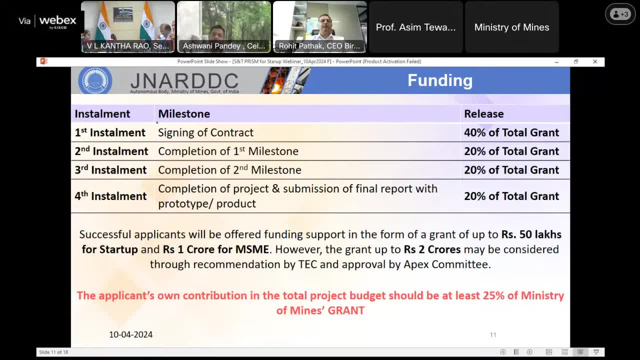 is up to 50 lakhs per startup. but if a proximity feels no, it is something of uh interest to the country, uh it can go up to two course. the applicant's own contribution to the project budget should be at least twenty five percent. it can be in any form as listed in the guidelines. 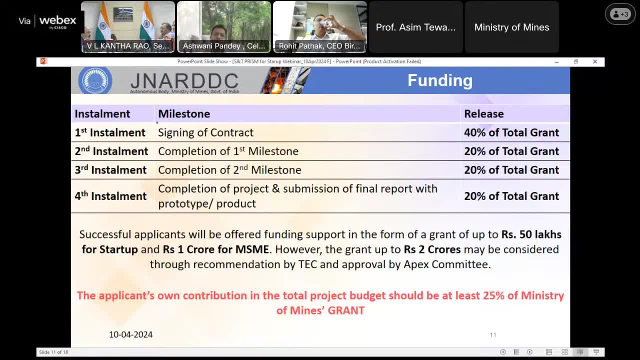 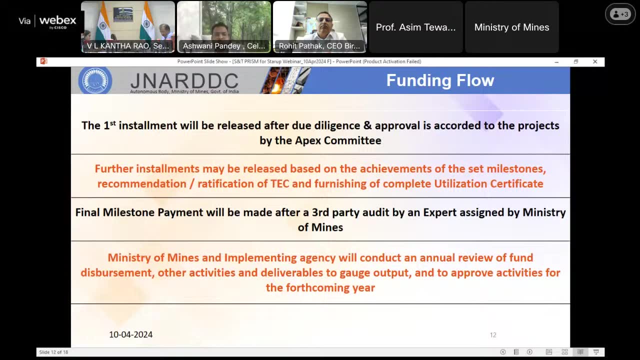 of ministry of miles. it can be land, it can be building, it can be other support, manpower support. so that is how it is going to be the funding pattern for the startups. next funding flow: yes, the first installment, as told, will be after due diligence and approval of the by the apex committee. further installments may be released on achievements of the set. 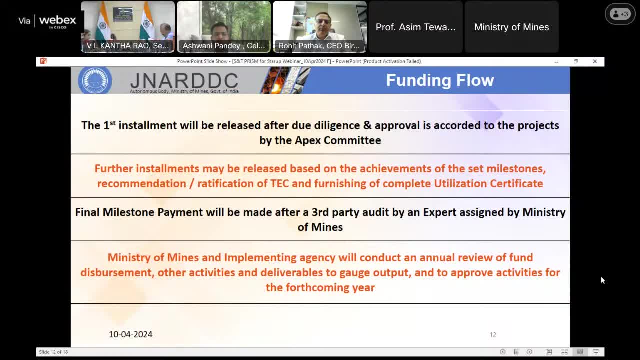 milestone. yes, that will be the criteria for releasing the the: the funding based on the recommendation or ratification, if required by the tsc, and furnishing of the complete utilization certificate. so this is what is required after getting the first installment. then the final milestone may be made after. third party: there will be a third party audit also before the final uh. 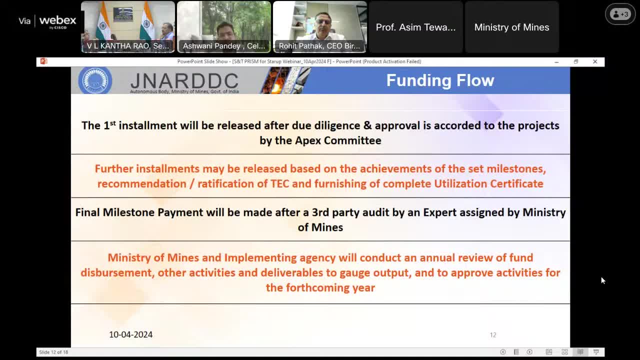 disbursement is made by audit by the expert committee, disbursement made by ministry of mice and ministry of mines. and implementing hc will conduct annual review of funds disbursement. other activities like deliverables of, to gauge output and to approve activities for forthcoming year. it will all depend on the progress made by the startups during the period. 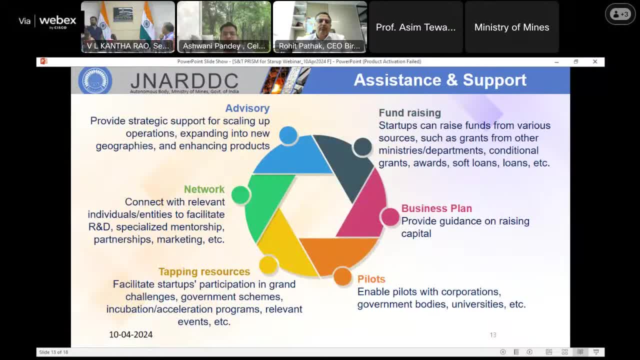 of two years next. please assistance and support. ministry of mines and implementing agency will be will be assisting. a kind of a hand holding will be done for fundraising. startups can raise funds from various sources, such as grants from other ministries, departments and whatever support is required from ministry of mines and implementing is. 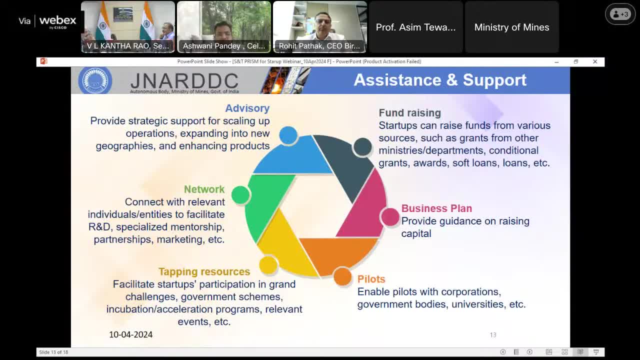 will be extended. business plan. provide guidance on raising the capital. minister of mines can interfere in there and provide the help pilots enable pilots with corporation, psus and universities. how to go from the startup to the pilot level. tapping resources. facilitate startup participation in grand challenges government scheme. how to line up. 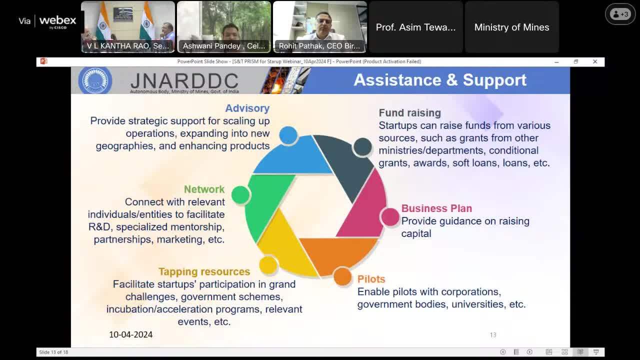 these startups with the government scheme so it can progress very well and meet the requirement of the country. then networking to connect with the relevant individuals, entities to filtrate r d or connect with the incubators. this kind of assistance can also be provided by ministry of mines and implementing agencies. 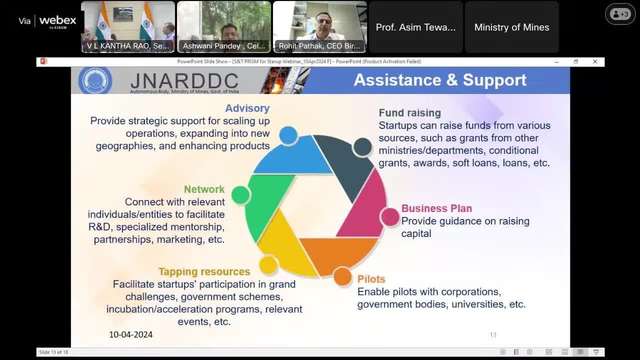 last but not least is the advisory: provide strategic support for scaling up operations, getting you connected with the psus, expanding into new geographies and enhancing product. so this is kind of assistance and support which will be extended by ministry of mines and implementing. next, please, opportunities are. 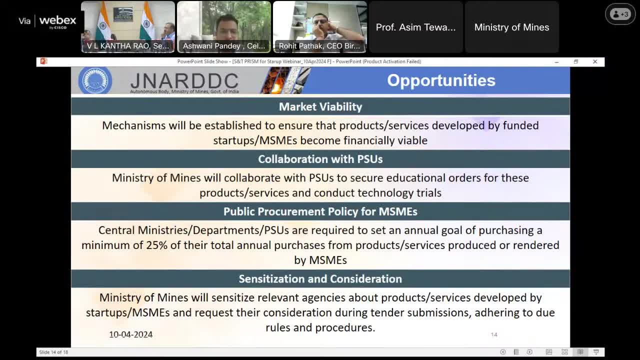 i mean i've listed only four of them, but there are plenty. market viable team mechanism will be established to ensure products become financially viable. collaborations with psu: that is kind of high hand holding provided by ministry of wines to collaborate with psu to secure educational orders, to promote your product, to take it at the commercial scale. public procurement: policy for msmes will be also supported by ministry of mines where 25 percent can be procured through the msmes. sensitization and consideration will sensitize relevant agencies about the product and services. all the platforms of ministry of wines and, of course, the government platforms will be used. 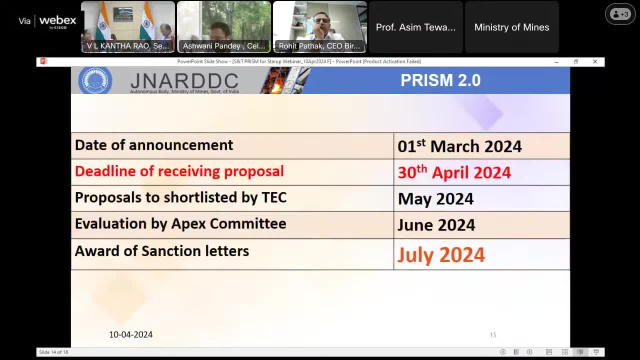 for that particular purpose. next now, prison 2.0. date of announcement was 1st march 2024, deadline for receiving proposal is 30th april and we see that the proposal will be shortlisted within a period of month, by may 2004, and evaluation by april of 2020. total plan, priority period of events and. 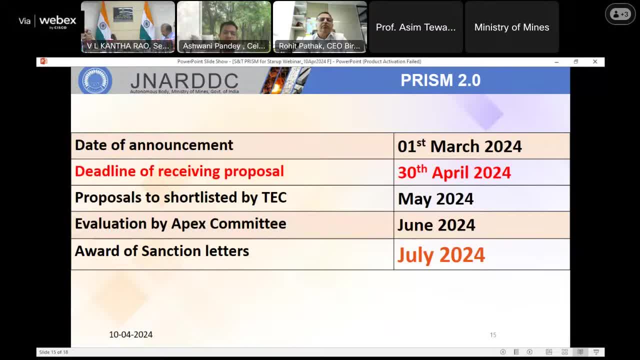 business in tele aiming services. support meeting- использ an termin, ripley 말�, İstanbul, MLK, its pex committee june 2024 and the award of sanction letters will be over by july 2024. so that is the schedule for the prism 2.0. so gear up. submit the proposal before 30th april 2024. next, 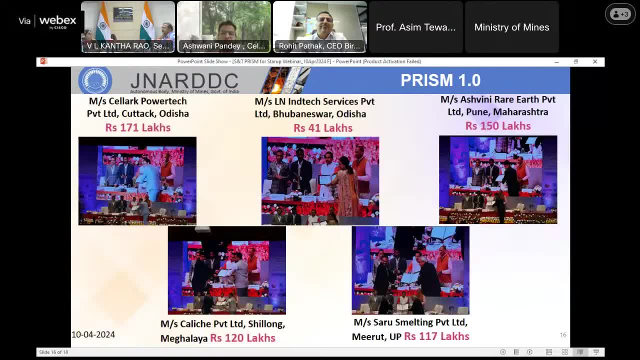 so this is a success story of prism 1.0. we had five startups. you can see the name of the startups and the area from which they belong to: 101.7 crores, 0.4, 1.5 and 1.2, except for one, which is: 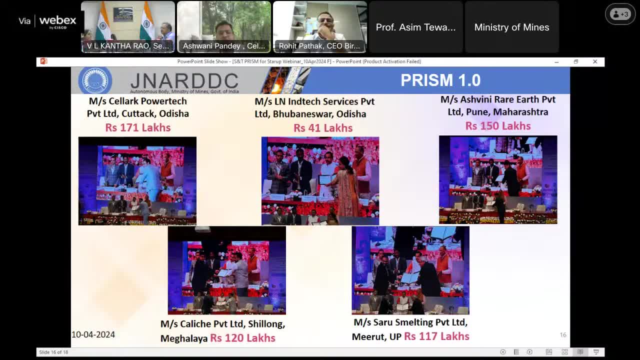 based on the software. three were on the deep tech. so this is the success story of 1.0, and we'll prefer to have more numbers in prism 2.0, because the funding has also been enhanced now and you have sufficient time to submit the proposal. last time it was only one month time, this time it's. 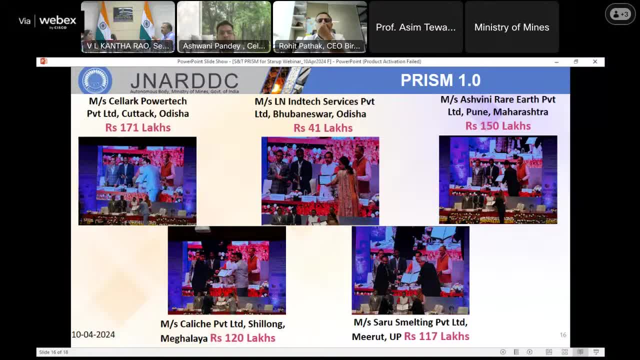 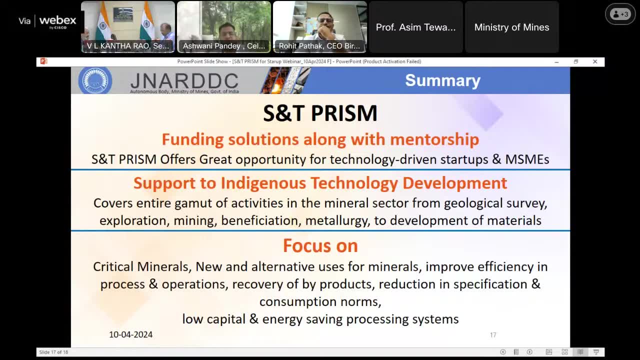 two months, so we expect more many proposals in the future. next, please. i think that's the summary. the fund snt prism scheme talks about the funding solution to have a connectivity between a talent and a startup, great opportunity for technology driven startups, support to indigenize technology development, which covers entire gamut of. 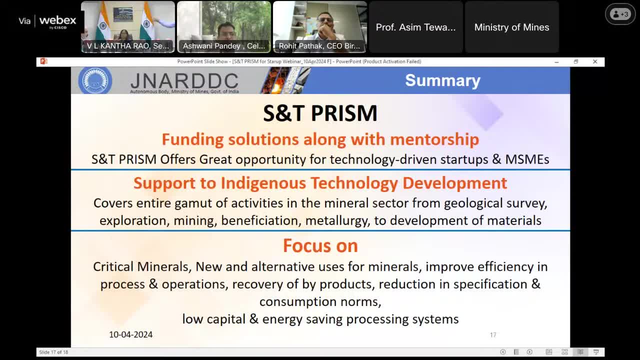 activities in the mineral sector, from surveys to metallurgy, for the product development, for the new ls development and, of course, this time the focus is critical mineralology, minerals. minerals- improved efficiency in process operations, recovery of byproducts, improvement in the specification of low capital, energy saving procedures. so all set to make india ivixit. 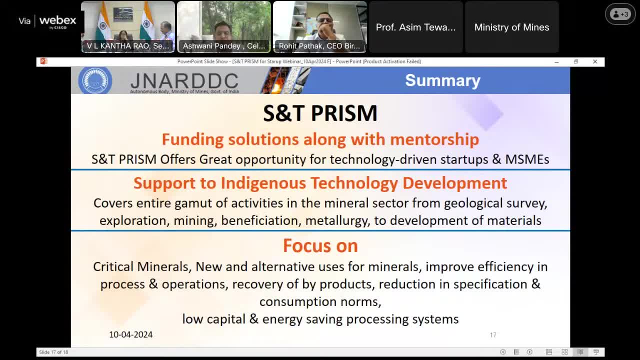 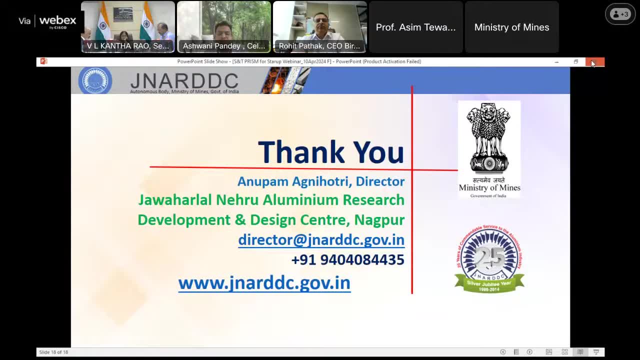 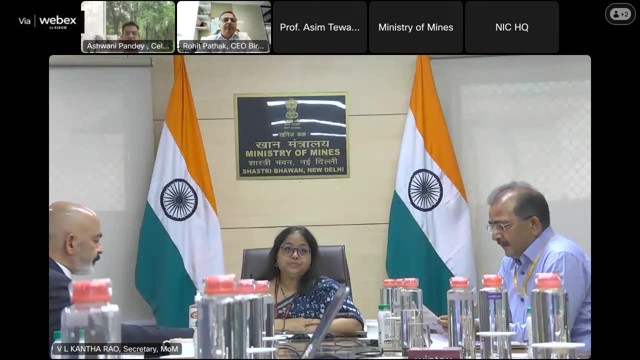 bharat a developed nation by 2047 through this startup scheme. so thank you, thank you very much for being part of us. thank you, thank you very much. so thank you, sir, for your nice presentation giving the detail about our startup of mining uh in general sector. now i'll request the sri amitash chena to give his opening remarks. 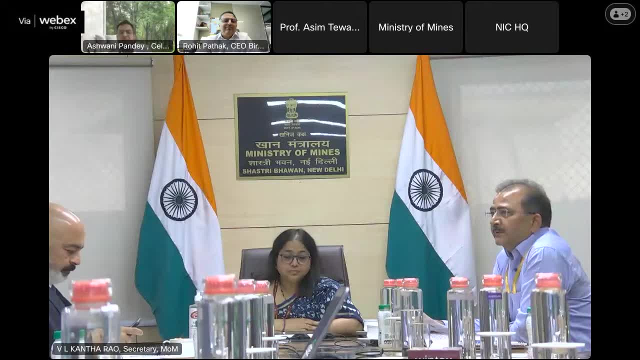 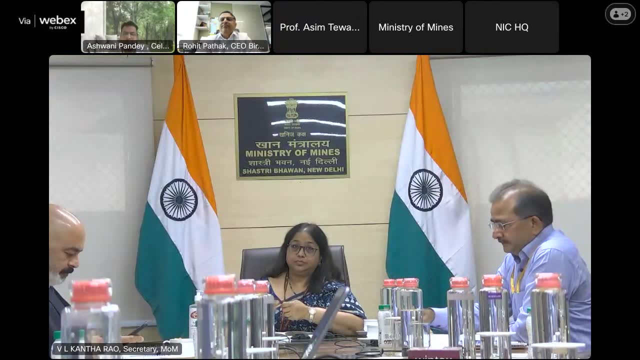 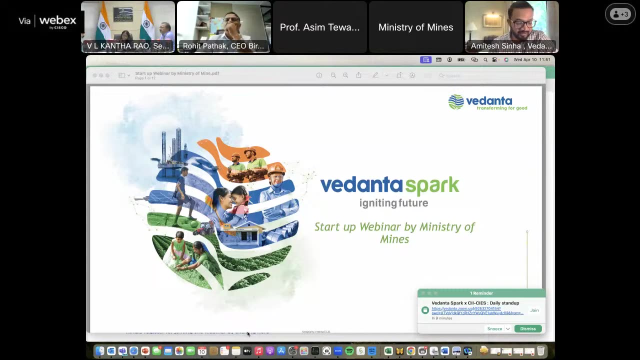 and also make his presentation on the subject. uh, mr sina, thank you so much. i think, uh, this is a great initiative, uh what we have seen from the ministry of mines. um, and a special thanks to the secretary, uh, kantarau, sir, uh, as as a general manager of the mining sector. so i guess we can call it a great initiative and we would love to hear your thoughts on this and share your thoughts with you. thank you, thank you, sir, as questions are coming in the next few minutes. uh, thanks sir, uh, thank you sir. this is a great initiative. uh, what we have seen from the ministry of minds, 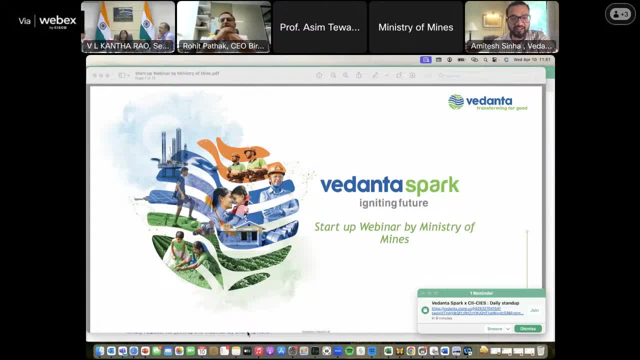 um, and special thanks to the secretary, uh kantar officer uh as as uh. by the way, thank you to our staff, for our jnrdc director was saying that he has made this possible and we are seeing that with the results and the outcomes. so this is, this is excellent. so i would like to talk about the vedanta spark. 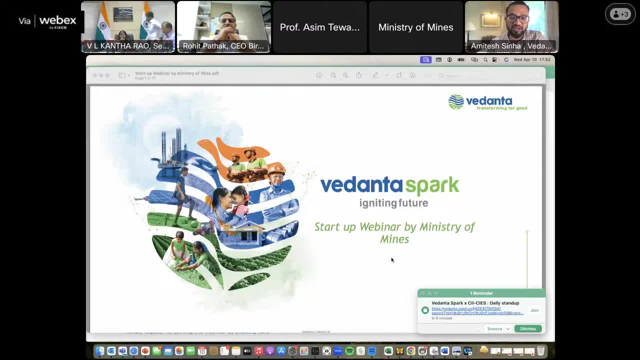 program which we are running and we are supporting the startups. so here i will run you through a presentation where we'll talk about how we are supporting the startup ecosystem and how we want to make sure that we are just not supporting startups to come and work with us, but in terms 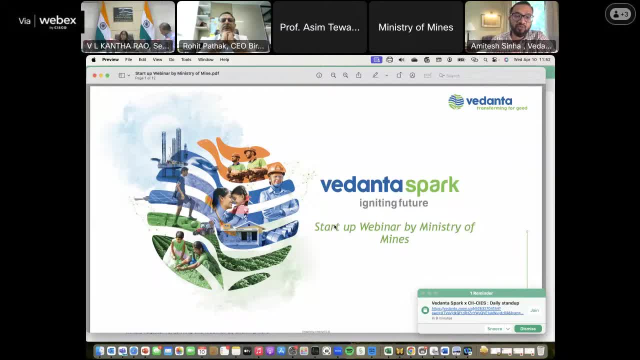 of how do we create an ecosystem with the startups which enables funding, which enables them to test their products, because you know the startups which we have worked with. what we have learned is that not only the funding which they need from the venture capitalist and other investors, the most important aspects of startups- 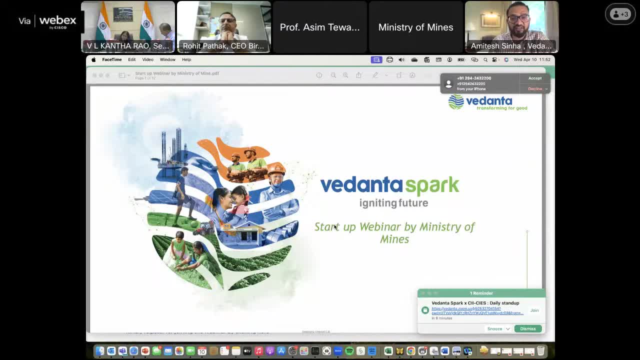 especially in the deep tech and in the manufacturing sector, is how they can get a support to test their products, because deep tech requires a lot of innovation, a lot of patience to come up with the product and some of the very critical mining assets when it becomes accessible to these deep 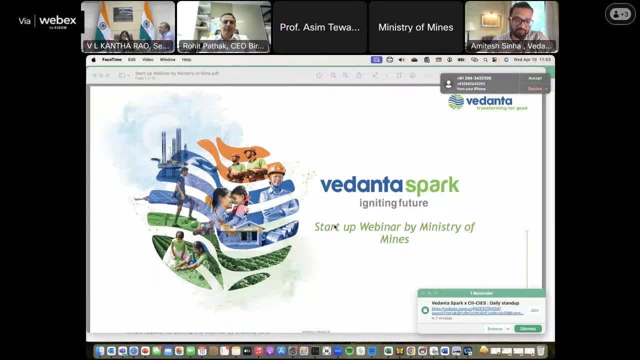 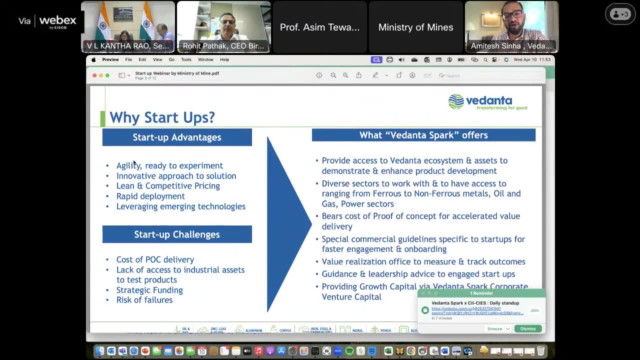 tech companies are very important. so with this, we would like to just share, as what at vedanta, what we have done. so, i think, why startups? um, so, because startups are, you know, agile. we have seen how flexible that can be and i'll give you some examples where we have seen that we were when we were trying to solve. 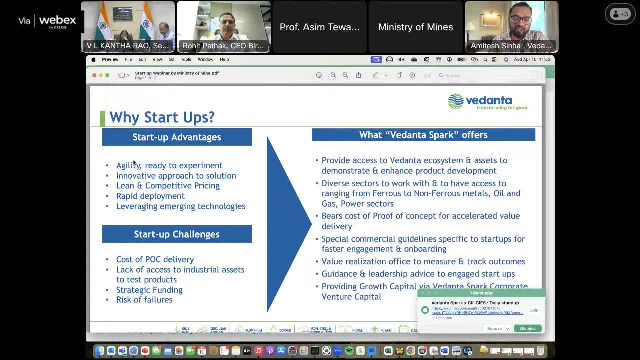 certain mining problems and how the, you know, the large oems were not able to kind of come up with a solution, but we were able to do with startups. so the agility is very important, the innovation which is happening. i think it is a very fast track which is happening with the startup industry. 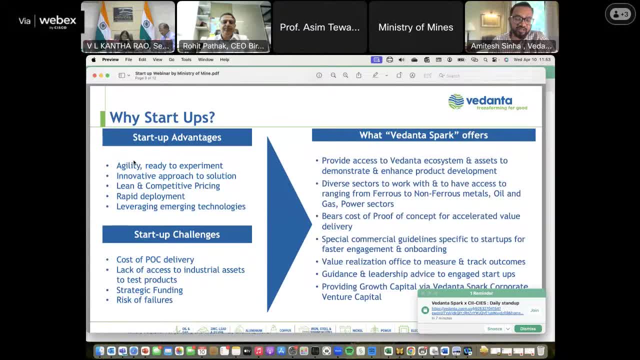 which is very fast, right, because if you're thinking about dimensions of China, is an engineer really, he's a marketer. it's quite a fast track because he can do a high cost business anywhere where he can get it to work. uh, yes, and there are other opportunities, right? so whatever i may be able to share with the startups. um just for an? um, if youub ISS start Entry Center, know, let's start with the startups. um just for an example, there are several rotary sensors which we can put in our mining equipment. um oem does not have those kind of sensors, which has um come up with. such a good innovation, but the startups are retrofitting and these startups are able to do it at a cost which is very reasonable as compared uh to the OEMs, so the cost reduction bringing the agility. rapid deployment is also very important and the emerging tech companies have less access to hire RSC trying to do this as well and thisיצong outdomination, because the 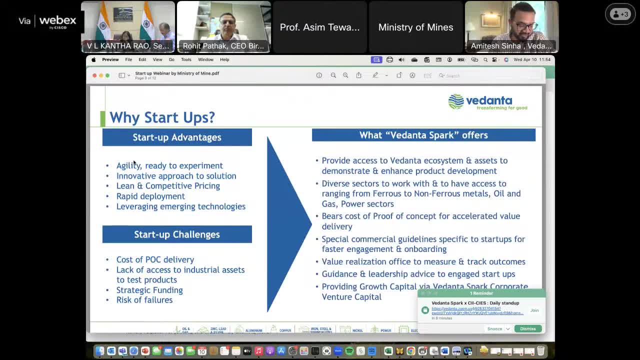 and the emerging technology kind of the research and the deep tech, what the startups are doing. we are able to derive from that. So with Vedanta Spark program, we are giving access to our assets and we are working with several startups to enhance the outcome through the innovation. 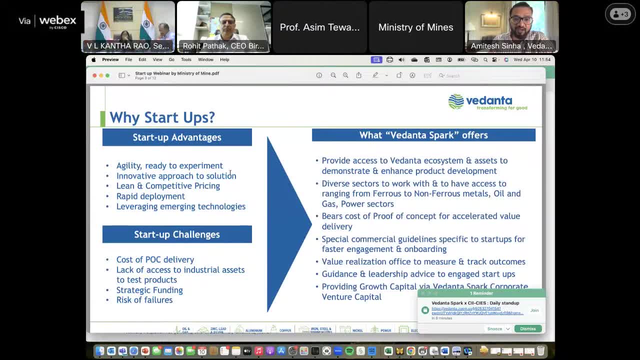 and the agility with the startup can bring in. So these are some of the things why we want to work with the startups, how we are creating the challenges We are working with our mining leaders across, because Vedanta is having a diversified portfolio when it comes to mining, be it zinc, aluminum, copper. 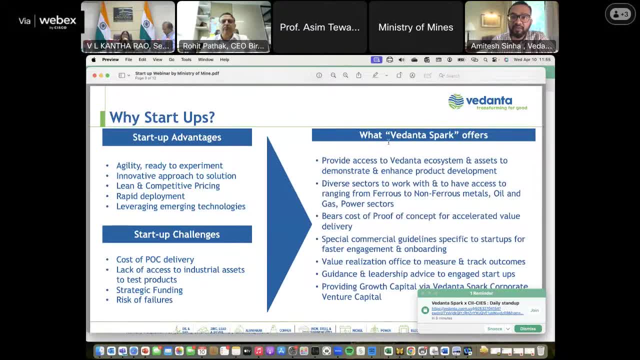 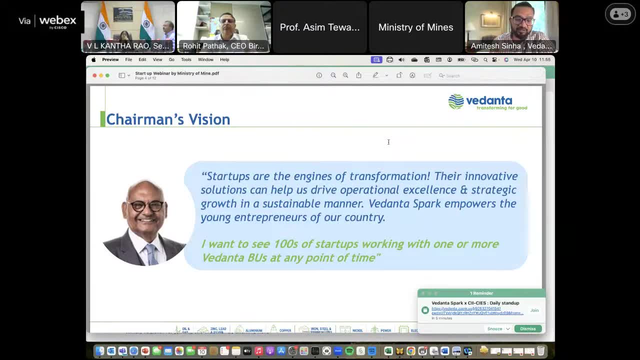 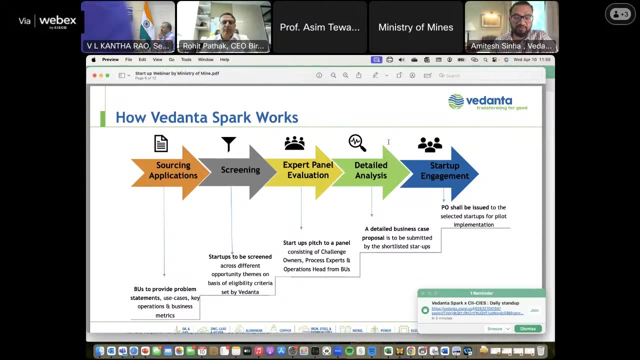 iron ore and so on and so forth. So the vision is we want to work with more than 100 startups. This is what our chairman and this is what we- the funding we have internally getting Now- Vedanta Spark, I think, is open for all. 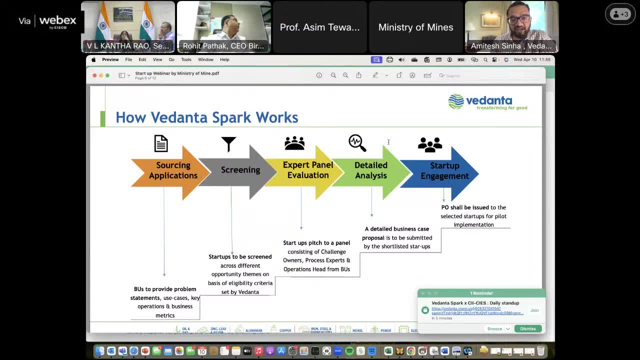 When we talk about mining, there are many AI and deep tech startups who can work with us And, as of date, we have worked with more than 80 startups and we plan to enhance these number of startups to beyond 100 and do a closer to 200 projects. 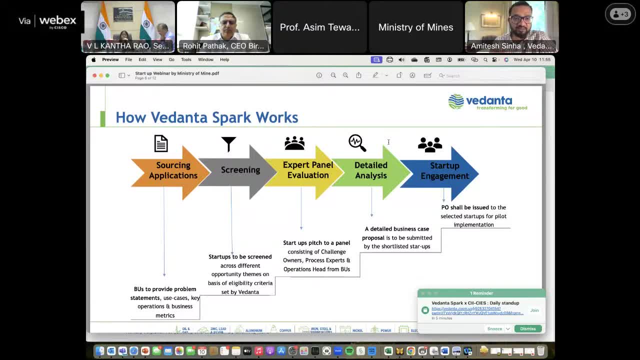 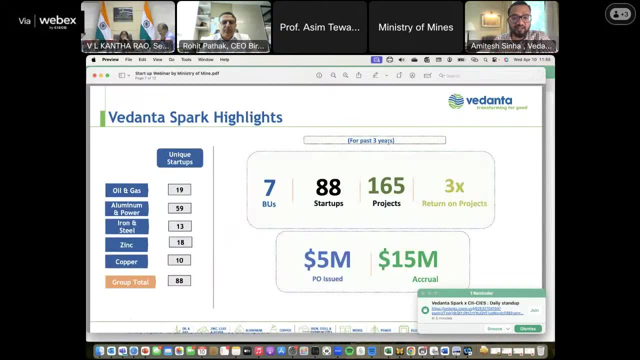 in this financial years. So we have a process where we take the startups, we screen them, then we put through the detail analysis and we engage with the startups. So this is a rough stat where we are In terms of startup. So all what we are trying to say here is: look, Vedanta. 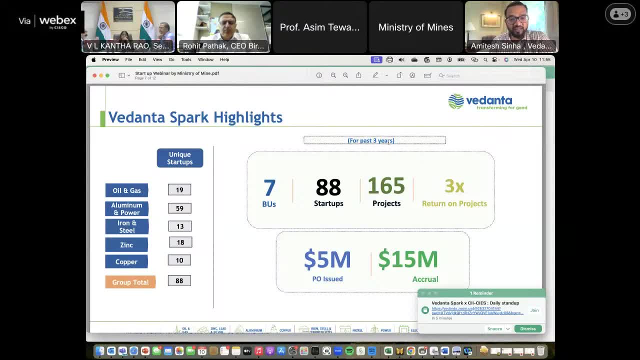 and, I think, with support of what the Ministry of Mines are doing and with the JNRDC efforts. we like to collaborate and we would like to see how we can bring more startups into the mining world, because it is a complex in nature. It requires a lot of deep tech technology. 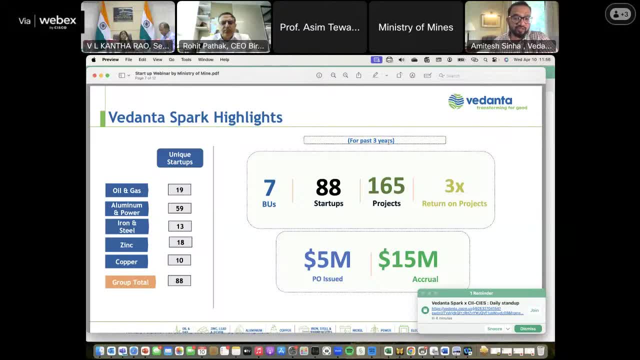 which requires a lot of time and patience. So we are here to support And we see how we can create an ecosystem of the startups which not only helps, say Vedanta, but it creates an impact on the overall industry of the mining itself. 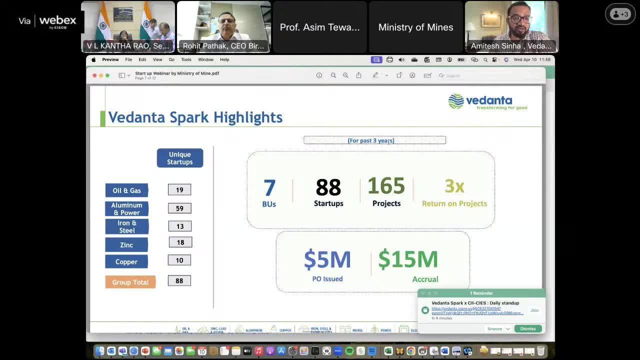 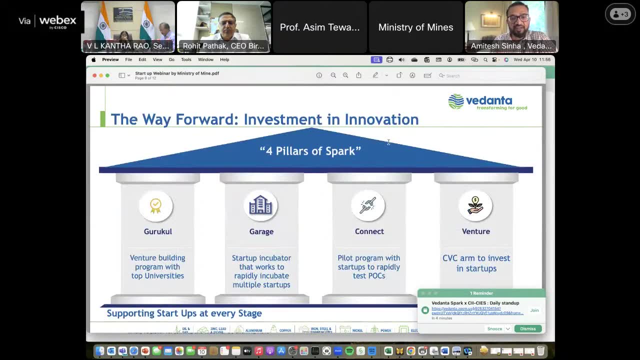 And that's why we want to be part of the whole synergy which we are trying to bring- and be part of the whole ecosystem- A very high level in terms of how we are providing or working with startups. We have the connect program where we do the pilot. 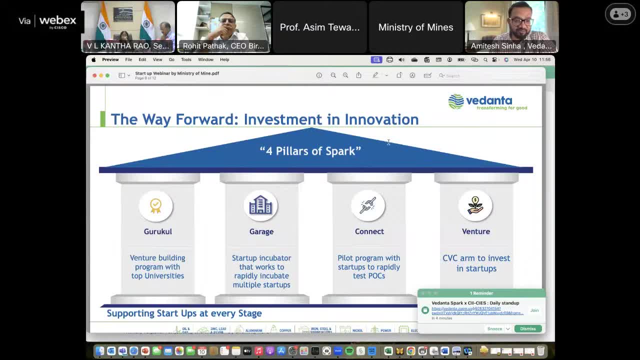 We have a kind of an incubator program which we are building. Gurukul is something where we partnered with university to see if we can do some specific research. We also have a CVC where we can invest and provide the growth related capital to the startups. 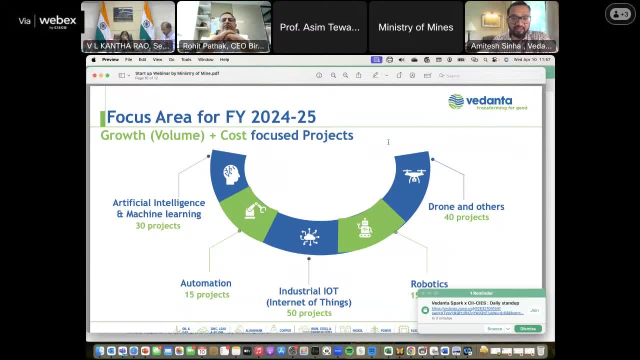 These are some of the very high level. you know the projects which we are focusing And maybe I invite any startups who are into this And we have listed all the challenges on our website, vedantaspargcom. So, in terms of you know all these teams where we want. 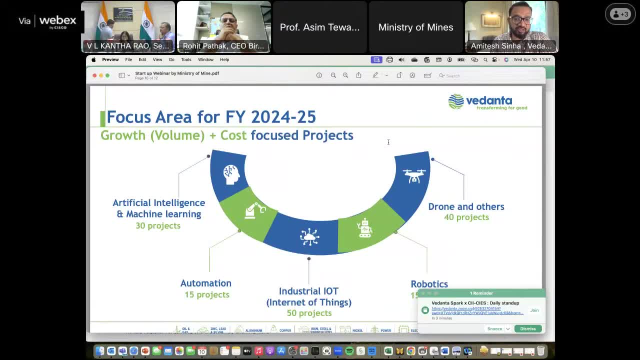 to work in terms of artificial intelligence, automation, IOT, robotics and drone and others which are enabling to do sustainable mining, And we are also focusing hugely of how we can reduce the carbon footprint because carbon capture which has come up and we want to utilize those emerging. 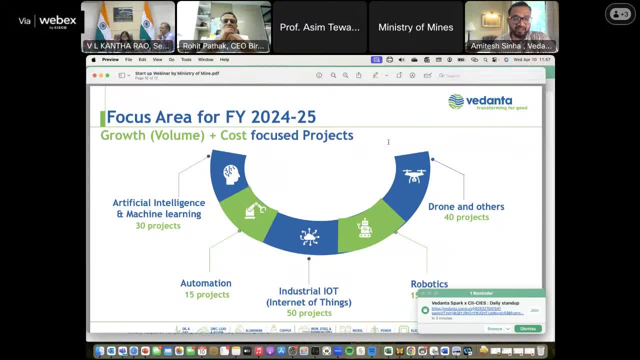 technologies, also to see how we can be part of the regenerative mining and reduce the carbon footprints and be much more sustainable from a climate angle. So this is something which Vedanta Spark is doing And we are very happy that we are partnering with Ministry of Mines to see how we can broaden the scope. 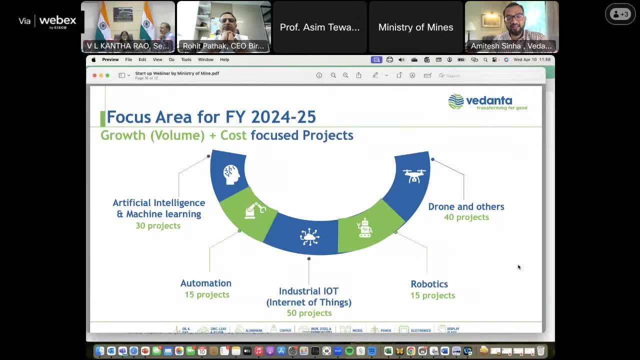 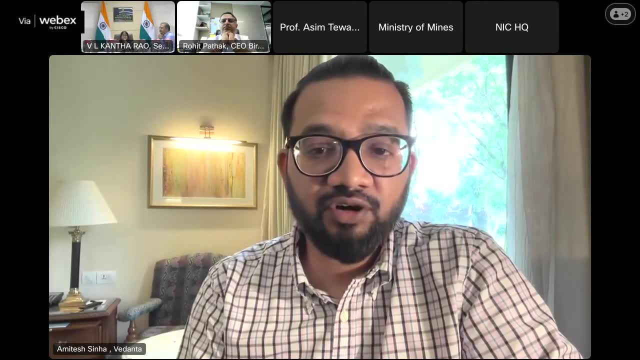 We can get more and more startups, And I think, look in the VC world, we have seen something called Death Valley, And Death Valley it's a really great startup project And it's really relevant for the startups who are into deep tech. 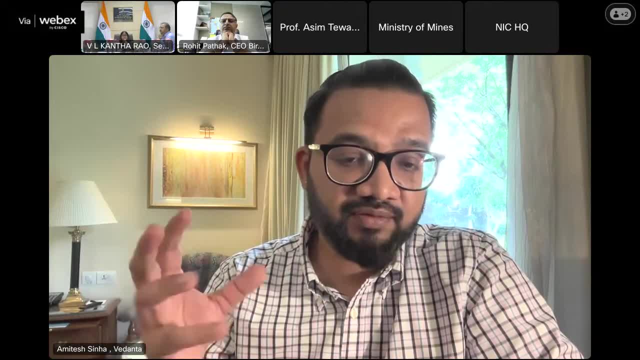 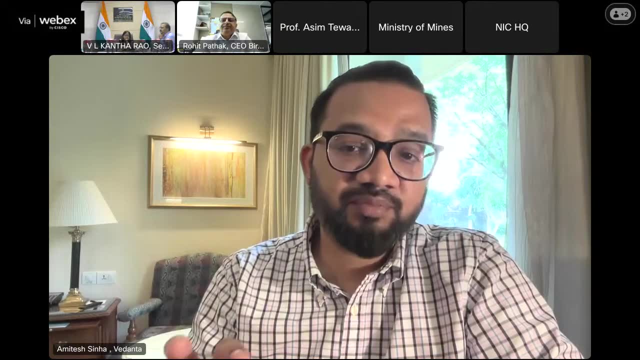 because deep tech curve is so high when it comes to the initial effort. And there's a point where you have, you know, you have created a concept where you want to translate that into a product And where Ministry of Mines, with this PRISM program, 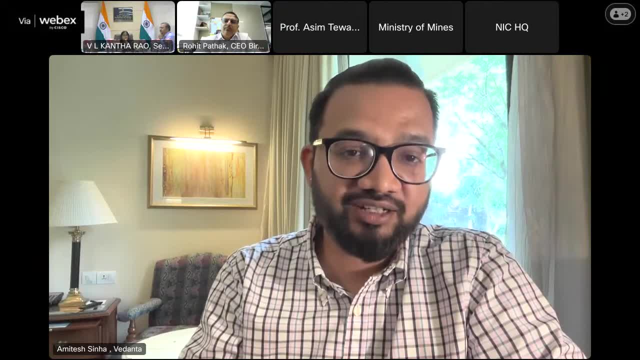 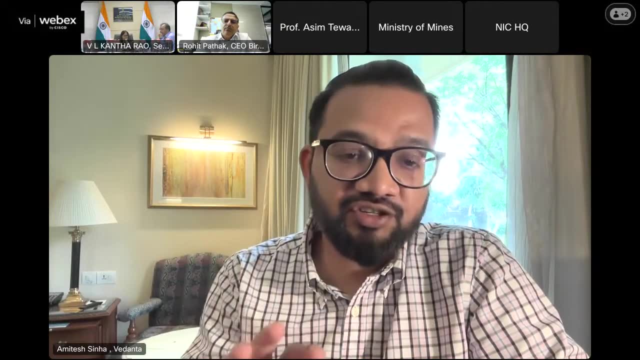 is supporting these startups is to support at the time of the Death Valley, as we call it in the VC world- is giving that grant Because we have seen, if you see, the history of the successful deep tech startups and even OpenAI got a huge grant from Infosys and others. 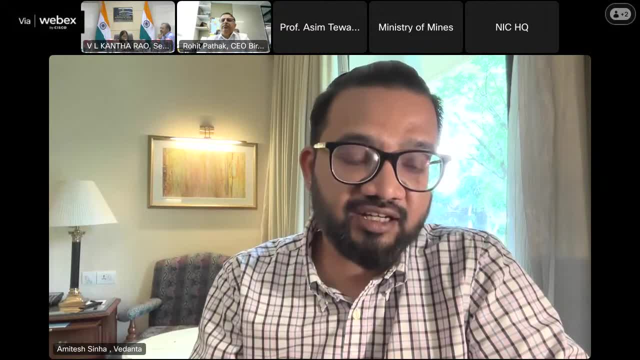 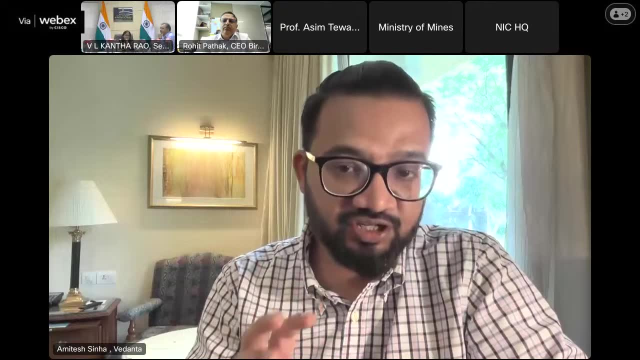 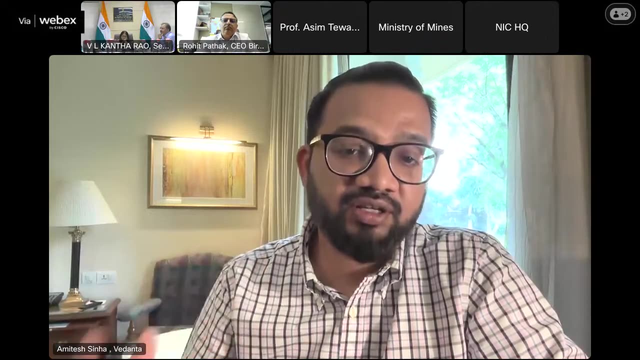 So that is a history And that's how this the nature of the deep tech startup companies is: that you need to have a non-dilutive capital support which is grant in nature to come from their research and commercialize and productize what that research can be. 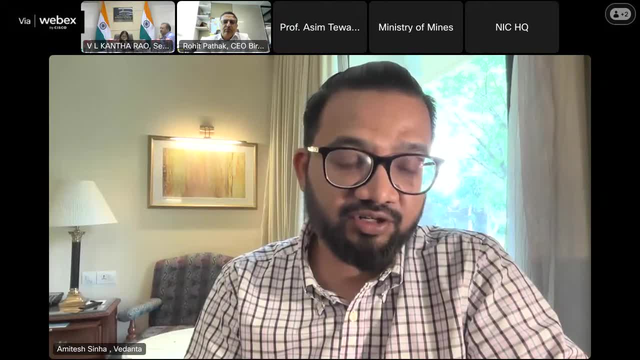 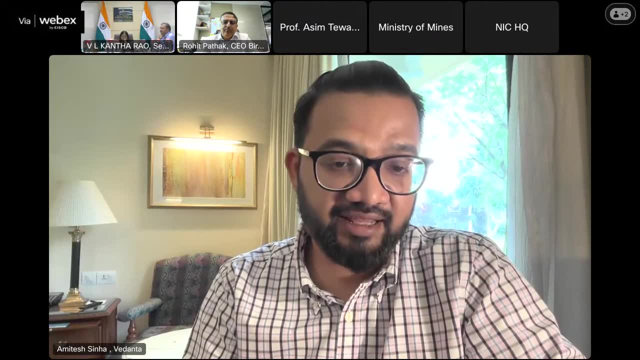 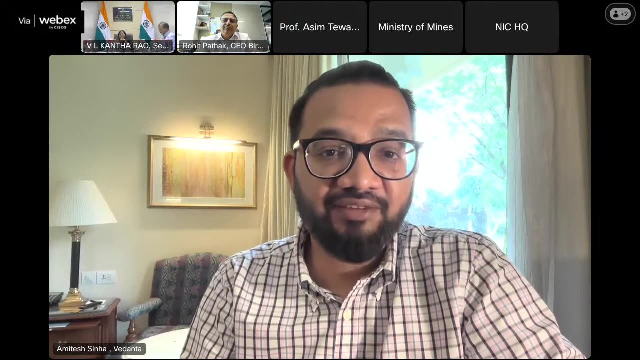 translated into. So I think this is a great effort and we are very honored to be part of it And we look forward as to how much we can support and create and enhance this whole ecosystem. So thank you, Secretary, and Farida ma'am for having us. 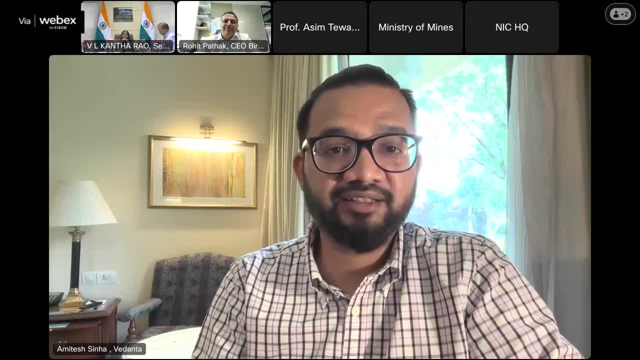 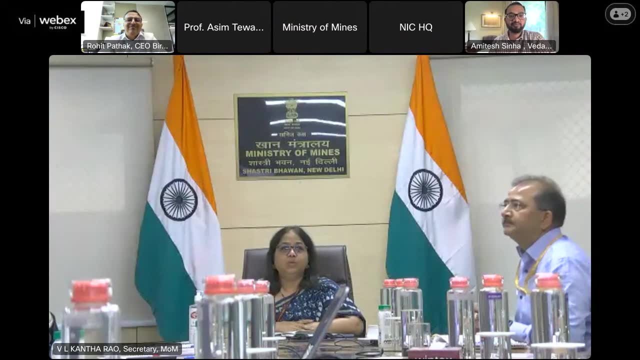 And then we look for creating a much larger impact. Yeah, Thank you, Amitesh. It was always nice. I remember when I first started looking trying to. you know I was trying to. you know I was trying to, you know. 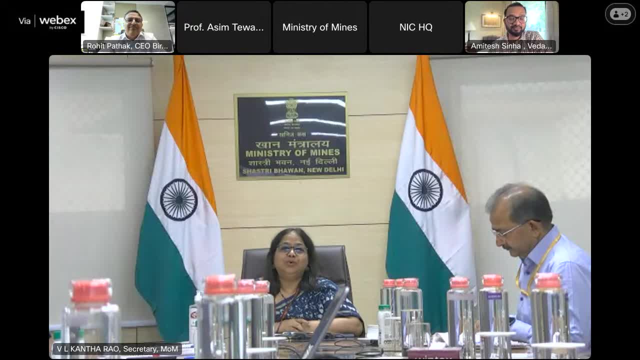 trying to do something with the startup, for as it was the place where I rushed to to have an idea about the entire thing. So that's the reason why I thought that in today's webinar also, I would like to have a participation of you and as well. 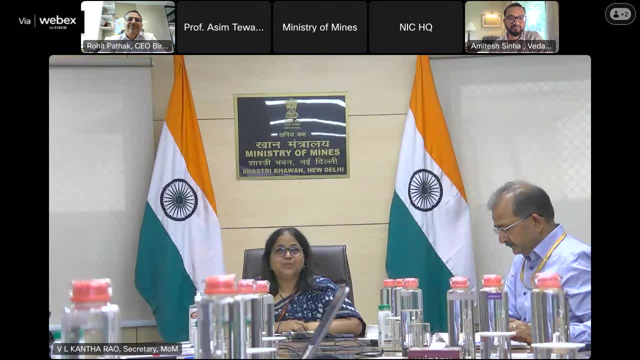 as in Indalco in the matter, besides the academicians. So thank you, Amitesh, for the insight and definitely we'll be working together in future also- And it's always- you will always be a part of our all startup- for summits and webinars. 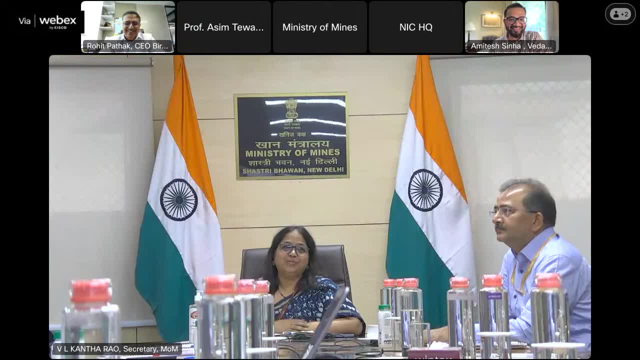 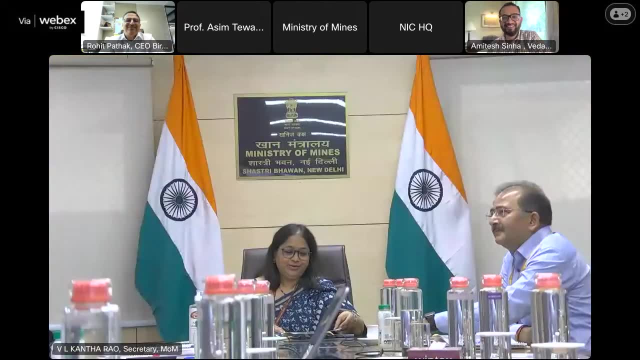 which we will be having to experience and encourage people in that. Thank you. That's a huge compliment, Farida ma'am. it's a privilege. Yeah, Thank you. And now I request Rohit Pathakji to please share your experience with us. 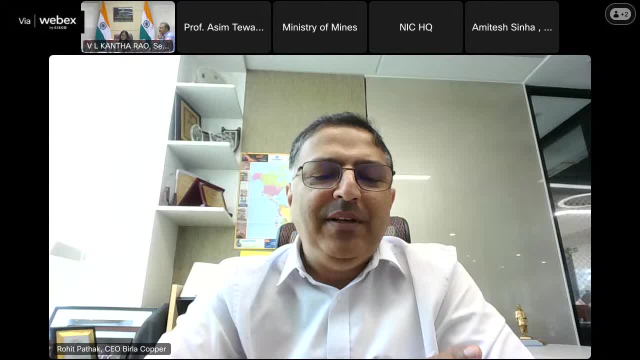 Thank you so much And I think at the outset you know let me share that it's a delight to be part of this session, Very happy to see such an initiative being the second iteration happening. Sorry, I was not so involved in the first one. 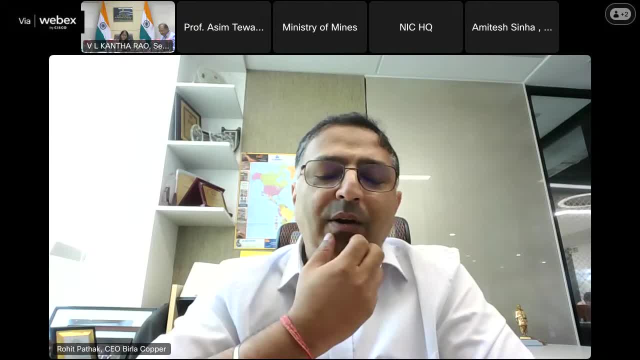 but happy to see the second one take off, You know, and not just as CEO of Birla Copper as part of Indalco, but also I was heading the Indian Electrical and Electronics Manufacturers Association, which is the parent association for the electrical industry in the country. 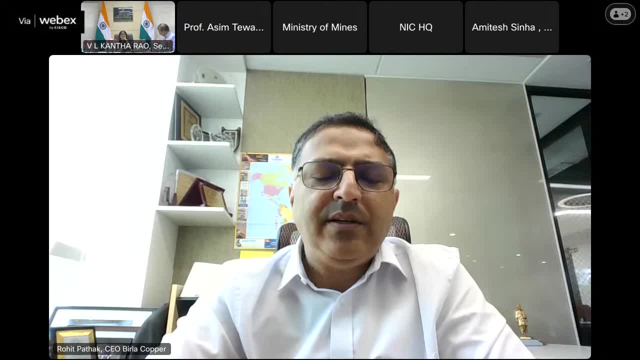 And there too, we started a startup program last year with the idea to encourage startups coming into the mainstream in manufacturing sector, Because I think to me the manufacturing and the core industrial activity is where, as a country, we have not drawn enough startups. 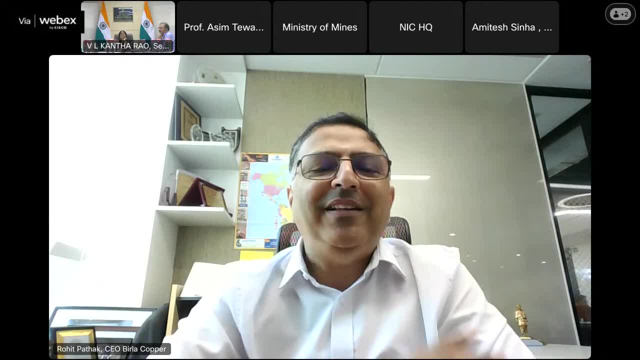 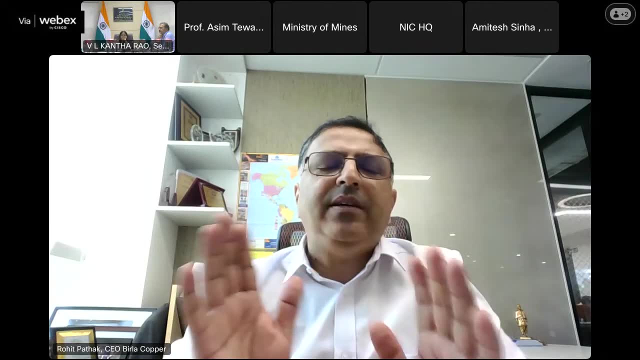 You know, a lot of it has gone to the software of the IT side, but I think there's a big, big opportunity And let me just start with, you know, sharing a few basic things on why I feel this is very critical. 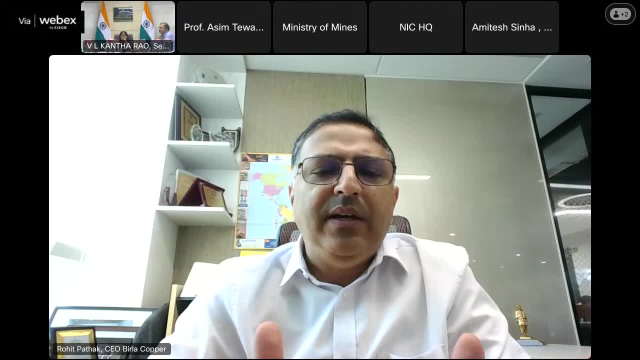 You know, all of us know, that this decade, maybe even the centuries of India's, the geopolitics are in our favor. The GDP is, you know, India is going to be the largest and the fastest growing economy And we will be home to over 25%. 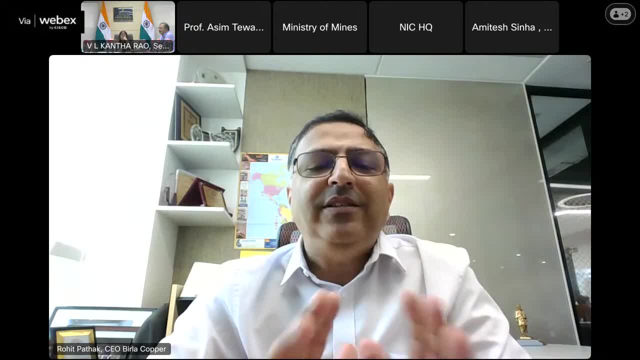 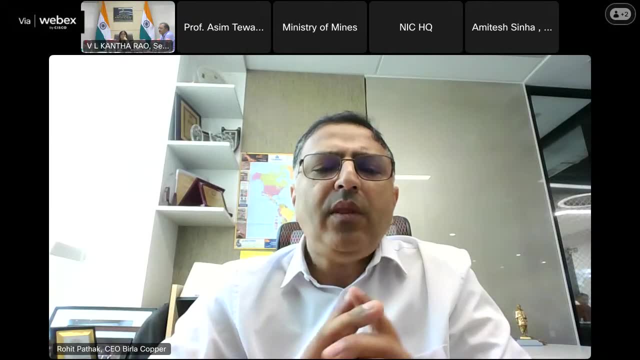 of the working age population of the world. So I think these three, if you just look at these three macros, you know there is everything going in the right direction for India And I feel, unless we really step up our game in manufacturing, 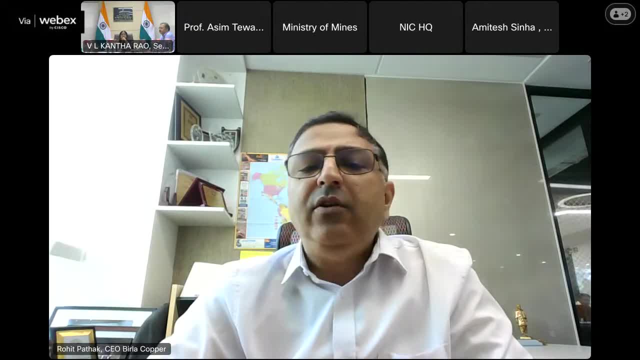 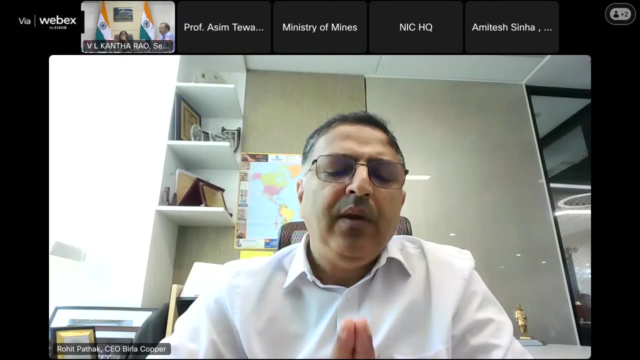 where metals and mining is a very core element, we will not be able to capitalize on this opportunity that presents itself, And an important difference for us in building this is going to be that we need to find our own sustainable solutions. There are a lot less resource intensive. 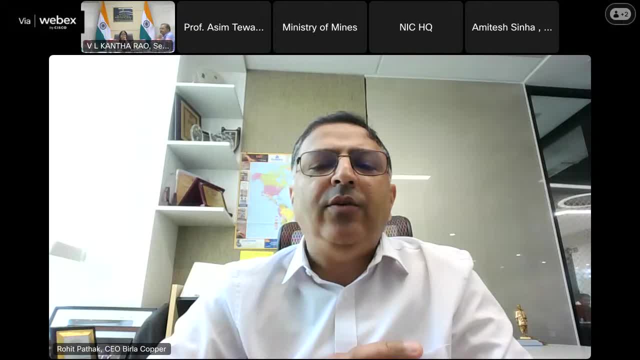 versus what the West has done in the past. So I think you know, historically, even if you look at- and I've been closely looking at- some of the startups that happened in India, many of them were started off as just copy of the models that worked in the West. 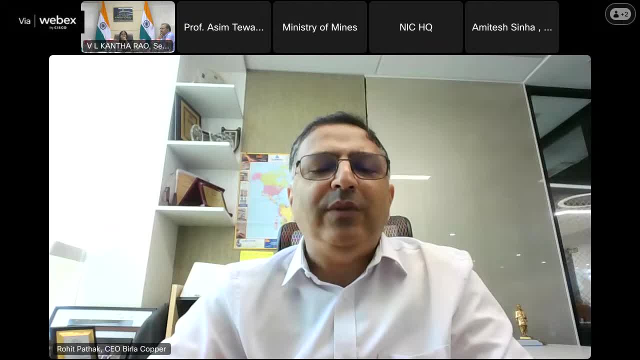 And you know, over the years people have figured out how to refine, tune them. Same in manufacturing. I think we can't just follow what has happened in the West. We need to come up with our own sustainable solutions in how we think about building some of the industries. 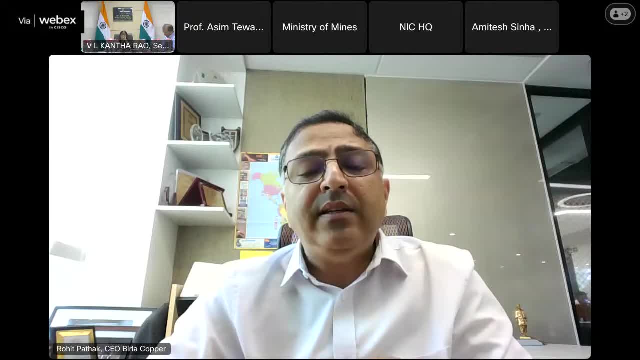 and industrial sectors that are critical for India. And you know I think we can't just follow. we need to work on this And I think we can. you know India As an example. I remember in the early 2000s when I was to visit China at that point. 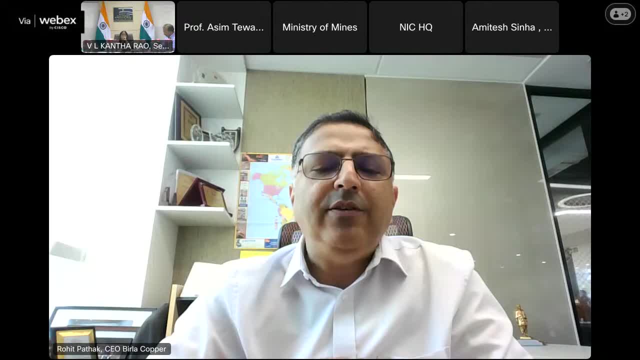 it was a very clearly stated statement that they used to talk about, saying: look, we will not be able to compete on the normal ICE engines in automotive, but in EVs we will lead the race right, And I think in the last 10, 15 years that is something that they have been. 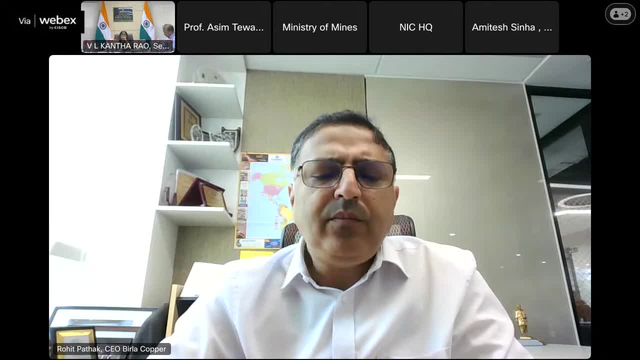 able to do where they are leading in the EV market. I think in India now we have the similar kind of platform. The scale at which infrastructure is being built is amazing And I think it is for us as industry, as startups, to leverage. 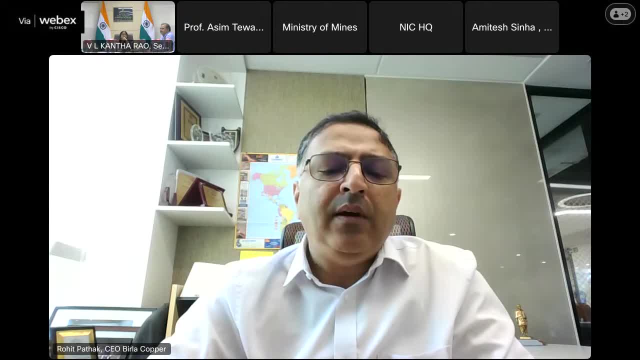 this opportunity. If you look at the program for the rooftop solar that has been just launched, the amount of investment that has been made in the infrastructure, the amount of investment that it will require and the kind of models that it can encourage, a lot of startups can. 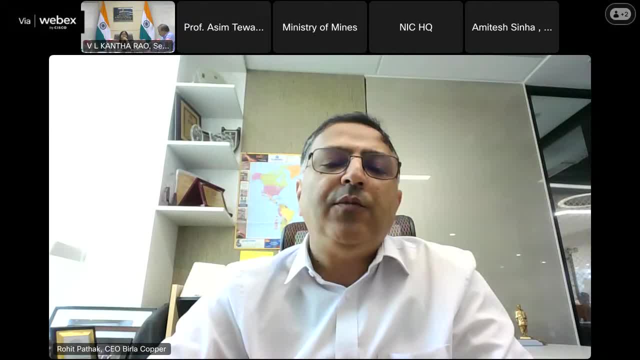 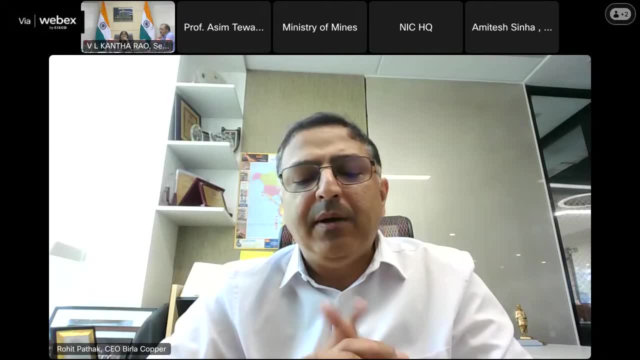 thrive in building solutions for making those work and make it happen in India, where we get to scale which can not just serve the domestic market but also the export market, And hence for me as an industry leader, there are three priorities as I look at startups. 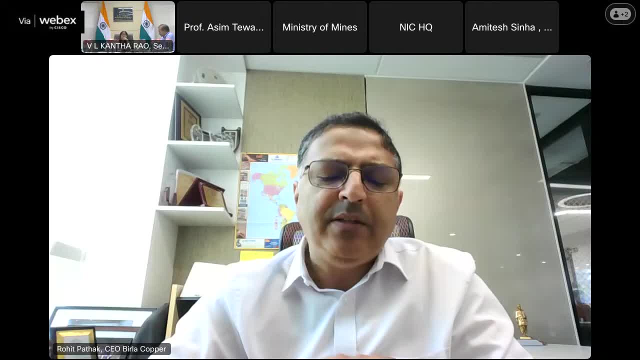 As Indalco, we have been leveraging and working with many startups across domains, but there are three domains that we We are very actively working on. One is around innovation around, And I'll give you a flavor of the kind of things along the value chain that we're working on. but one is around 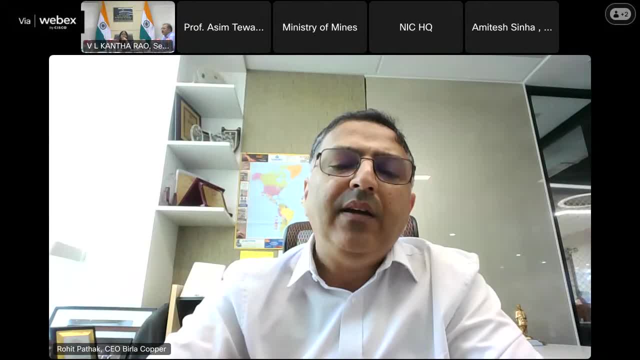 R&D and innovation. Second is around quality, And how do we improve quality of what we make in India, Because that's something which our Indian customer requires and also for exports is a critical part. And third is around skilling. I think a big part of what IT and tech can. 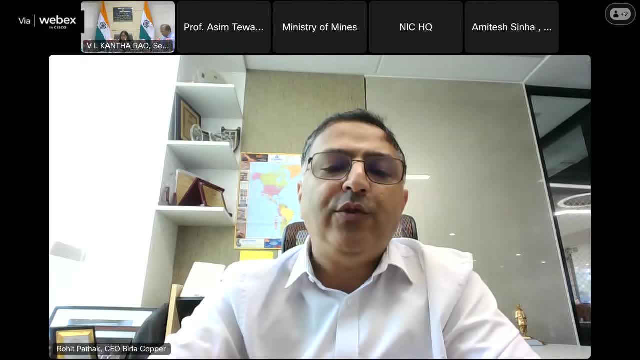 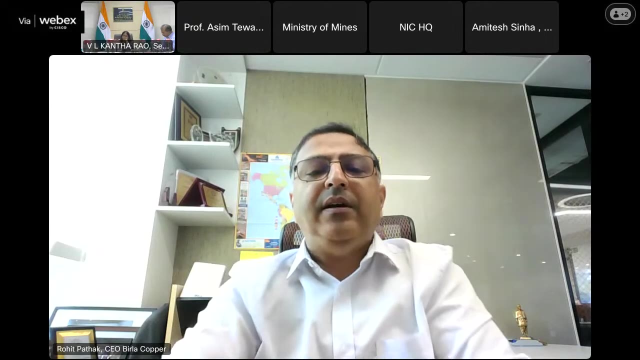 do for us is Accelerate the way we skill our workforces across the value chain. That's, I think, a big lacunae. A lot of models and startup opportunities are there for even skilling across the value chain, for processing metal processing, mining and stuff like that. 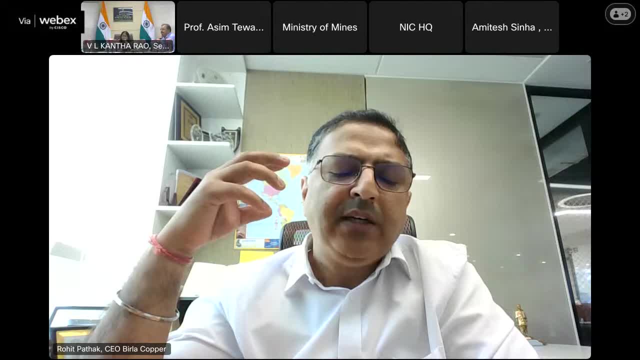 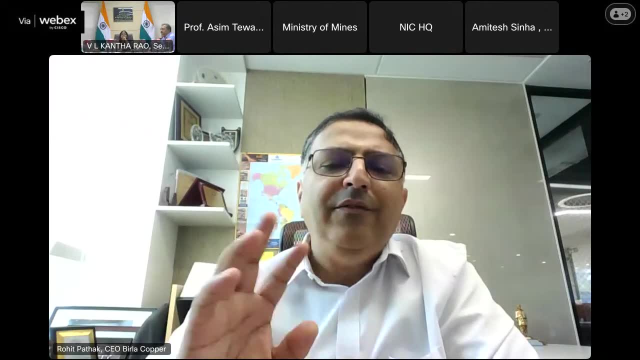 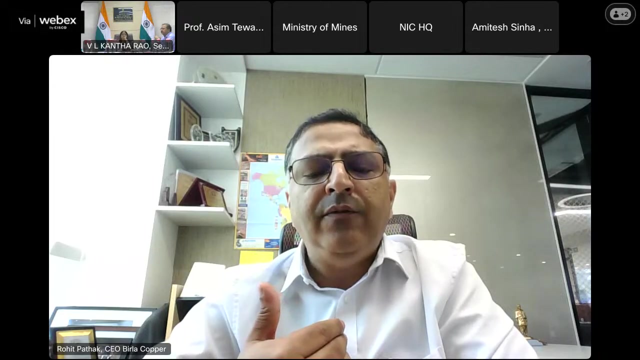 So I think- for us at least, the way I think of startups is- they are an extended R&D organization of companies. We as a country miss the R&D bus, but I think startups has given us an opportunity to leapfrog and drive innovation faster. So for us, if we are able to give you the right problem, 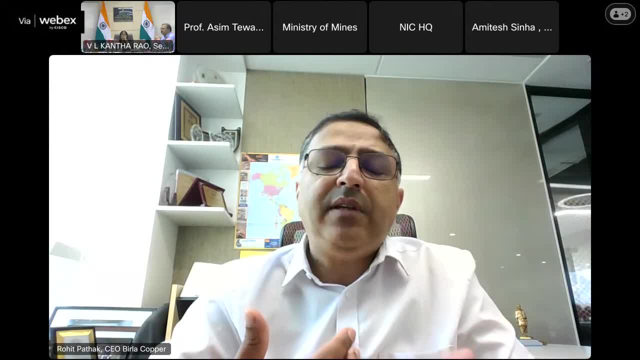 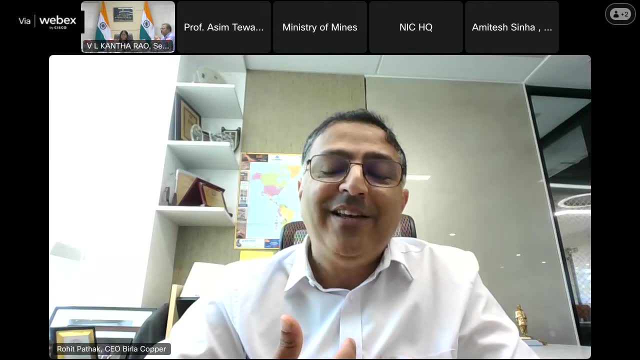 definitions of what we're working on. I think, to me, working with startups is a faster way of- And a lot more cost-effective way, by the way, of working on R&D on new innovation and new areas than the typical R&D of investment. 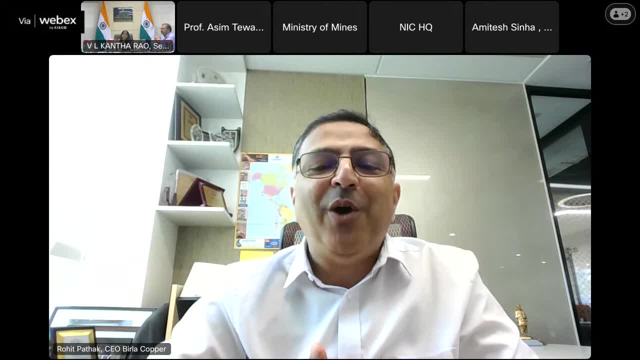 Okay, Thank you, Thank you, And I think that's something that we're all very proud of, And I think that's the way of investing ourselves, that was the normal way of doing business in the country, And I think that's one big mindset shift that we are going through. 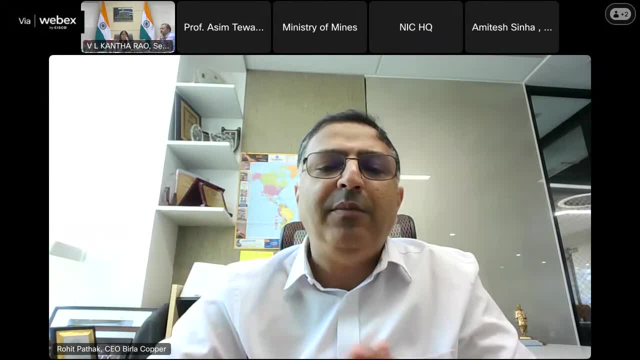 And hence very happy to see this industry, academia and government triangle that is getting formed to drive programs like this, which are important For India, and copper and aluminum, which are two metals which we are big in, as well as many of the rare earth materials. 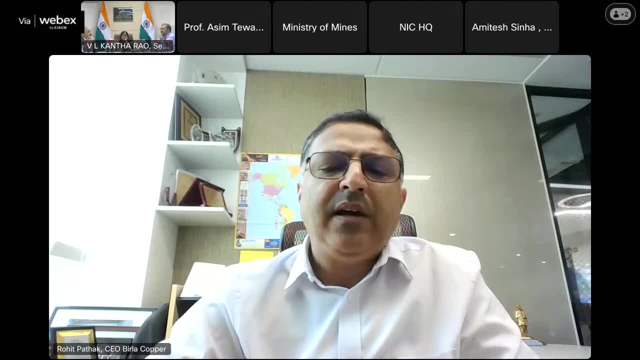 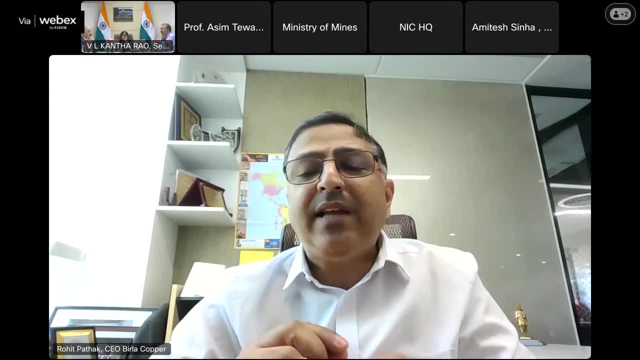 minerals are going to be very critical, uh, in the coming years, right across applications. these are the four metals where you'll see a lot of activity. we are just scratching the surface at the moment, right, uh, we have to. we have an opportunity to grow 10x in the next 20 years in each of these. 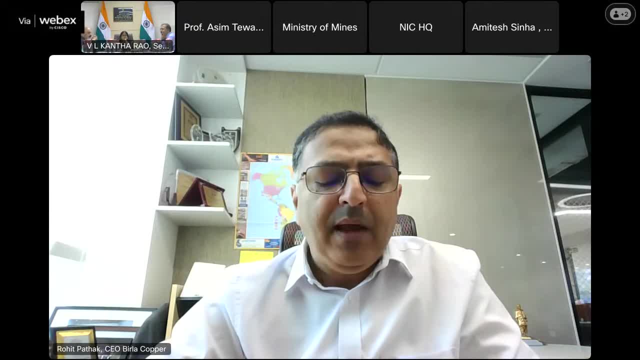 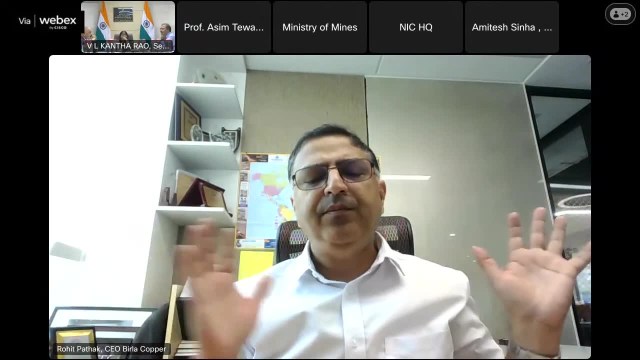 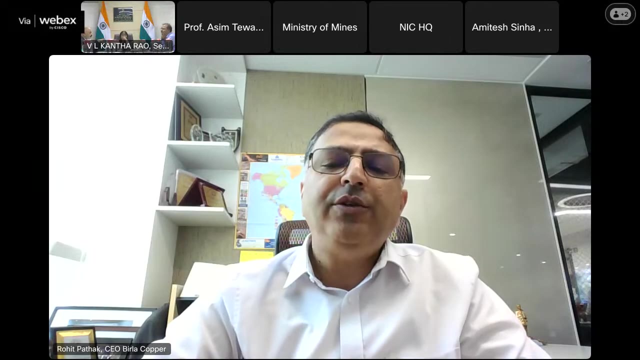 minerals. if we really uh address it well, and you know, hence for me the way i am looking at the startup opportunity, there are four distinct elements. there is, of course, the mining side- i mining exploration side, where i think the secretary also mentioned. there is a lot of opportunity uh on 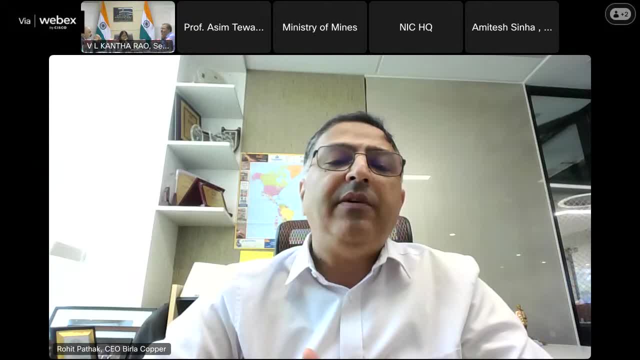 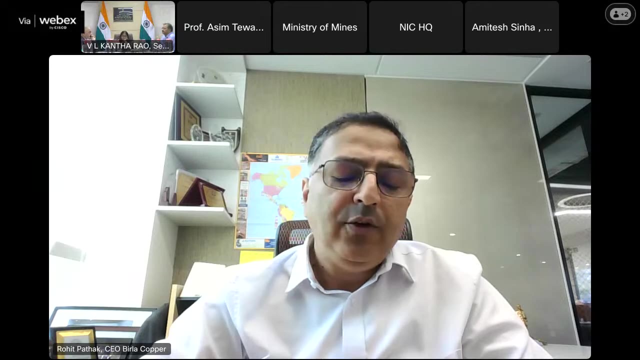 data analytics and geo mapping to discover a lot of minerals in india. india is one of the least discovered or explored uh geography in terms of mining resources and there is a lot of potential, especially with drones and ai technologies, to drive exploration uh in the country. the ministry 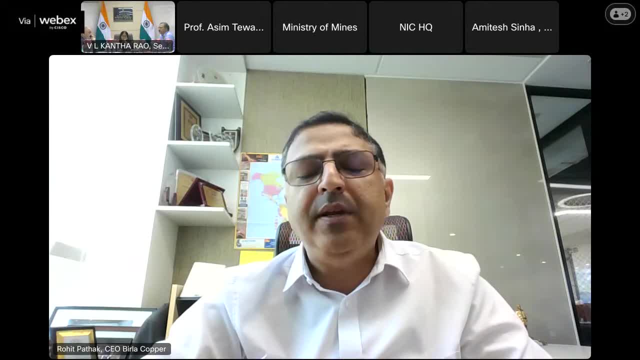 has taken, uh you the very bold step of opening up mineral resource mines for exploration and composite licenses, which many of us as industry have gone into. but, to be frank, i think you know we, uh we need to build the technology to be able to do this smartly and fast, and that is where uh resources- i know startups can. 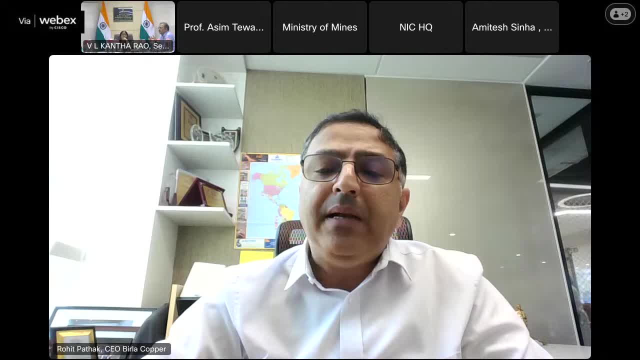 play a big role. the second big area is melting and refining of minerals. i think this is a huge area. even today, when we go for technology, uh, for building a new smelter or building a new refinery, you either have a chinese option or you have a european option. 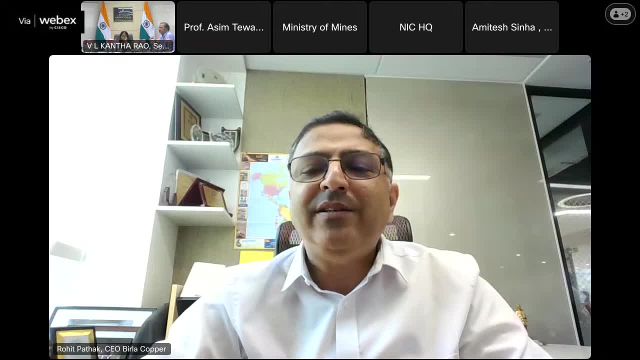 the chinese is uh fast and uh maybe not as reliable. yeah, some of us racist. going there- european, on the other hand, is very, very expensive and takes too long. right, there is no strong indian uh technology which is uh existing in many of these areas, and i think that's one. 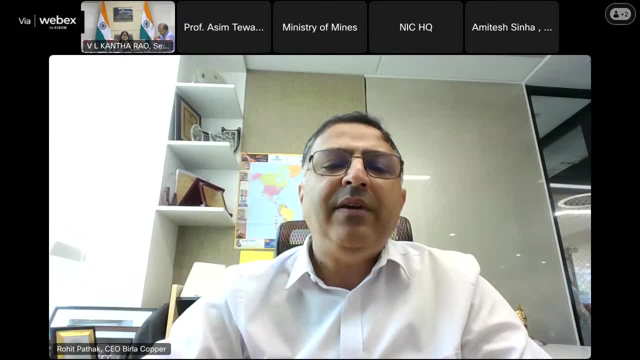 especially in the rare earths and some of the newer metals. it's an area where a lot of uh scope is there. it's a area where a lot of uh scope is there for uh, this kind of uh. it's a very scope is there. There is a big vacuum. 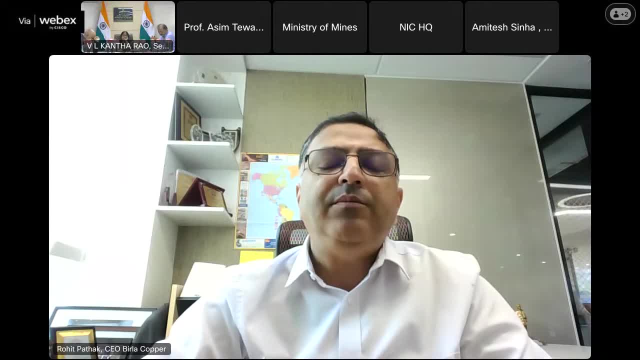 for someone to come in and come up with new technology processing suggestions on how we can extract metal better, how we can improve the processing. A lot of AI we are leveraging, where we are now working with some startups in India to improve our process efficiency. 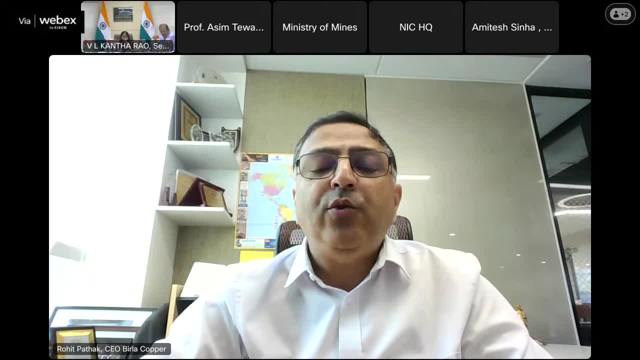 build digital twins of our smelters, do thermal mapping of refinery to find things like shorts in the refinery circuits. proactively, I think things around reducing and reusing a lot of the waste that gets generated in the processing setup, whether it's copper smelting. 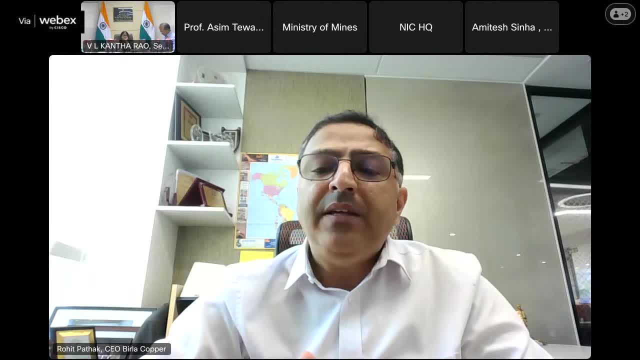 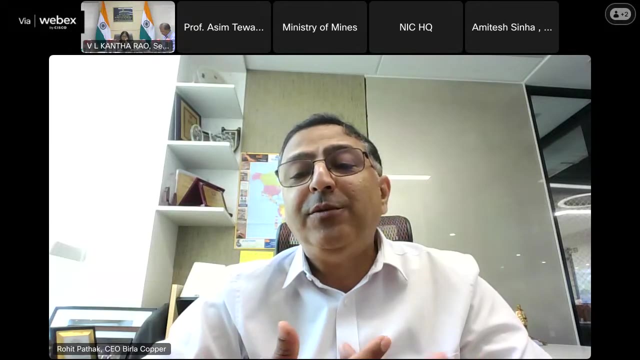 or whether it is aluminum refining. a lot of waste gets generated which can be reused for repurpose, for useful applications, And that's a very big area where I think many startups can play a very active role, because it's a huge value creation. We end up paying today to dispose. 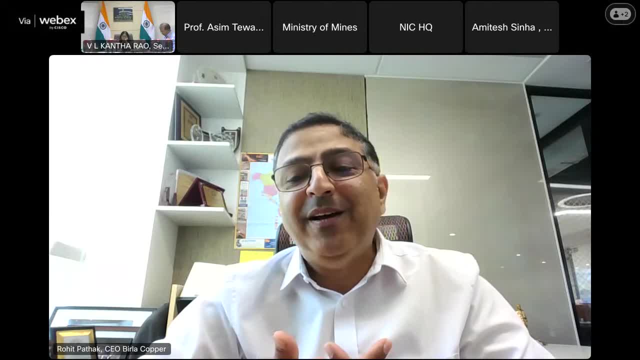 of that waste Now. if you can create some value from it, it's a win-win for all of us. Apart from saving resources, I think there's a huge potential in the waste handling part, or by-product handling part, in metal processing. 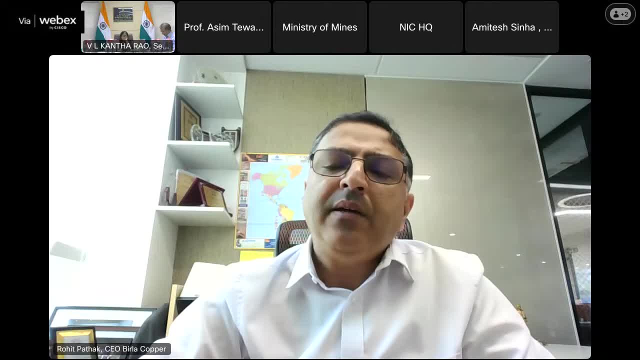 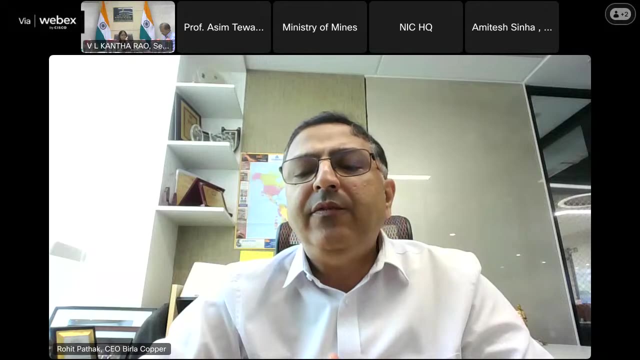 Third area is around downstream. A lot of products need to be developed in India, A lot of alloys, a lot of design options where I think startups can play an active role. For example, as we look at high-speed railways, there are different. 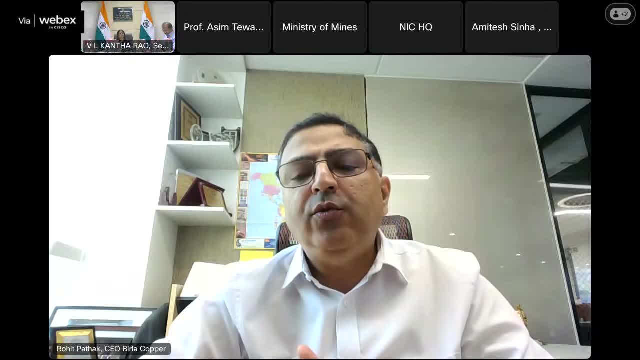 alloys of copper which are required to be made to handle the high-speed railways. I think big opportunity for new products and new alloys to be developed. You look at, like I said, the rooftop solar scheme, A lot of copper products today and aluminum products. 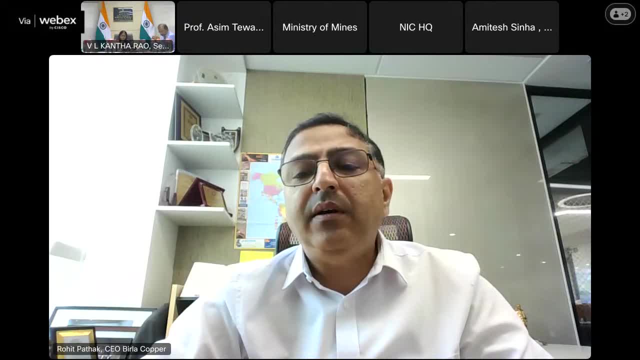 they're not made in India. They are going to get imported from countries where we do not want to import material from, And opportunity for many of you to get into making those products in India which provide you a very quick scale-up if you get it right. 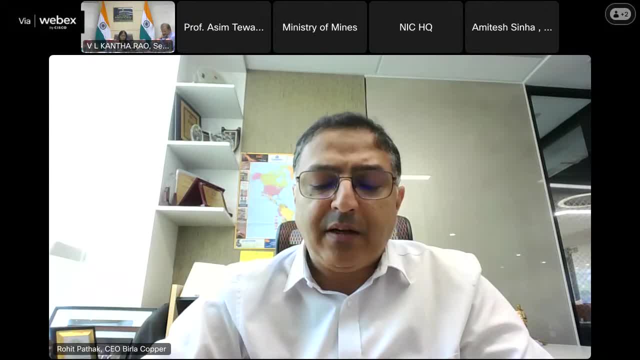 to indigenize and drive products in India. And the fourth area is around recycling. I think Dr Gingal-Othri also shared JNR. DDC has taken a step forward in that where I think we are currently not doing recycling enough. 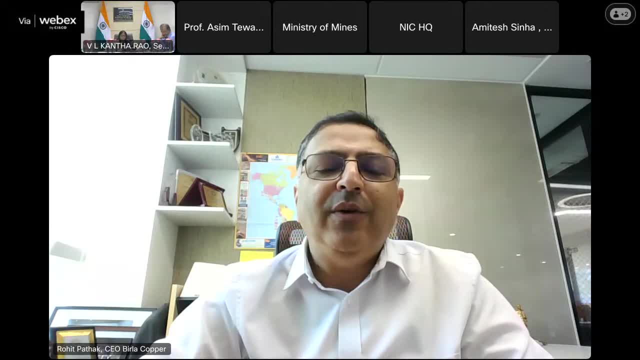 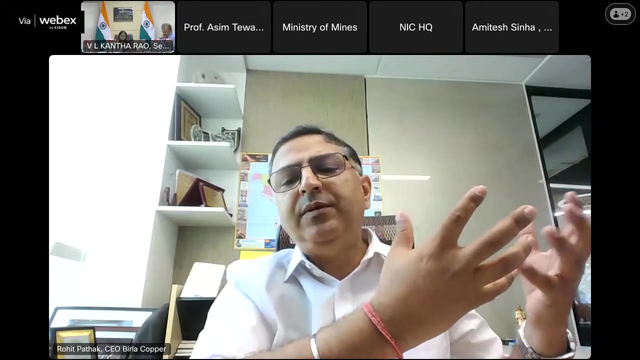 A lot of what we do today is remelting and not really recycling, which can make products back to the original specification of metal, And I think there's a big, big opportunity there to both look at the collection mechanisms, which are a different type of startup We have. 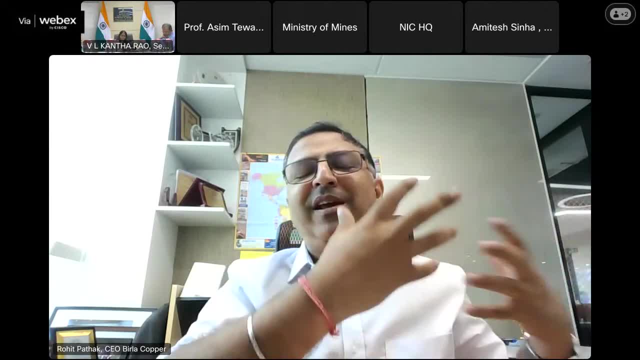 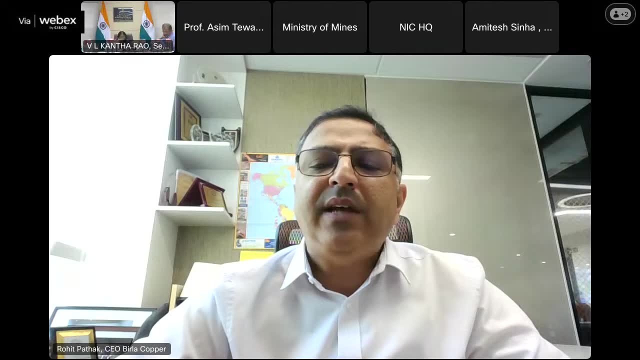 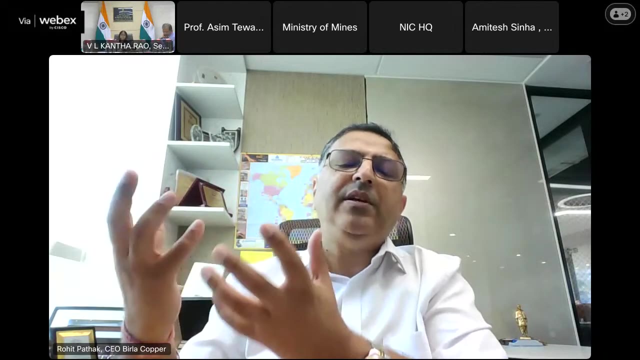 the Swiggy's and the Zomato's of the world, which have created a collection and a distribution mechanism which can be leveraged for creating the collection of scrap and recycling material. There is a lot of technology required around the segregation and pre-processing. 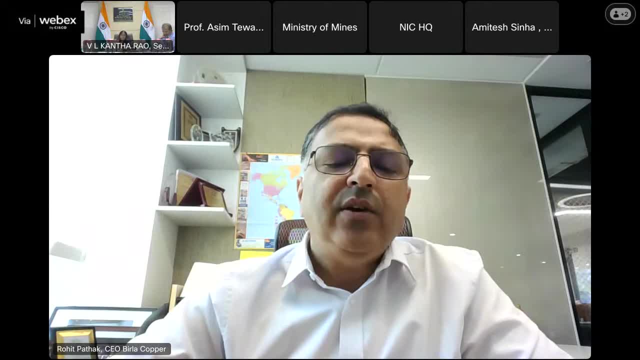 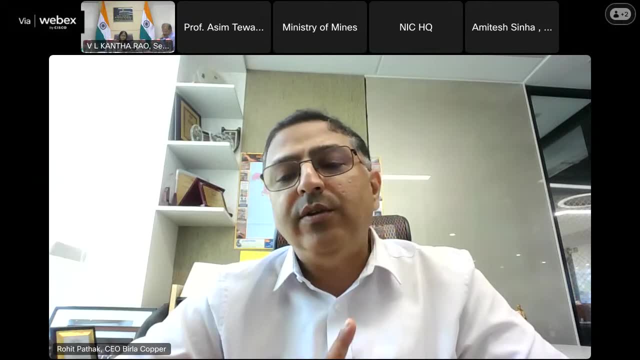 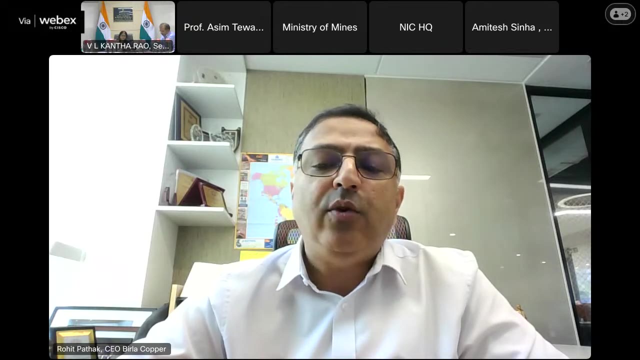 of the scrap And then, of course, around the final processing and recycling of this material into a re-purp or useful metal back again for the original use, Whether it's batteries. you look at, for example, the program of smart meters that is being rolled. 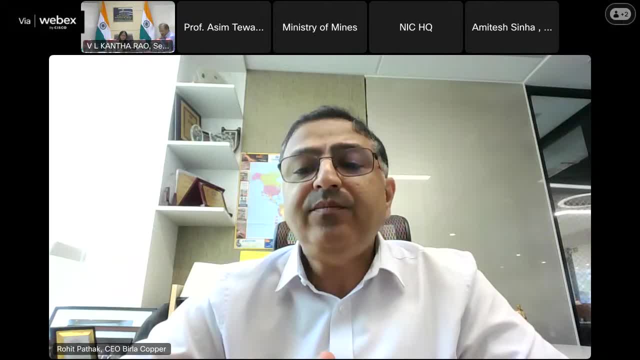 out at a scale which is no other country has seen. But while we launch and we set up new smart meters at home, there will be a lot of old smart meters or old meters which will be taken out. A big opportunity to recycle and leverage that material back. 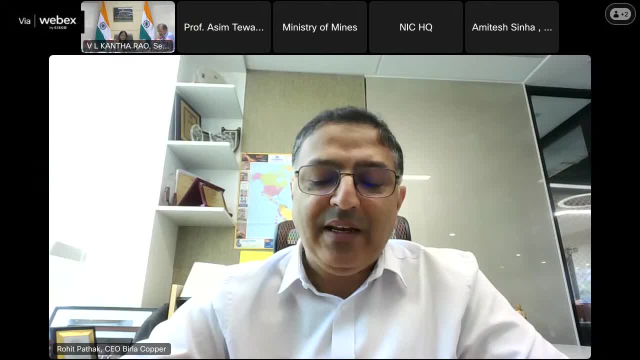 into useful form through proper recycling. So I think recycling is the fourth area where I feel there is a huge amount of opportunity. As Hindalco, we do run programs on startups from time to time on areas that we feel are important. Every year we run 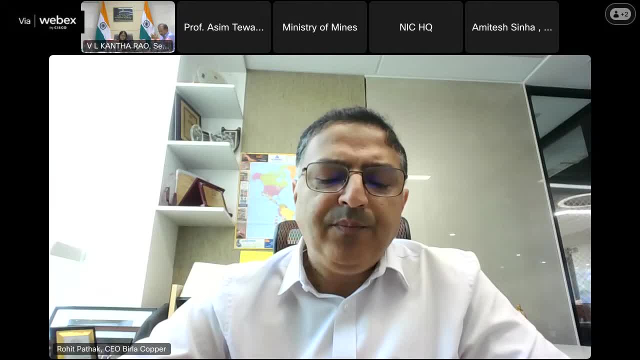 one or two programs. A lot of it is around some of the digital technologies that we will need at our plants, as well as around some new products or areas of processing technologies that we would like to work on. Feel free to reach out. That is a huge opportunity. 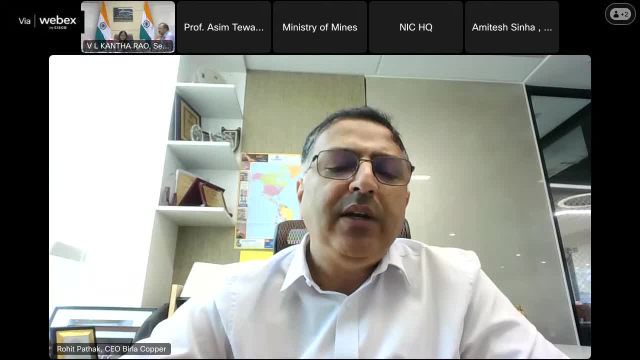 We will be very, very supportive to give an opportunity for you as startups to participate. Try some of your solutions at our plants and if it works, you can scale it up. So very happy to partner with many of you who participate. Strongly urge all of you. 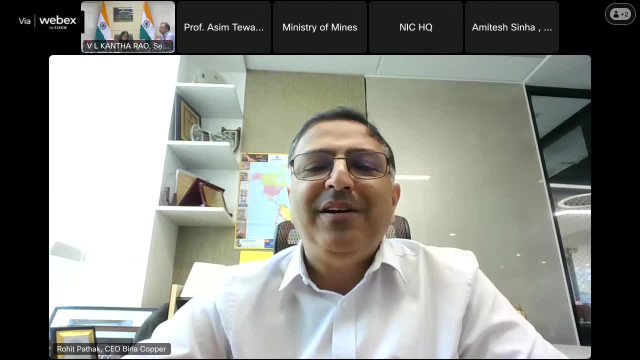 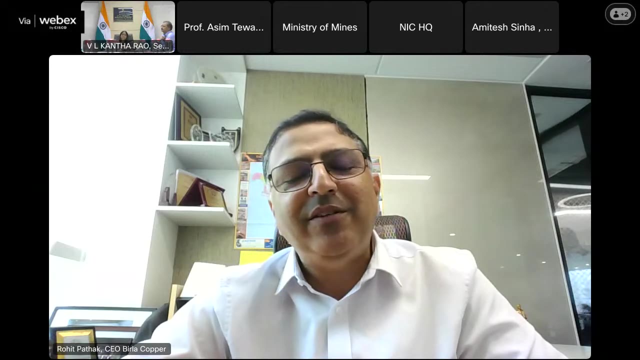 to make the best of this scheme of Prism 2 that is being launched and participate in a big number And as an industry, we will be fully supportive for all of you. Thank you so much for this opportunity and look forward to being part of this initiative. 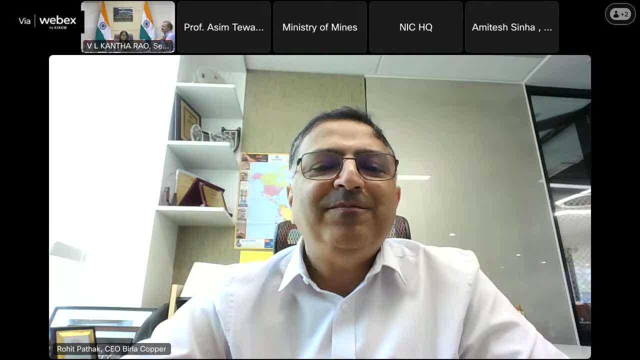 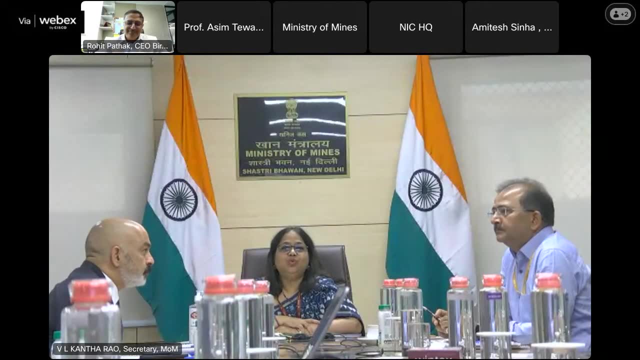 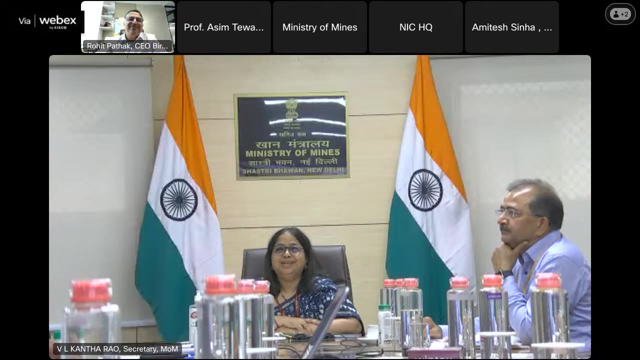 with the Ministry of Mines. Thank you, Thank you, Rohitji, for all your guidance in the matter, and we also look forward to be connected with you in future also and participate in all our summits and guide us Perfect. Thank you so much. 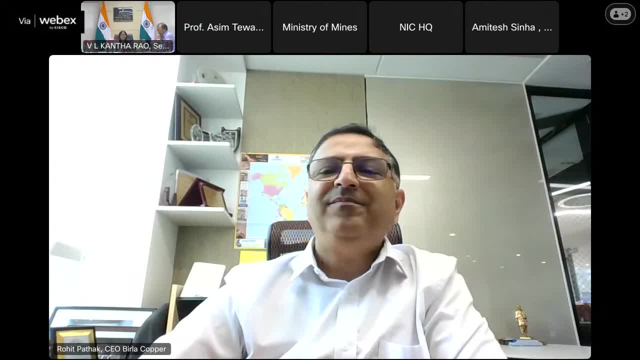 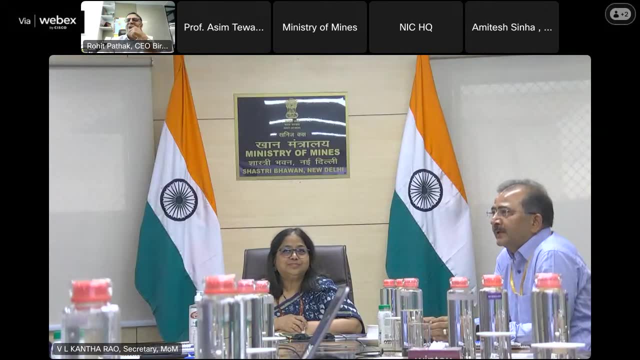 Thank you, ma'am, And before we could invite the next guest speaker, I would just urge the participants to just give your answers to the pause that we have started in the webinar itself. Questions have been already posted in the webinar and you can just. 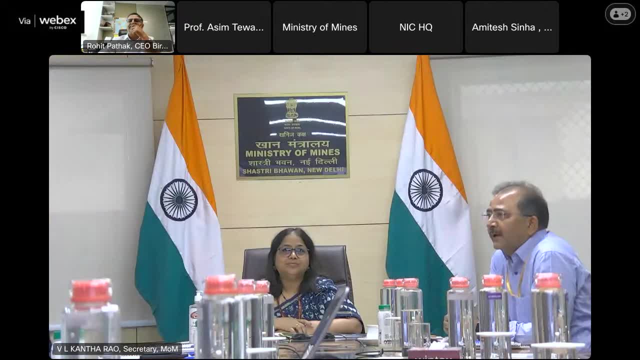 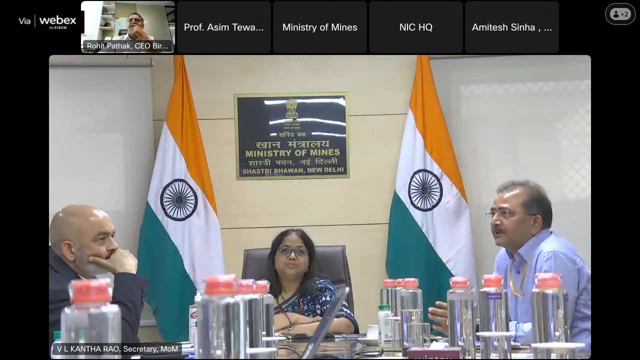 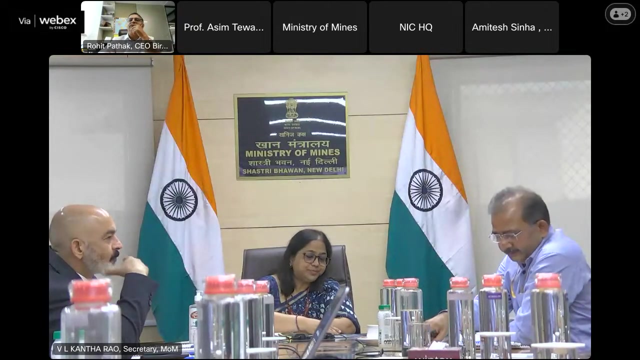 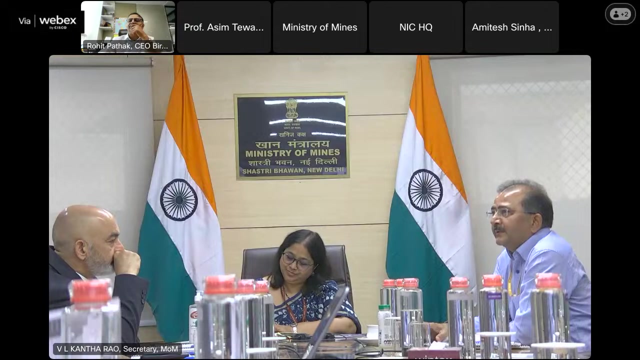 go to the chat box and answer the questions so that we can have a fair idea about our scheme and about the Government of India initiative of the startups. I will request all the participants to please participate in the webinar. Apologies, need no honor. Thank you. 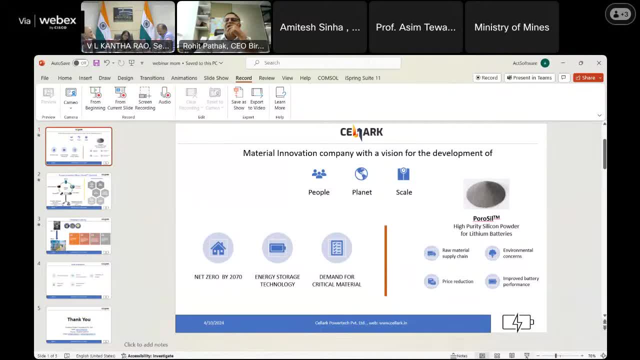 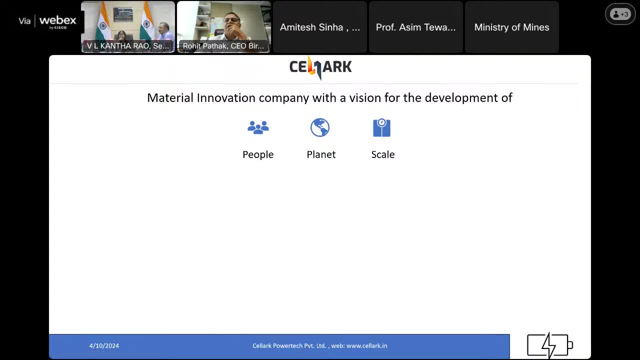 Thank you very much. Thank you and another question raised by Mahesh Mital from the Ministry of Mines. So Mr Doctor Sandeep Pandey is there from the CELARC and he will be just making a presentation about his experience about the startup scheme of the Ministry of Mines. So over to CELARC. 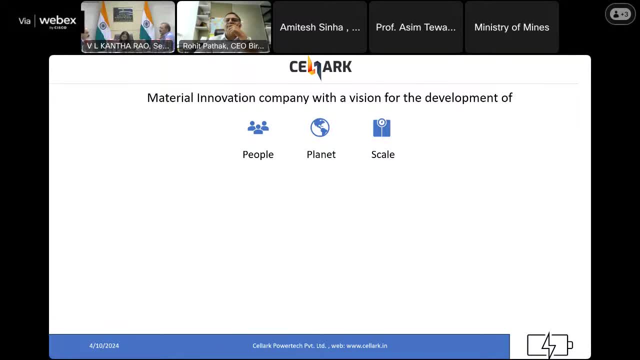 So good afternoon everyone. once again, I am Ashwini Pandey, co-founder and CEO of CELARC. CELARC is basically a material innovation company based in Bhuneshwar, Odisha, and we founded this company with a vision for the development of people, planet and scale. 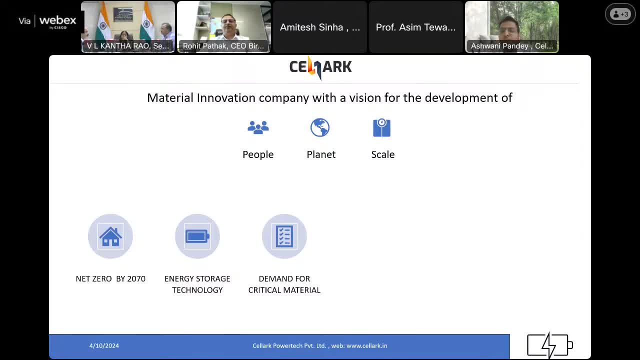 Basically at CELARC we develop materials for energy storage technology. So we develop material for cathode and anode for advanced chemistry cells and the basic idea of development of those alternative material is to reduce the dependency of the critical materials that goes inside the cell. 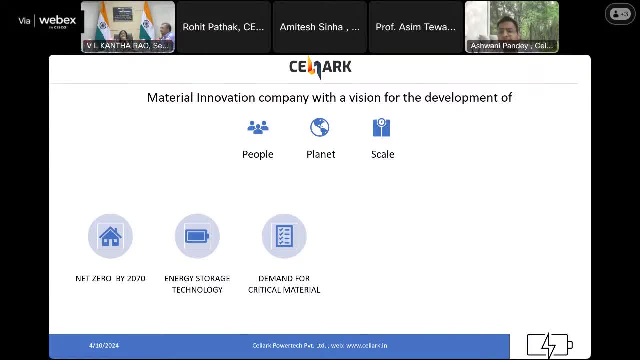 So we decided to make these energy storage technology and, in line with our vision, we have come up with our first product, that is, high purity silicon powder that we use to replace graphite in lithium ion battery. and, of course, this silicon powder brings its own advantages in terms of when we talk in terms of lithium ion battery overall performance. 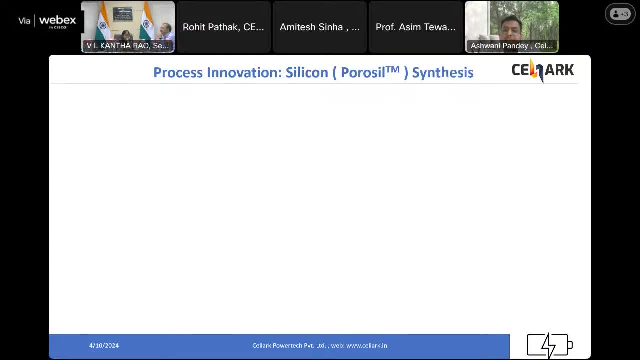 And if you look at the process of this silicon synthesis, We start from aluminum silicon ingot or aluminum silicon scrap, We do many chemical leaching process and finally we have this silicon powder And if you look at this entire process, we have many- you know- byproducts which have a huge value addition. like in our process, we generate a lot of hydrogen. 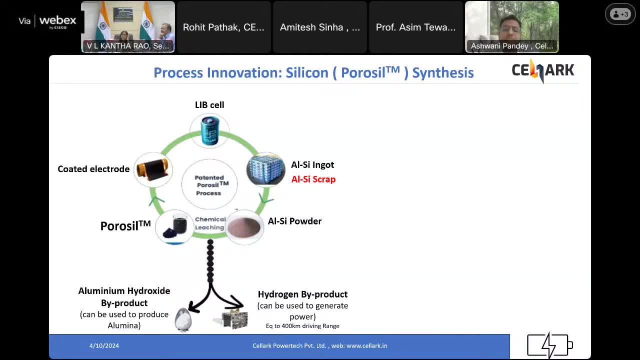 We generate aluminum hydroxide, which can be further convert into alumina. Now, since we are, we are, we are using this process in a very small scale. We are a spin off company from IIT Bhuneshwar. when we started this process, we were developing material only in the range of 5 to 10 grams. 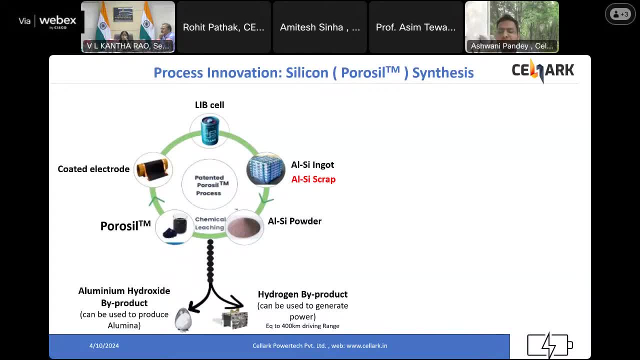 And later. right now, we are developing material in 100 to 200 grams. Now, in that small-scale scenario, it's not possible to tap all the by-products that we are producing here. So that's exactly what we are going to do with the funds that we received from Ministry of Mines. 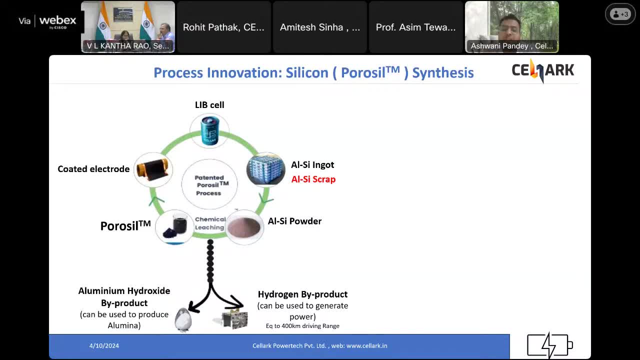 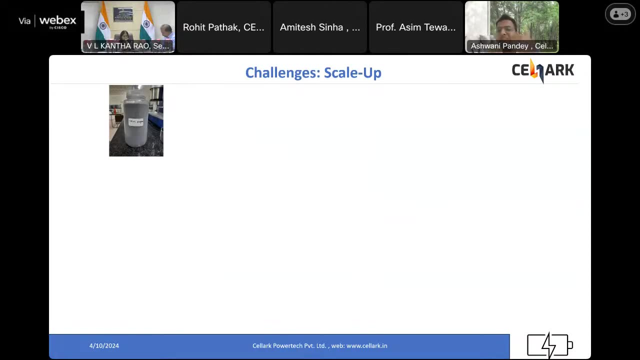 We will be scaling up the production of this high-period silicon up to 25 kg per batch with the funds we received. And for the people, for the startups like us, the major challenge right now in the startup ecosystem, if I can mention here, is in terms of the scalability. 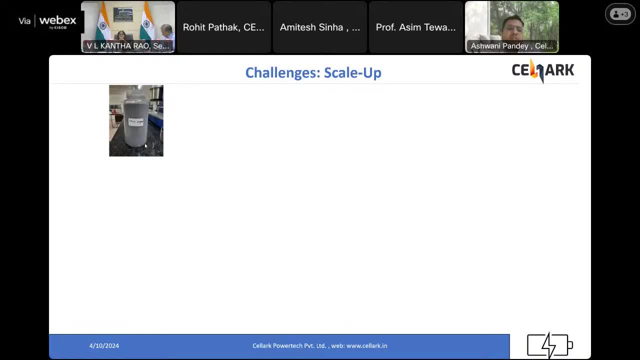 the scaling phenomena. So just I mentioned that right now we are producing 100 to 200 grams of silicon and we are at a TRL level 4.. We have already validated the POC. We are already developing the cell technology using this silicon material in collaboration with Indian Oil Corporation Limited. 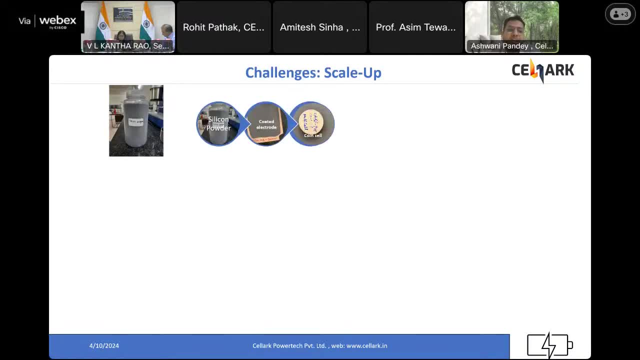 But the real challenge is that we are not able to scale up the production of silicon. So the challenge comes in terms of translating this TRL 4 to TRL 6 level where we will be starting the piloting. And the challenge right now in the startup ecosystem is- I have categorized- 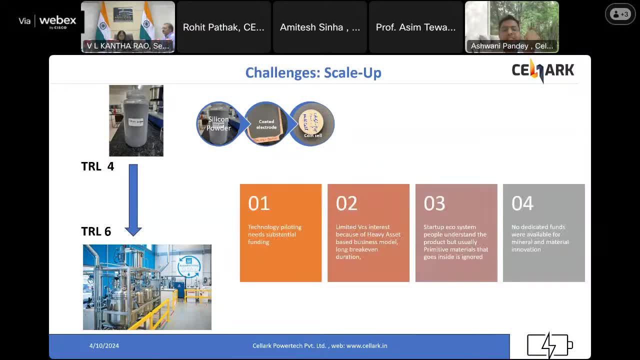 it in four categories. The first challenge is for translating TRL 4 to TRL 6,. a huge amount of funding is required for setting up the entire pilot scale setup And those fundings are not available right now in a conventional grant. So we are not able to scale up the production of silicon. 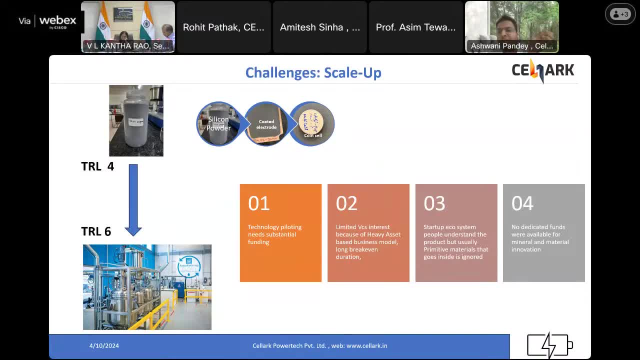 in the country. So mostly they limit up to 40 or 50 lakhs of the range. The second challenge- that already mentioned by Mr Amitesh G- that very limited VCs are there who are interested in these kind of business, who are based on a very heavy asset business model as well as long break-even. 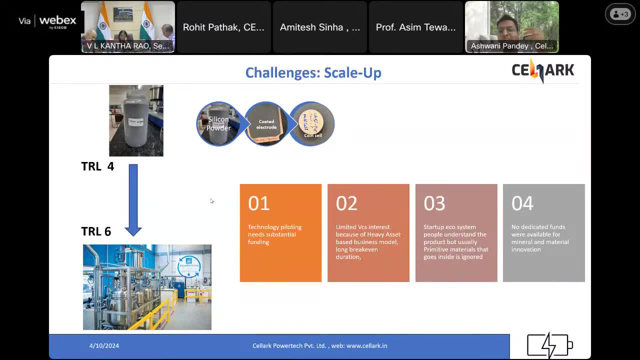 duration is there, So the VCs are not interested to fund these kind of innovation. So that's another challenge. And the third challenge that I have observed. maybe it's not applicable to its entirety, but in the startup ecosystem people understand the end. 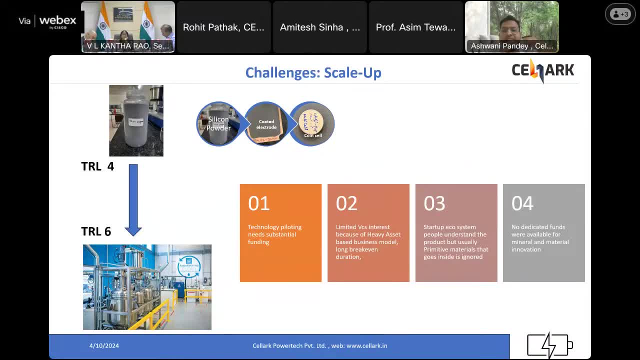 product. So in my case they understand the battery pack, they understand the electric vacuum, they understand the charging stations, But generally they ignore the primitive material that comes for that is used to make those consumer products. So that is generally ignored. 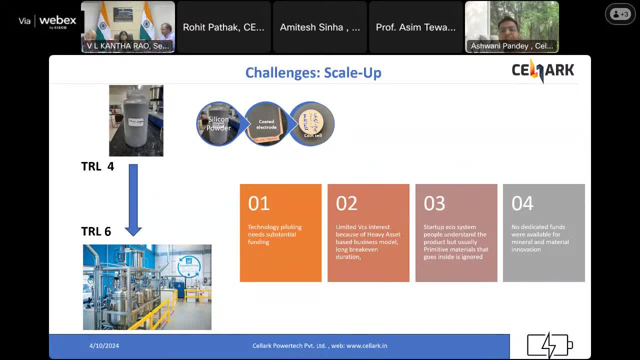 in this segment. And the fourth and most important part challenge is there is there is no availability of dedicated funds for innovation. So that's another challenge that I have observed. And the third challenge that I have observed is there is no availability of dedicated funds for innovation. 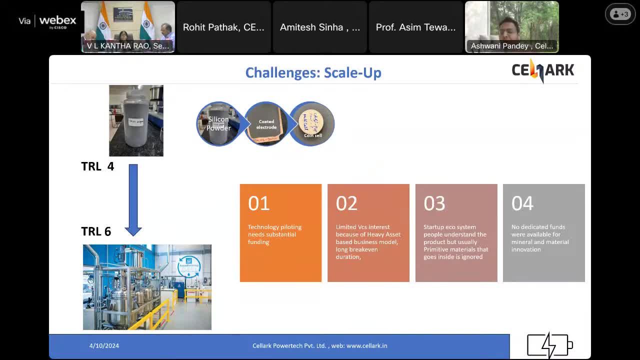 that is happening in material and mineral innovation segment And I'm really happy and I'm really grateful to Ministry of Mines that they have observed these challenges and they have worked on addressing these challenges in form of curating this S&T Prism scheme for startup and MSMEs. 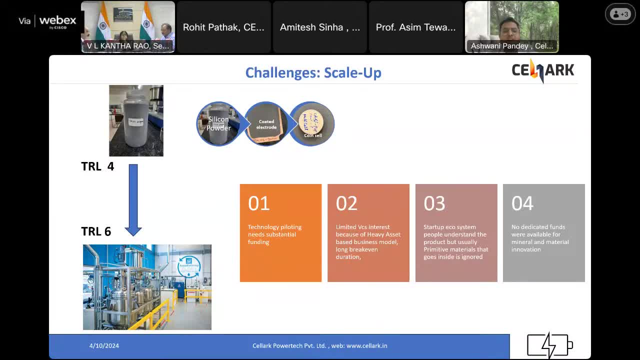 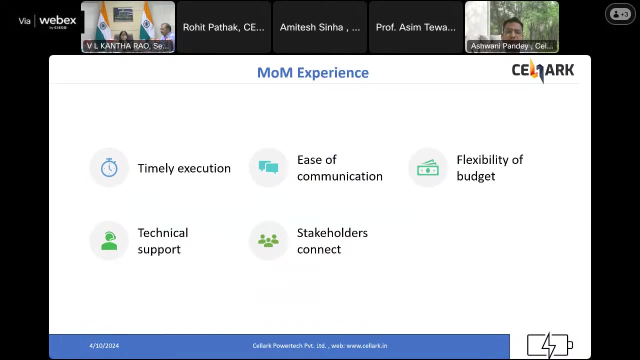 I would like to summarize my experience so far. For the last four months I'm involved in this Prism 1.0 journey And I would like to summarize this entire experience in five core segments. Like the first segment is the timely execution. 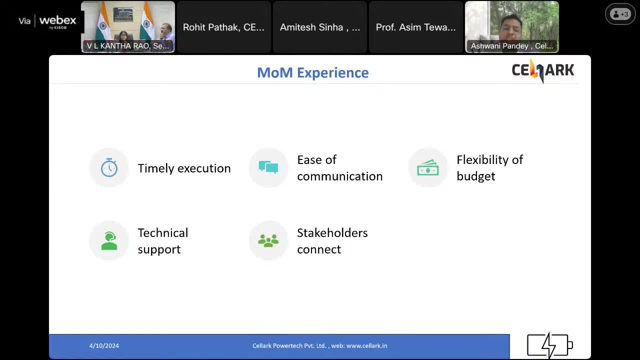 and it's really commendable job done by the entire MOM team, The entire process of filing the application and the sort listing the results and finally signing the MOU with the MOM. it hardly took two and a half months, So it's really rare in any government grant scheme And I'm really seeing. 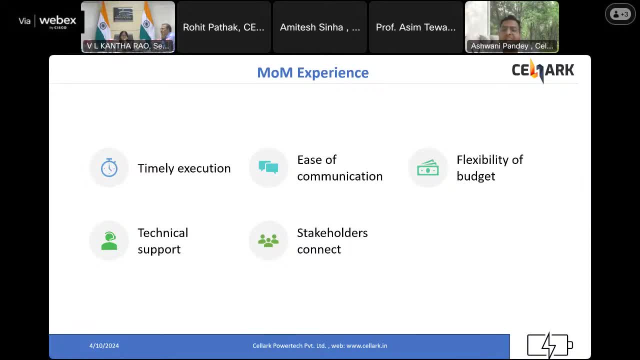 this kind of speed, first time in the entire startup ecosystem. The second thing I most like about this scheme is ease of communication. So the officials who are managing this scheme. they are easily approachable. You can communicate with them over WhatsApp, you can communicate with them over phone, email, and you can expect the reply within one or two. 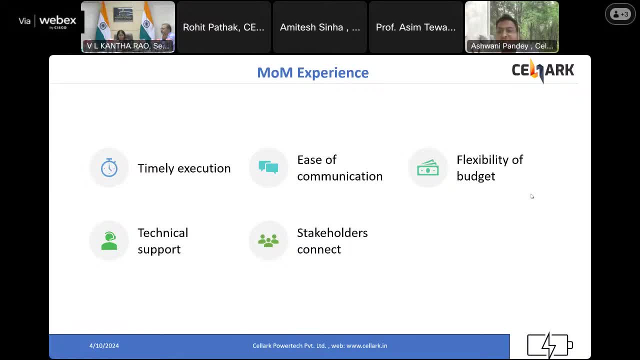 hours, So they are really approachable. That is really missing in some other grant scheme. Dr Prakash Rathore MD. And the third and most important advantage of this scheme is flexibility of budget. So when we were applying, 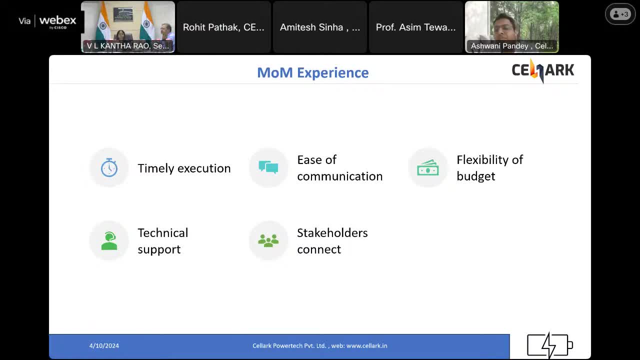 for this grant. we were really skeptic whether we will get the grant or not because our asking amount was a little bit higher than the 1.5 crore rupees. And this grant, as Agnihotris are already told, that grant is designed for a maximum cap of 50 crore And in some cases it can be. 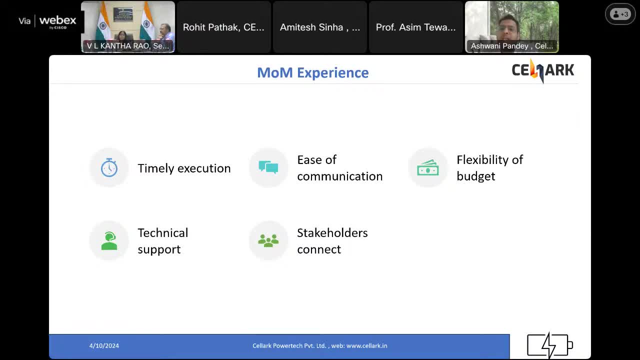 given up to 2 crore rupees. So I'm really happy that Agnihotris team did the due diligence. It realized the importance of the technology scale-up and they granted the money depending upon the requirement of a particular startup. And the fourth and most important part I observed is in terms of technical support. 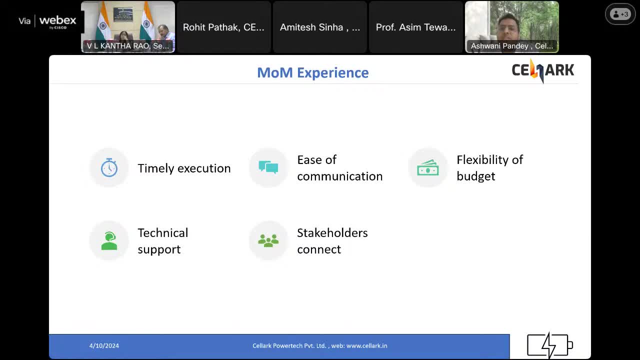 Being a startup company, we have certain lack of expertise for scaling of these technologies And since JNAR DDC is nodal agency for this MOM scheme, they have a very good lab characterization facility to test your materials. They have a very good pool of expert. 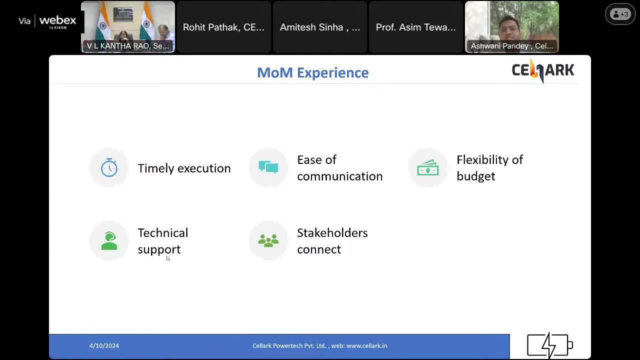 members who can help you to bring the expertise for scaling of the technology and you can further bring down the overall cost of scaling up your product or innovation. So for the last four months- just recently in the last one and two months- I could observe that technical support. that I can obtain from JNAR DDC team. And, of course, the fifth part that is already discussed is the going-to-JR G&A and G&A m��d. You can do this from the start-up and keep it that way for the entire year. You can do the entire year. 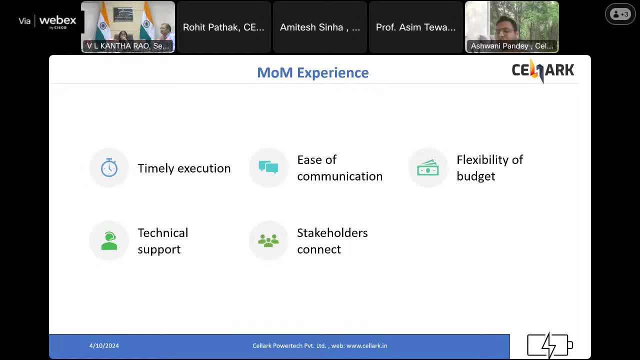 And, of course, the fifth part that is already mentioned by Agnihotri Sargi, that being a startup. in this entire MOM scenario, we have a great opportunity of networking because all the stakeholders are well-connected with Ministry of Mines, whether they are your raw material supplier, whether they are your potential customers. 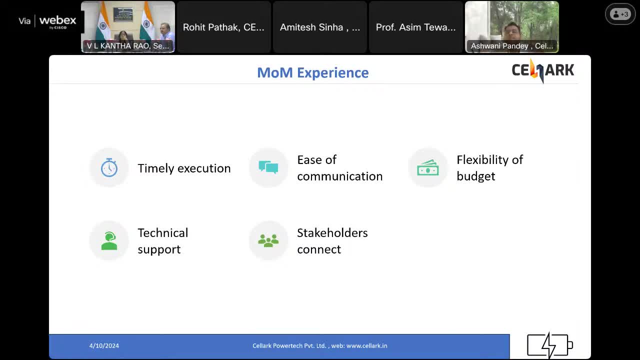 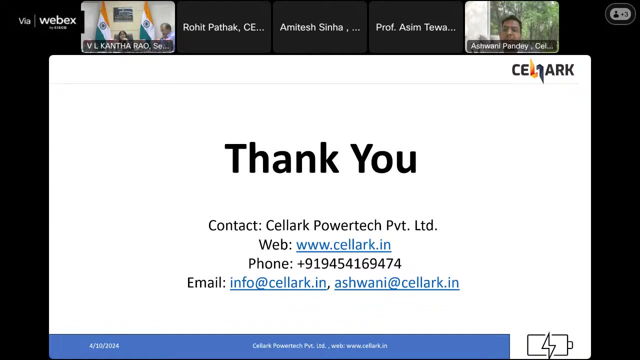 So those networks can be explored a lot being inside this scheme. So these are the advantages we generally get being in this project scheme. So I would like to conclude by this and I'm really thankful to entire MOM team for giving me opportunity and actually trusting our innovation and supporting for the scale-up of this innovation. 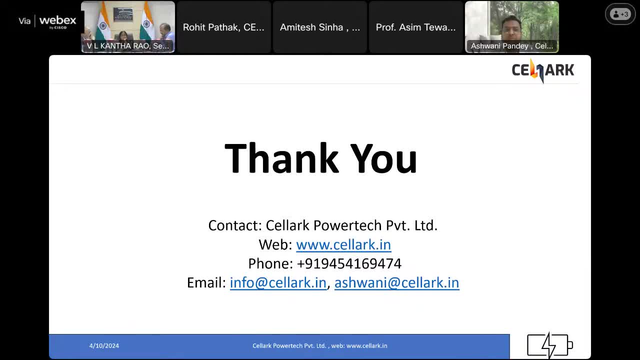 Thanks a lot. Thank you, Ashwiniji, for sharing your experience about our Ministry of Mines startup scheme And I hope, if you…. Thank you, Ashwiniji, for your encouraging word. others will be just motivated to participate in our scheme itself during this phase two program. 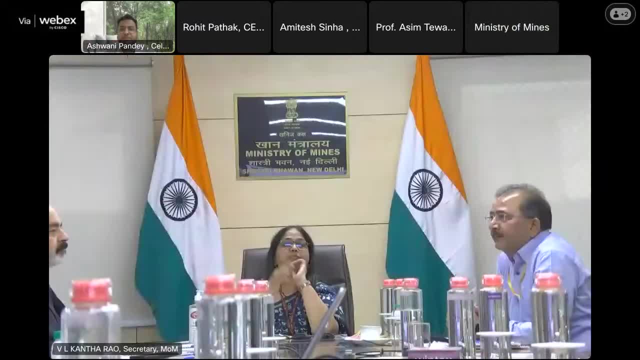 So thank you so much, And now I'll request the Caliche team- that's another startup that has been funded by the Ministry of Mines- to share their experience. And I'll just welcome Matthewji and just request you to just share your experience. 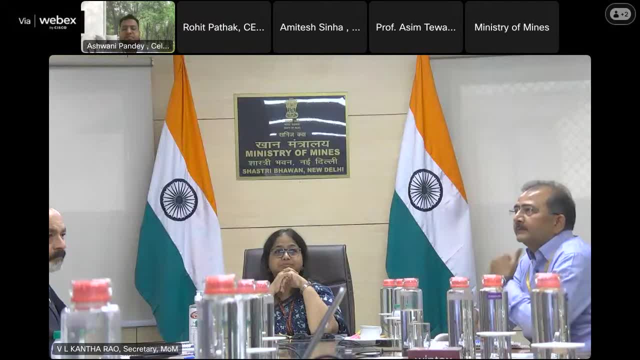 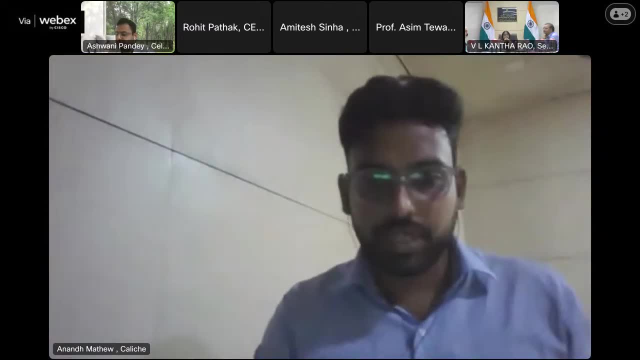 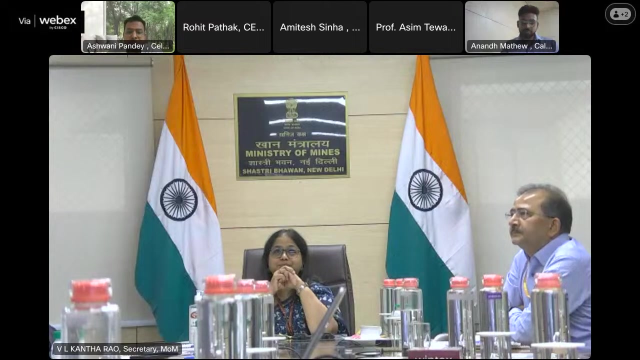 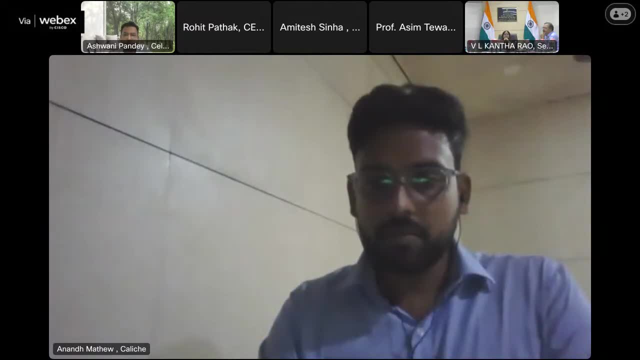 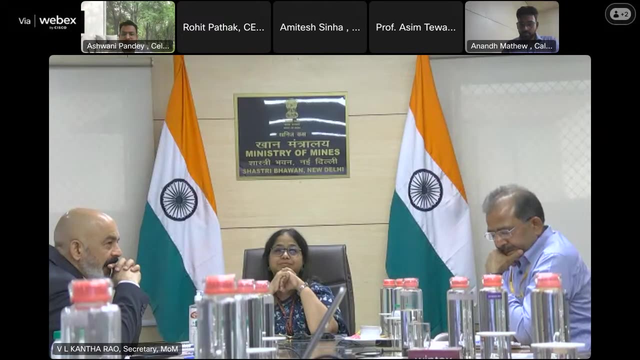 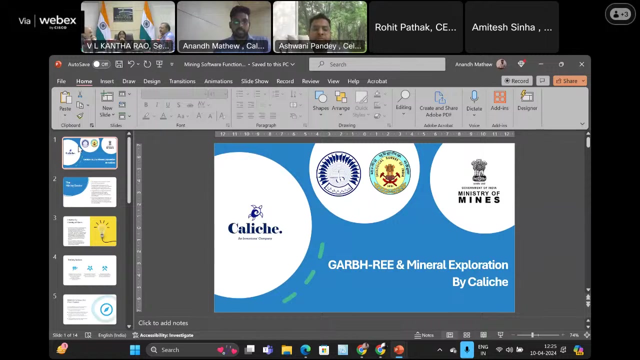 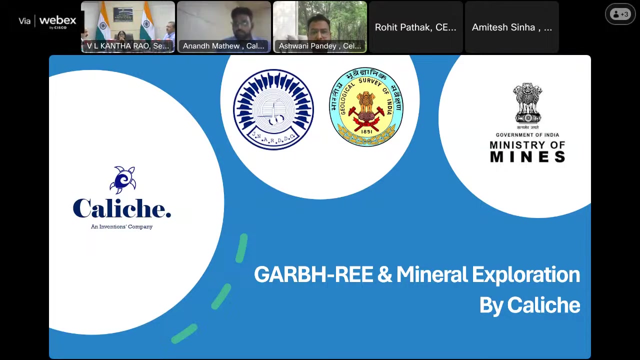 No, No, No, no, Only your visible. I hope it is visible. Yes, it is. Yeah, Let it close screen. yes, so, uh, first of all, uh, before starting, i would like to thank the entire team of prism process uh for giving us an opportunity and also to uh give given our platform to 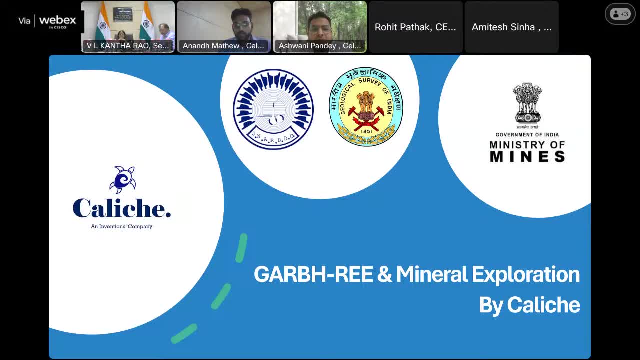 share our experience about how we entered into this particular industry and how was our experience so? uh, we are a northeastern startup. we started back in 2018, so currently in mining and mineral sector, what we are doing is we are developing uh software for re-exploration. 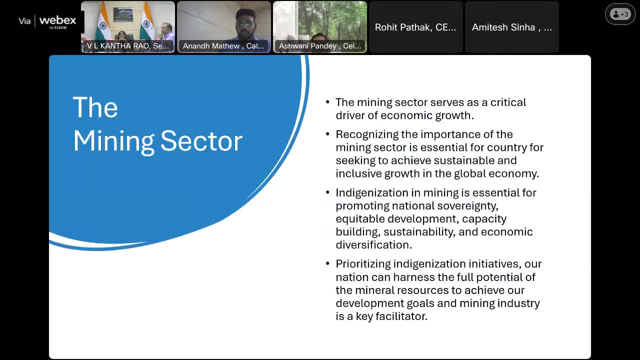 so, uh, in the mining sector, uh, we've been working in oil and gas sector when we started, so see, oil and gas sector and mining sector has a lot of similarities when in terms of supporting the economy. so we are a northeastern startup, we started back in 2018, so currently in mining and 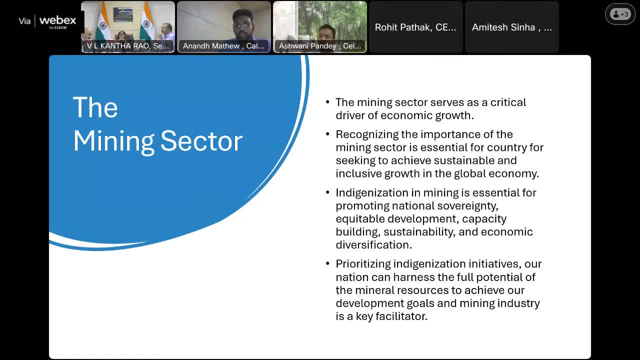 the economy of the country. so we were waiting for an opportunity. uh, what if we can do something in mining sector as well? so that was one of the key factors. so there were obvious reasons why mining has as very important role in the current economic situations for our global development goals. so 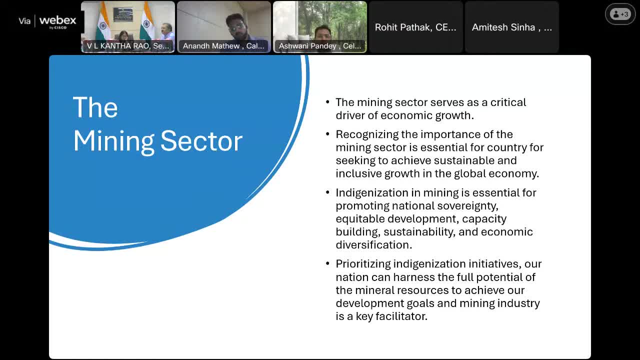 we've been finding out. what are the areas where we can actually work and on what platforms you should be reaching out. what are the? what are the other sectors we should be considering in development or developing technology technologies for, since we were a very R&D based technology from beginning? 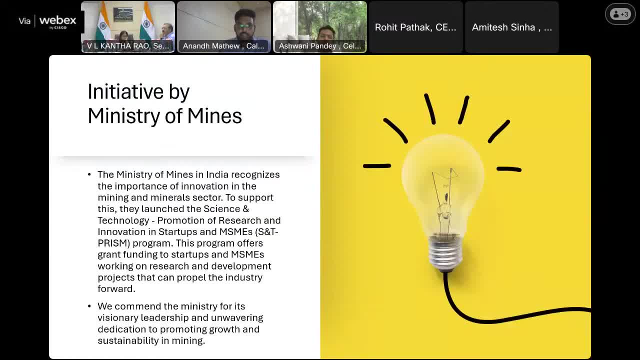 and that is the time we came across uh, this, uh prism initiative by Ministry of Mines. so from the beginning itself, we were very, uh positive about the, the approach that Ministry of Mines had, because, for the first time, such a very, very detailed overview of how a startup 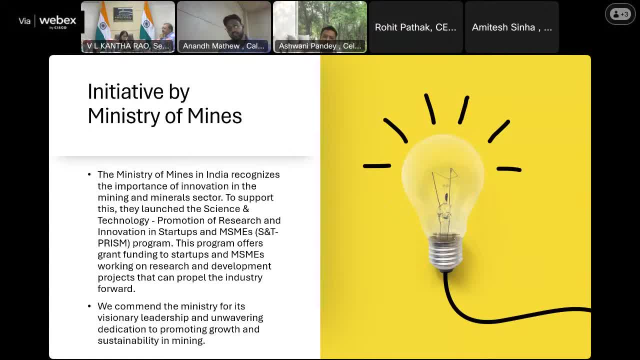 needs to be supported, because I was a part of the total process and when it started, during the policy making itself. so it was very instrumental, I would say, and very thoughtful decision was made and whatever uh points, or each and every that has been drafted, that has been considered after taking a lot of inputs from the industry, partners and even 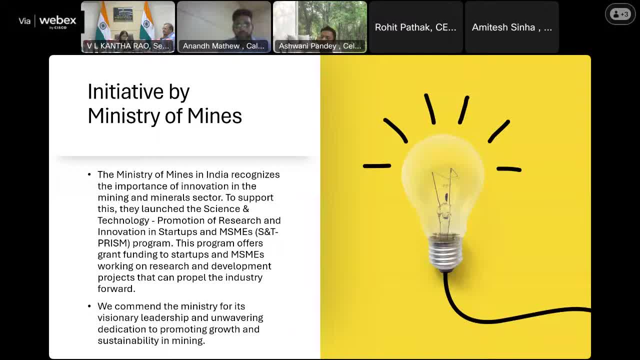 the startup. they've taken the inputs from the startups also because Ministry of Mines have requested, uh, their stakeholders also to give your inputs on what needs to be added, what needs to be removed from the policy as well. so, uh, we would like to comment on the Ministry's visionary leadership. 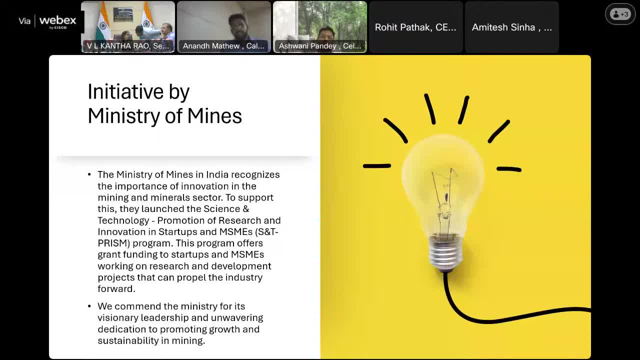 over here and the dedication to promote, uh that sustainability, growth in mining sector in deep state and supporting startups in solving problems in the mining sector- uh, a few key factors I would to mention, uh for others who have joined here, uh about this program. so, uh, it is. it is actually 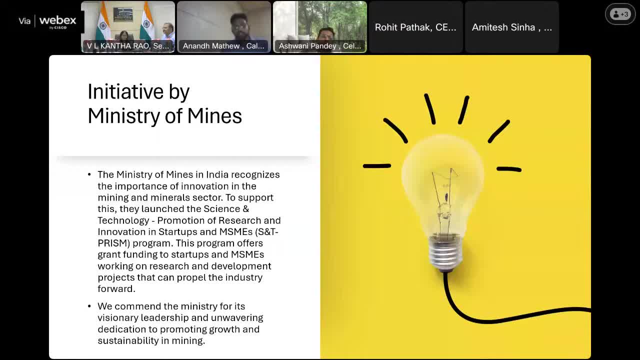 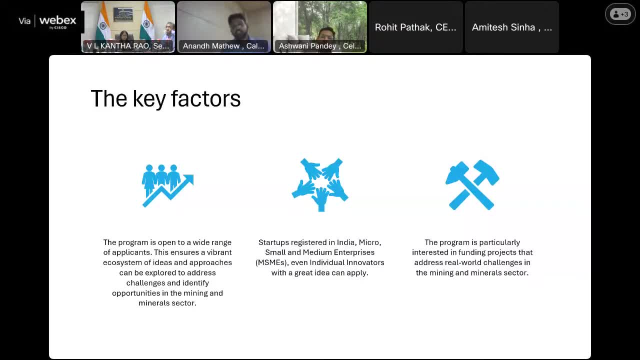 open for a wide range of applicants. so it is not that it is limited for somebody, it is open for wide range of applicants. and, of course, when it comes to applicants, the wide range of challenges are also addressed. so the challenges that we can actually produce, develop solutions for that number. 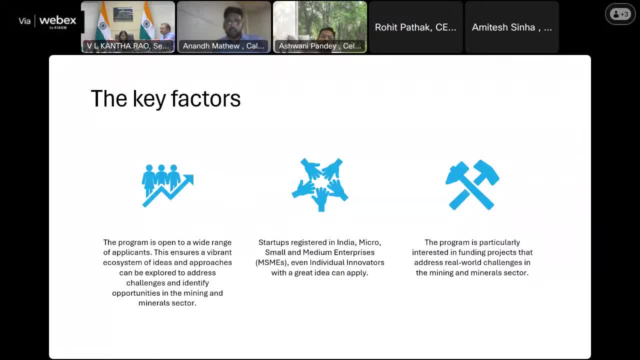 is also very high. so that means there is a wide array of places where you can actually uh, figure out where your technology or your idea will fit it, and they have been an opportunity for startups- msmes- also to be a part of this, and if you don't have any of these, you can actually if an individual 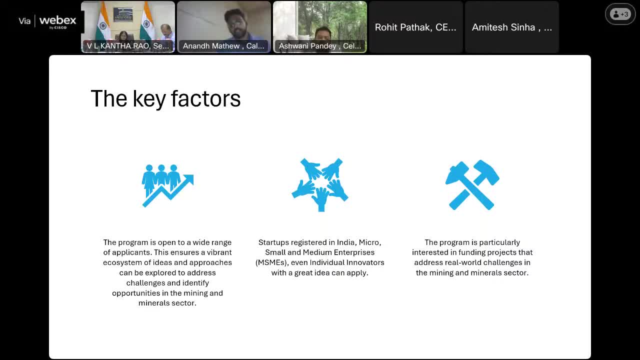 innovator and you have an idea which you think that will fit in the trust areas you can actually apply as an individual investor as well, innovator as well. so, uh, now this program, what i feel personally very uh, what i feel very personally liking about it, because one thing: for an idea to uh materialize: 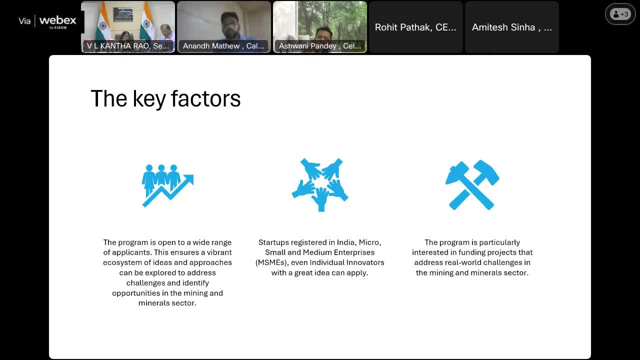 so of course, you do a lot of r d in it, that's true, but when it comes to scaling it up to a state where the clients can use it, they, they need a lot of funding, so that funding is required. so, coming to my uh fellow mate, uh from salah, he mentioned about it that the startup doesn't 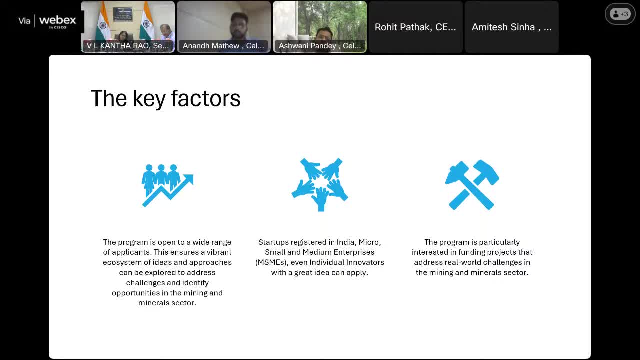 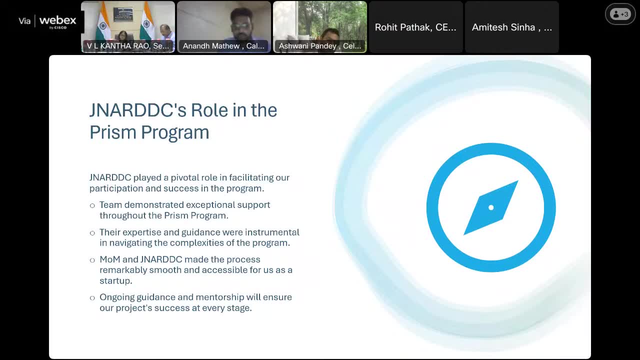 understand this part. so ministry of mines have been very instrumental in understanding this part. now i would like to add a few point about dna���c as well, avoiding uh them if this would have been not to be a successful. so the team played a very pivotal role in supporting uh this initiative, even though it was- what do you say? it was very new. 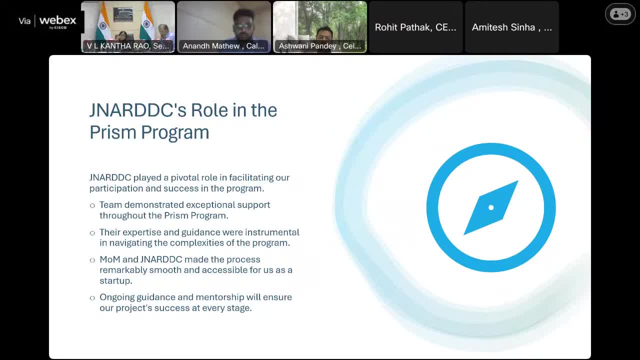 uh in the, in the industry, but they've been very supportive in the end-to-end processes. so, uh, starting from the product, uh, the proposal, drafting submissions in on um, in-person presentations, documentation processes, onboarding processes, whatever you name everything, whatever includes in this process. it was quite easy and 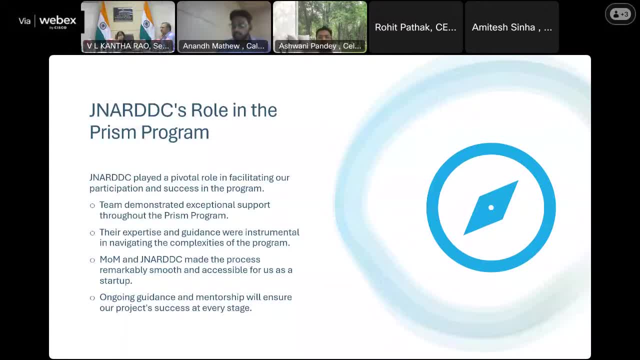 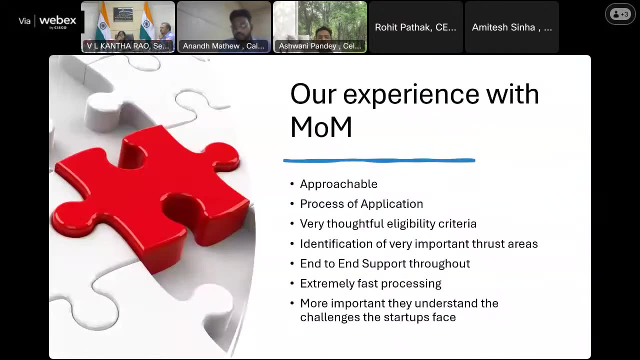 smooth in in the total phase and i would like to thank the analysis for this uh support that i've offered. so, uh, briefly about our experience with mom. uh, first of all, we've worked with another other industries as well, but ministry of mines is very approachable from top to every level. 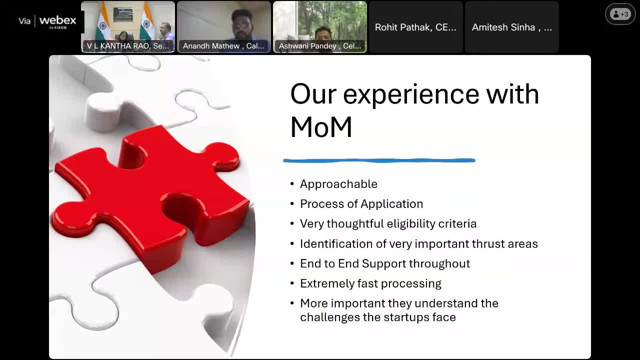 the process of application was very, very easy to go ahead with. uh, with very minimal understanding about uh the process- background process, you could actually anybody can put that application. the eligibility criteria is kept very thoughtful. that is very commendable. uh, the thrust areas identification was done on a thoughtful manner to like for the project terms that. 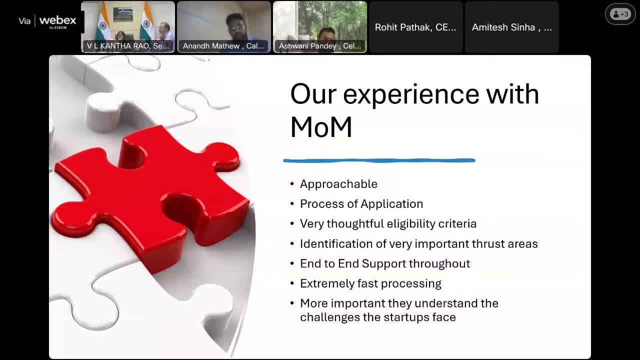 they have mentioned, the thrust areas falls in goes a very right fit, and the current ecosystem that we have, uh, in terms of development for the country, uh, that includes- they have included- everything, uh, the end-to-end support that they have given from the ministry. that was phenomenal. 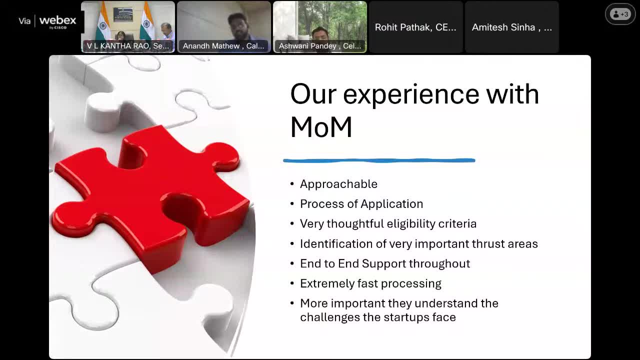 and uh extremely fast processing time. this is, this is an achievement, i would say uh, the processing time from the day the proposal was initiated, the proposal was submitted, and the time that you got done was uh approved later. uh, more important, that the ministry of mines really took care of the. 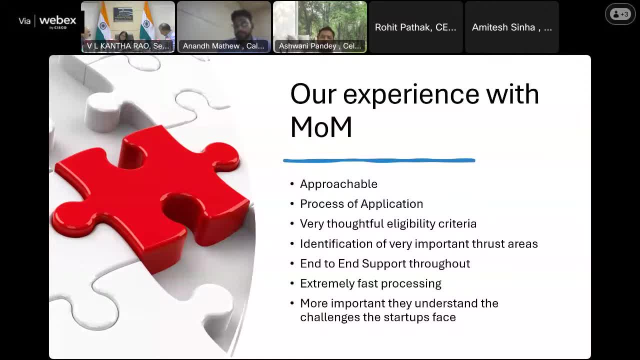 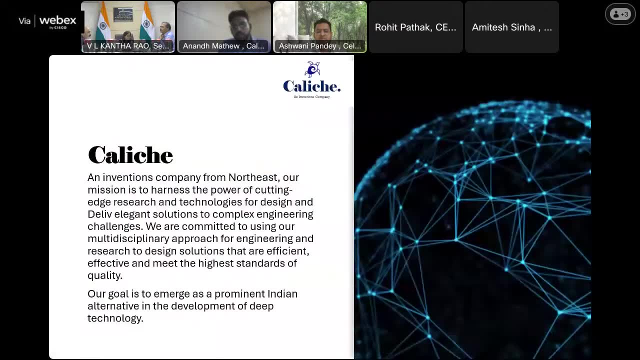 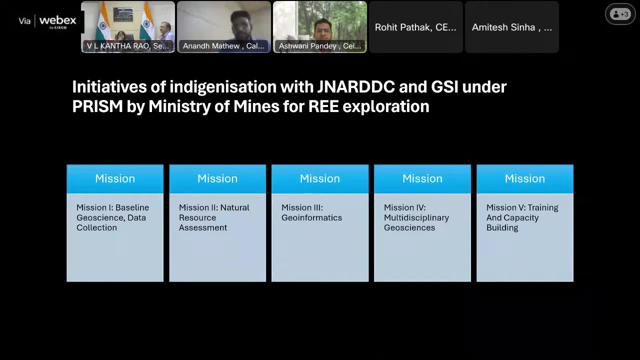 challenges that every startup is facing. for us, it was a very great support that they have offered. so, uh, going to our technology, what we are doing is uh. we are in collaboration with jnr, ddc and gsi, we are developing uh re exploration software for government of our india. so, since we do not have uh, 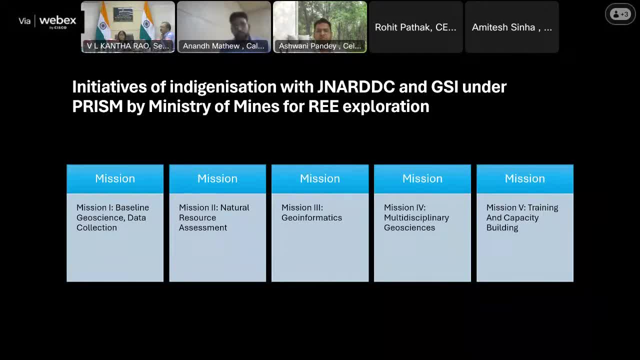 we, we are developing uh indigenous software so that it can be used in our uh for for our country. so the ministry of mines have identified a lot of critical minerals so this will be a game changer in uh in that process for ad, for achieving the codes. so we are categorized, entered into many 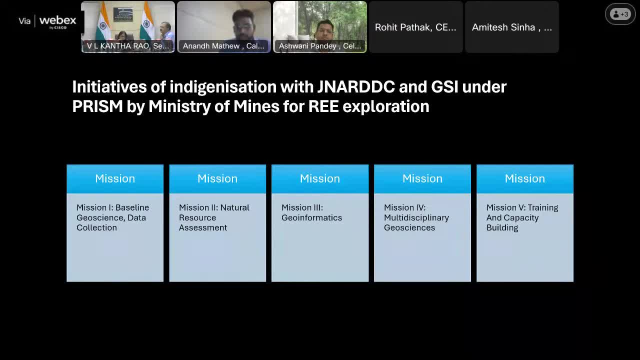 subdivisions wherein uh baseline indigenous data collection will be done so that data is already available. industry of mines has made it uh public so that can work on it uh, so we will be doing a lot of data processing- part of it- and the software will be built on that data process part. 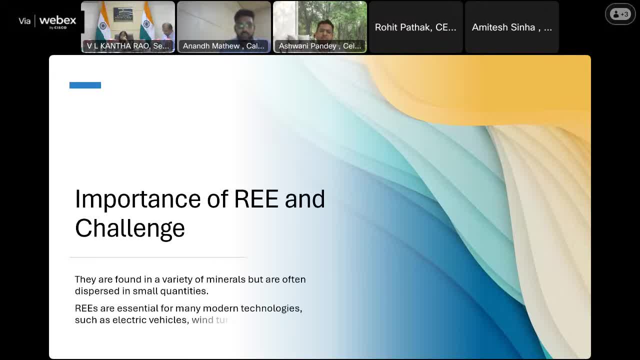 so, uh, why we wanted to do in re is because, uh, we identified that re will play a very important role uh in economic development of the country and being at the right place at the right time. such ways uh give a lot of mileage for the- i mean the companies who will be working on this. so, for 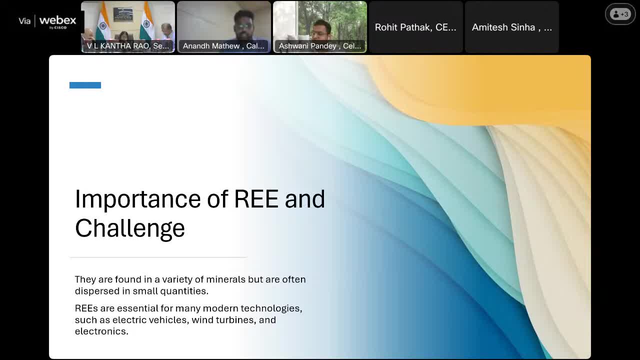 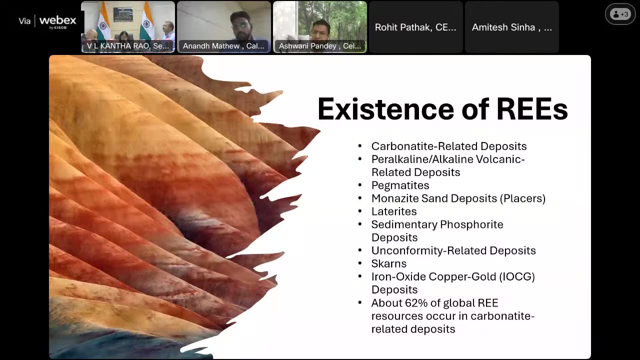 example, the stakeholders will be working on re production or extraction, but for them it will be a very, very good, uh help that we can actually offer. that's the reason we wanted to work on re one dot. have you ever started your own? so, uh, we call our the software as garb. so what we wanted 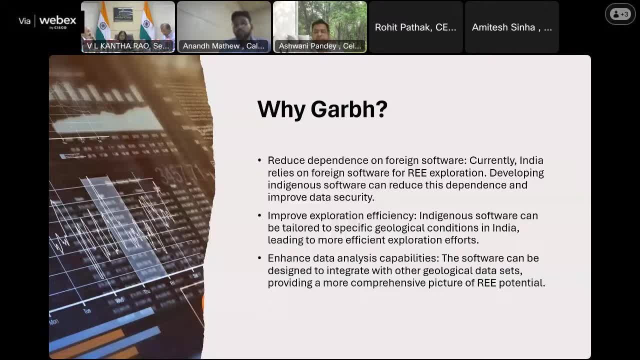 to achieve is we wanted to, uh, reduce the dependence on foreign software, improve expression efficiency and enhance the use of data analysis capacity that we have. so we have the data, we have the access to the data, but what we do not have is that we have the gap that we have between 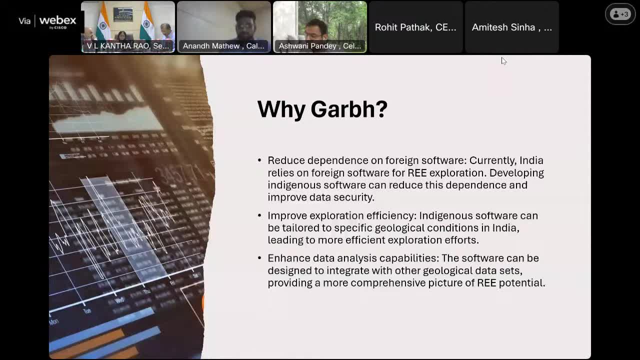 details. what we are trying to do is build the gap between this. this is about us, uh. we started as a oil and gas startup, we've extensively worked in r d sector and this is our first initiative in mining sector, and we are very, very uh happy about. 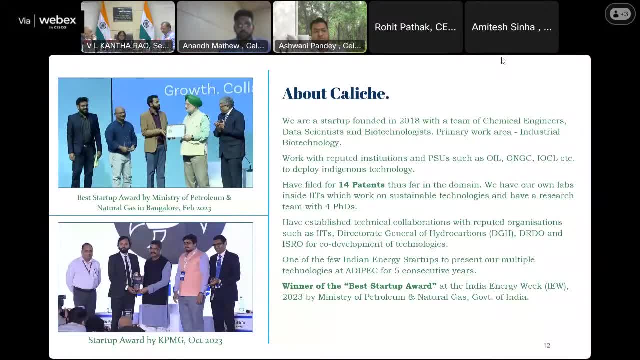 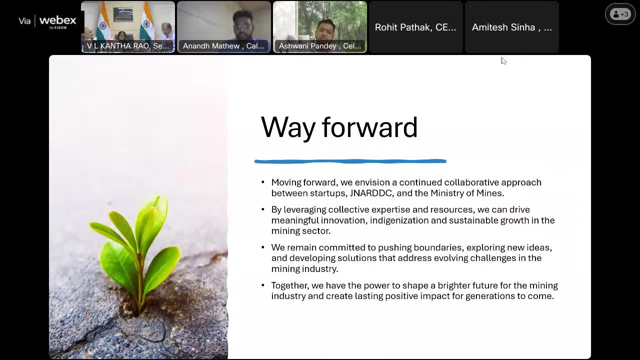 this opportunity and we believe that we will be able to foster more innovation in the sector and moving forward. uh in collaboration with all the entities involved, that is, jna, radc and ministry of mine, we will be developing this technology and we'll be uh giving it to the clients to use so that 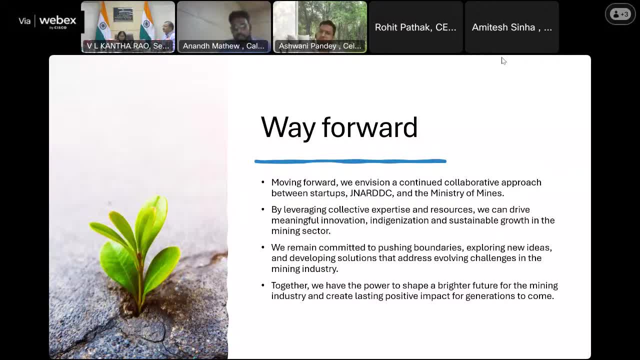 we have an indian software to work on. uh, the collective expertise will be always helpful. uh, in innovation, one thing: uh, we believe in that mining industry has the capacity to lead uh the innovation in the sector. we- this is just a start- and with our, with everybody's- 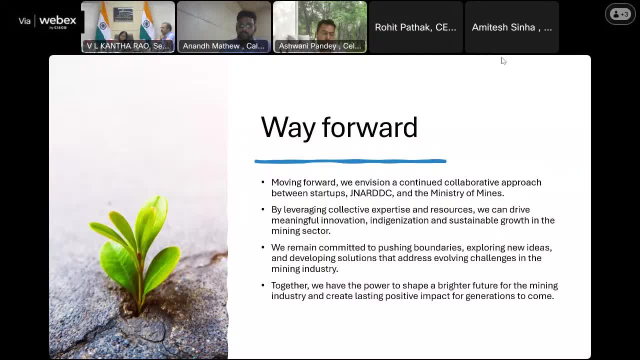 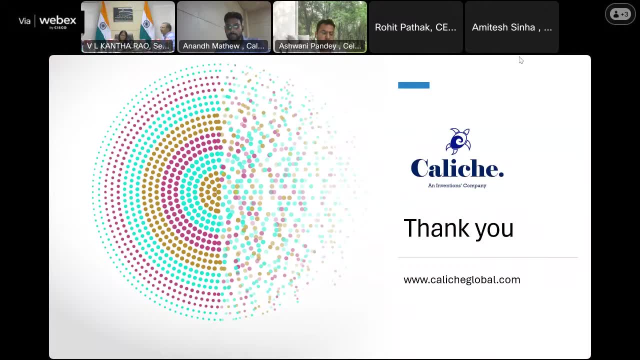 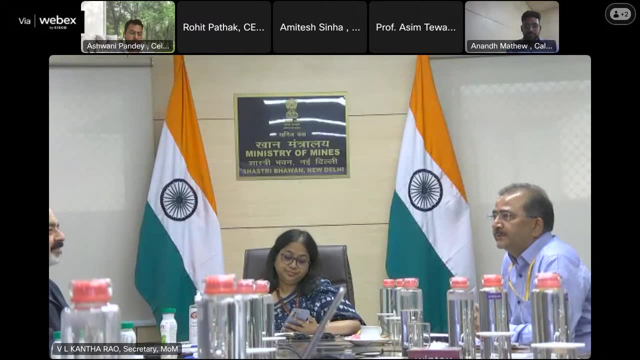 support. we will be achieving it uh in times to come. thank you so much, uh. thank you, matthew. i think your encouraging words would also motivate the others to participate in our snt business scheme and i assure all the participants that, in case you submit your proposal, you won't face any problem at the ministry or at the jna ddc itself. jana ddc. 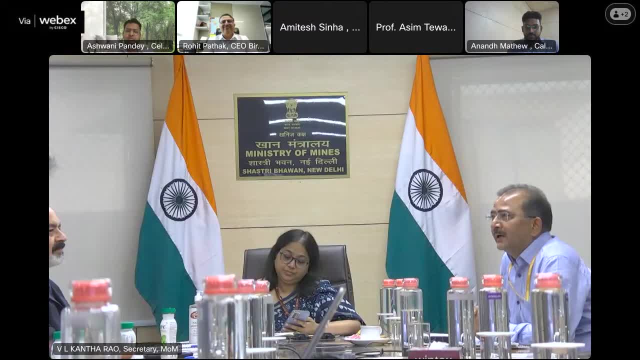 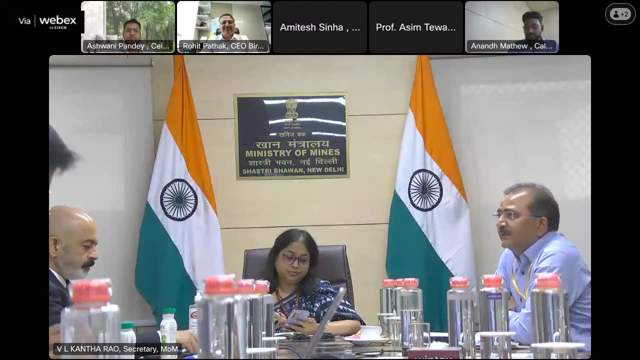 director is here and he is all supporting very positive and doing wonder in the field of not only the r? d but also in the startups nowadays also. so in case if you have any problem in just drafting your proposal or just having any idea proposal also, you can just contact him also or you can contact the ministry also and 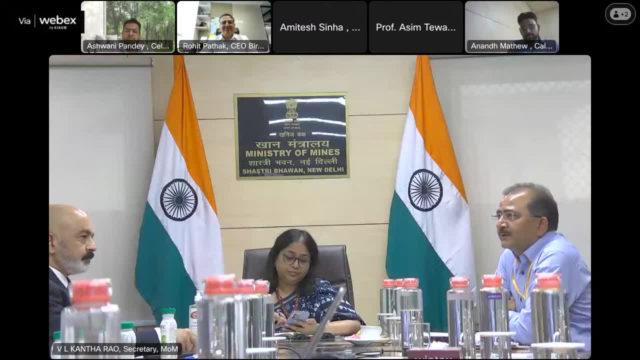 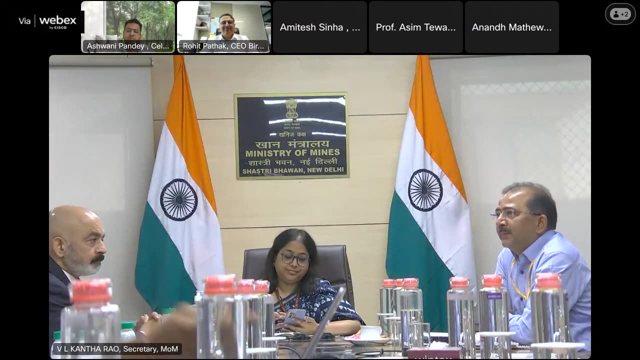 we are all here to help you and support you to participate in our scheme. so with these, what i know, professor asim tiwari from iit mumbai to give his presentation also address the participants over to professor asim tiwari from iit mumbai. 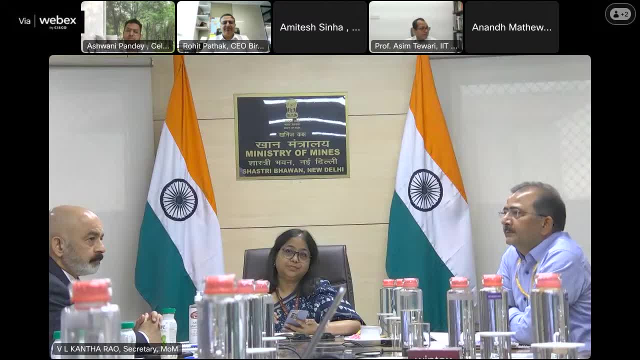 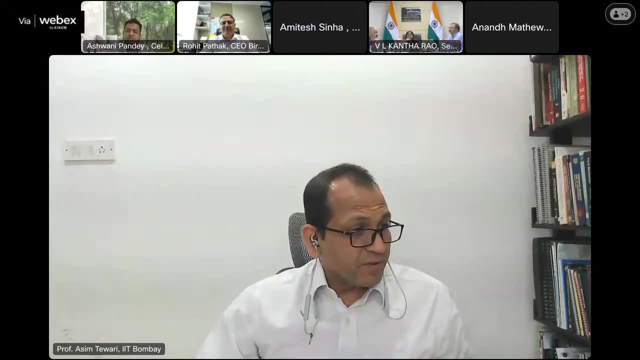 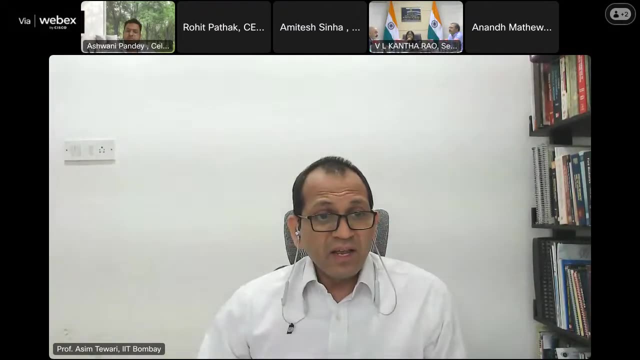 thank you very much. um, i'll just share my screen. what i have put is that i have put together the. the work which we are doing in the area of artificial intelligence and ai is transforming the world in a manner which we cannot even imagine. so i'm not going to go into a lot of details. i'm 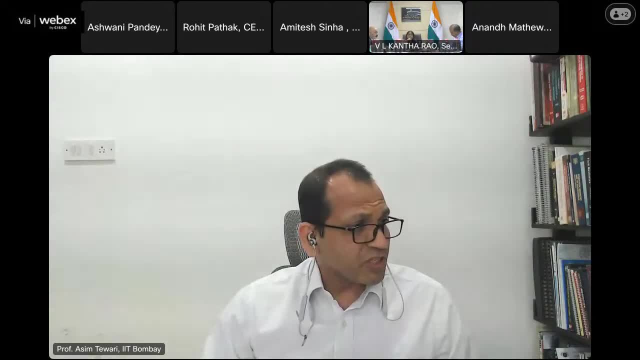 also associated with a startup. let me just share my screen. i'm also- state uh- associated with a startup, so i'm not going to go into a lot of details. i'm also associated with a startup and i will be talking a little bit about the work which is being done by them. but due to proprietary 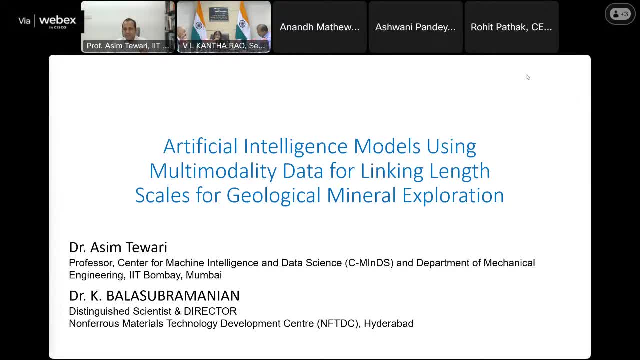 nature, i won't be able to share all the details. i'll give a high level overview of what is happening. so this is now talking about the elephant in the room. no matter where you go, what you do, ai is there. ai is with us in our communication. there are ais which are doing live translations of what we are. 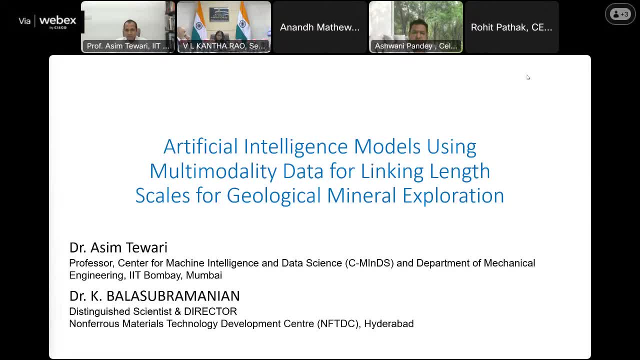 speaking, transcripting that data, figuring out keywords and so on and so forth. so and every aspect of security data and inference is being looked at by ai. so this is about artificial intelligence models using multi-modality data for linking lens scale for geological mineral exploration. i would like to specifically thank dr bala. 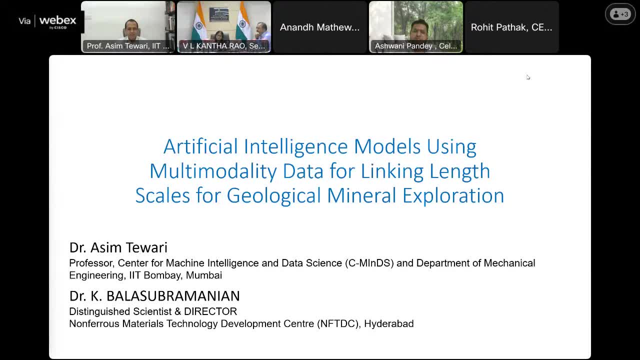 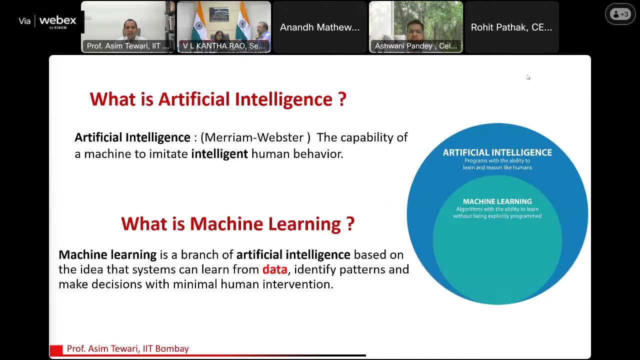 subramaniam, director uh, distinguished scientist and director of nftdc, because he and myself have been very closely working on activities uh on mining and aspects associated with engineering and engineering and geological exploration, and the general liberation and geological exploration is one of them. machine learning has been something which has been more of. 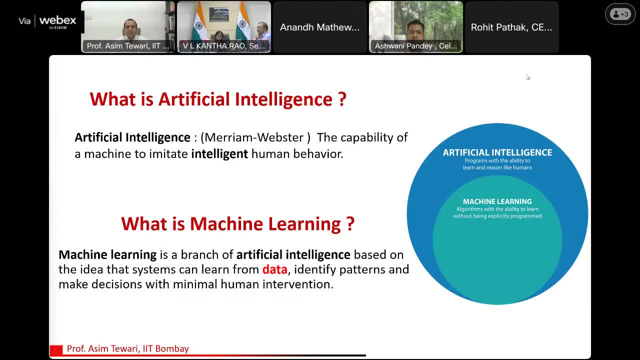 a recent phenomena as compared to ai, artificial intelligence- the term itself was coined more than 70 years back, but it was machine learning which kind of captured the imagination of people way back in about uh 90s, when a lot of advanced machine learning techniques came, and they were, they were. 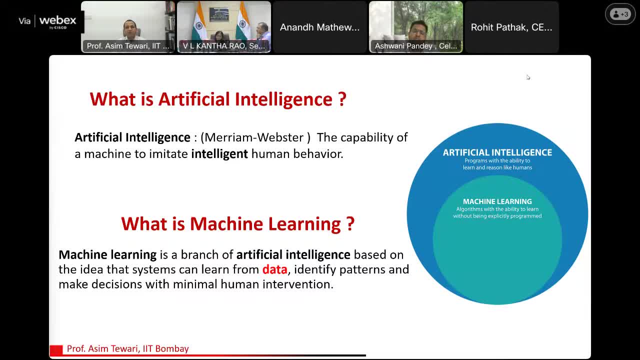 thought to become very advanced. unfortunately, 활용 Speaking ж, We rather use a lots of natural knowledge因为 dellsarean do anything, and these are some of the most common techniques which we were having. no, these techniques could do anything. and these are some of the most common techniques which. 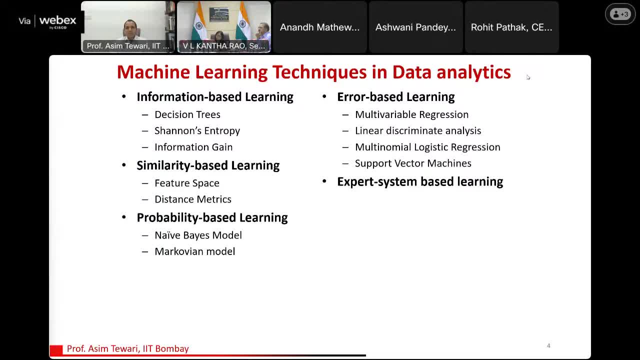 learning techniques which we were having, which were which were based on information theory, which were based on probablistic stocks and statistical learning and other kinds of techniques. there came a time in the history of ai techniques which were based on information. intellectual intelligence will just be something which will be far inferior than AI- artificial intelligence- and human capability and knowledge- Natural intelligence- are useful. intelligence will just be something which will be far inferior than human capability and human knowledge- natural intelligence- and will manage different受 samillest at you. so, based on the studies of AI, AI has taken up a lot of strugglinginations, have taken up these techniques. 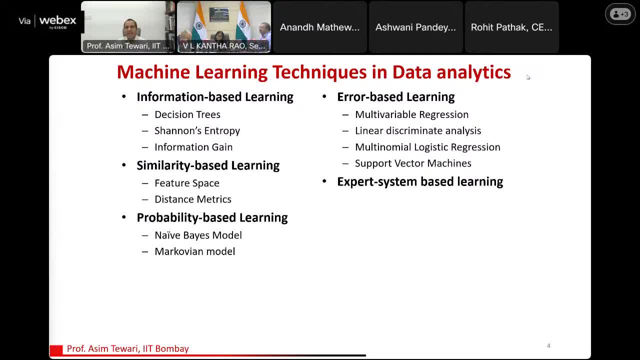 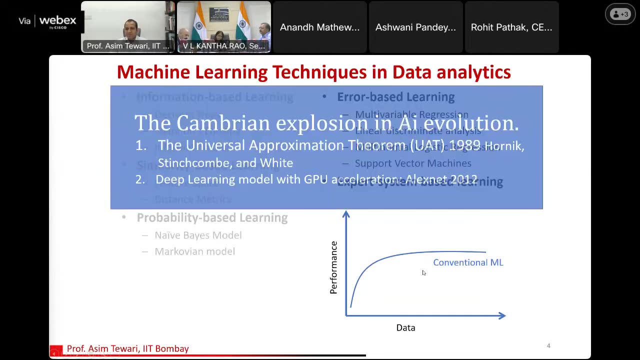 natural intelligence, So AI could never exceed natural intelligence, and AI is what was thought about. However, that changed And this was the curve which they saw for artificial intelligence and machine learning to do that. as you gave more data, the conventional machine learning became. 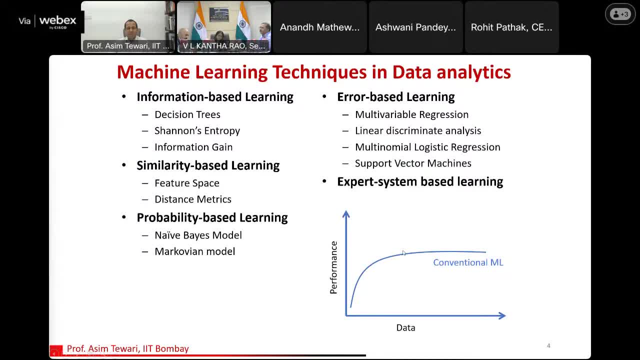 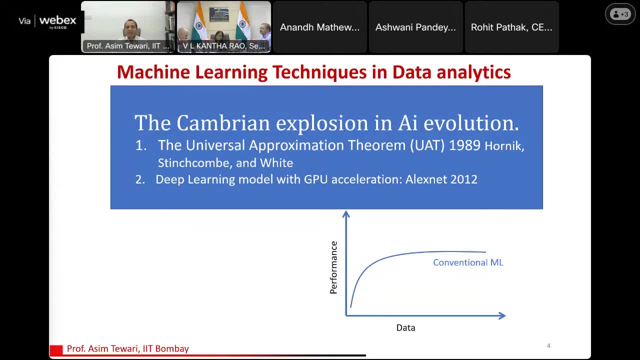 fixed and it could never have performance better than a level which was far inferior than human performance. But then there was a Cambrian explosion, in a sense in the area of artificial intelligence, Cambrian explosion is an event which happened in the history of Earth about. 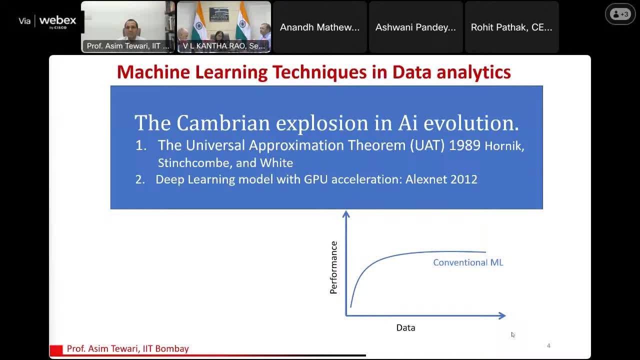 550 million years back, when the evolutionary process suddenly became accelerated by orders of magnitude. Species after species started evolving, new species started coming and the evolution became extremely fast. There are many theories which say what could have led to that, but there is no one understanding. 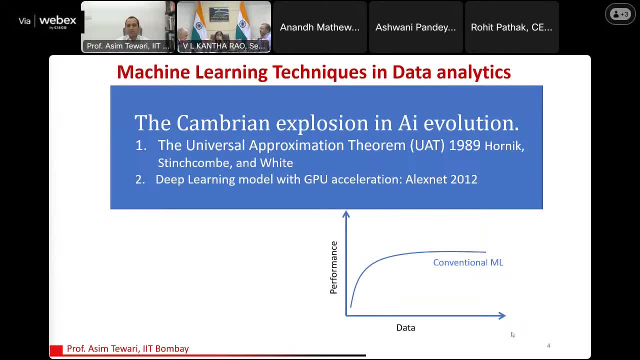 As to what really led to Cambrian explosion, but it is no doubt that that Cambrian explosion led to the formation of Homo sapiens sapiens- the humans. Had that not happened, we probably would have never come. So this Cambrian explosion happened on Earth in the history of evolution. 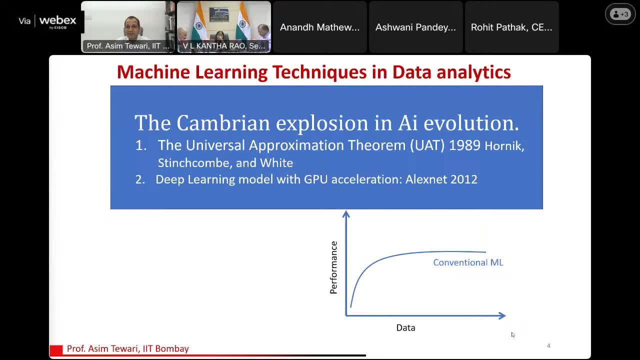 more than 550 million years back, but a similar Cambrian explosion happened in the evolution of AI. And this is started by a humble theorem which was proved in way back in 1990s- 1989 to be precise- which was known as Universal Approximation. 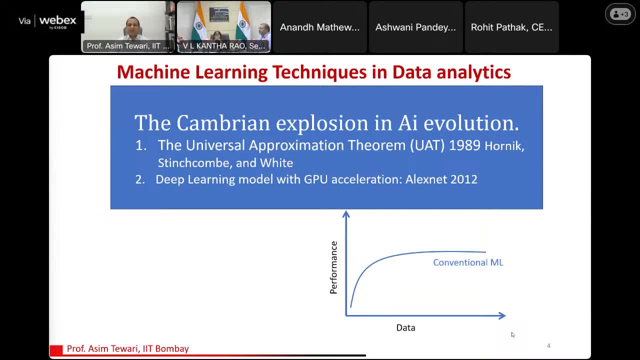 Theorem. This is the holy grail of the current machine learning. This theorem says that a deep learning model can assimilate and model any universal phenomena to any degree of approximation. There is no phenomena in the universe which cannot be modeled by a deep network. This was proved. 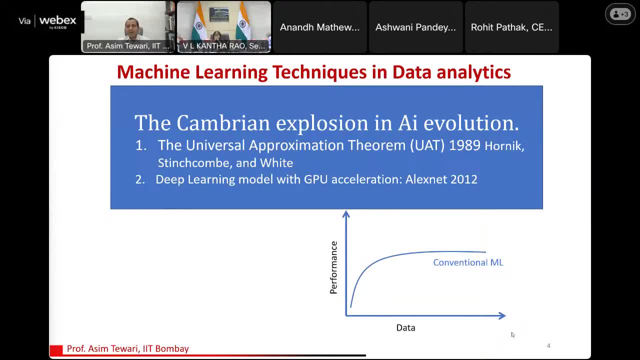 mathematically, but it was only in 2012 or 2010 when people were able to actually make it happen, And this was possible by hacking a GPU, a graphics processing unit, which was used for gaming, for PlayStations, Nintendo and other aspects. So this is where a hardware which was made for gaming 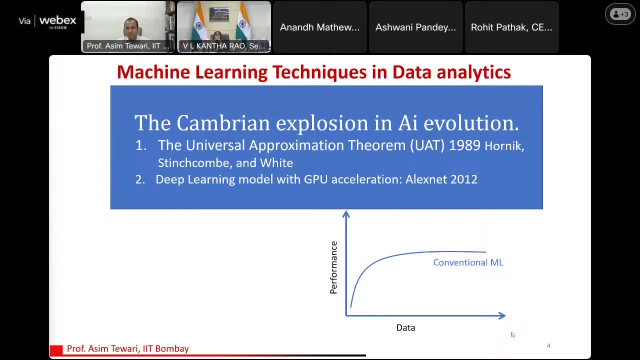 stations was hacked for deep learning, And this was the beginning of the current explosion which we see. And this is where deep learning starts. Deep learning is a phenomenon by itself. You feed it more and more data and give it more and more compute, and it will become more. 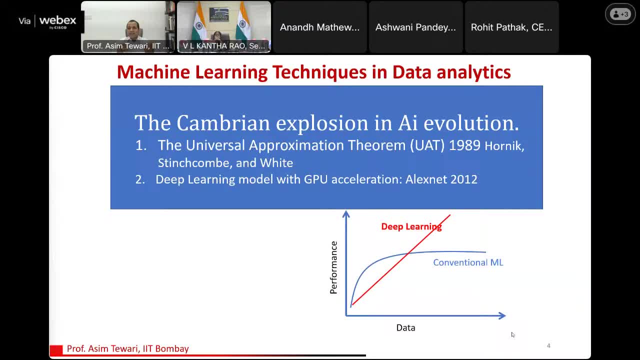 and more powerful. It's like you give fire fuel and oxygen and it will burn like a rage. So this is literally like fire and it is changing the world, and every year we were seeing things every month. we started seeing things. now, every week, we will see things. It is. 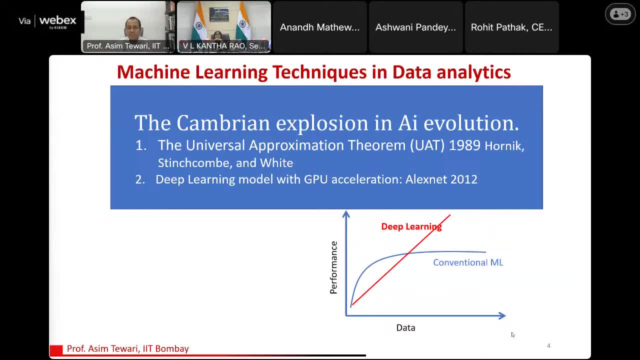 changing the world, and every year we will see things. It is changing the world and every year we will see things. So just imagine how fast things are changing. This is much, much, you know, a far cry from the the one and a half year for the hardwares to improve and double their computational power. 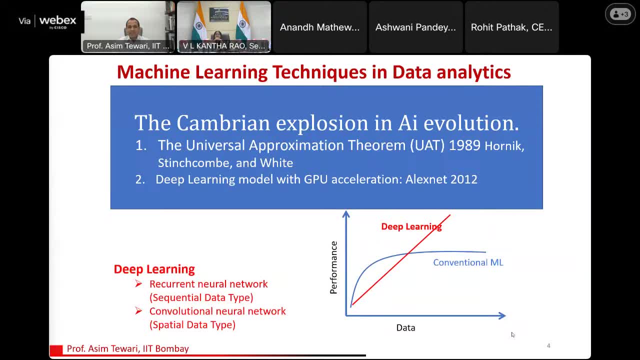 Now these are the two major algorithms in the deep learning network- recurrent neural networks and convolutional neural networks- which are leading the way. Recurrent neural networks are for sequential data and convolutional neural networks are for spatial data. Recurrent neural networks came and became well known with chat GPT, which is an unsupervised 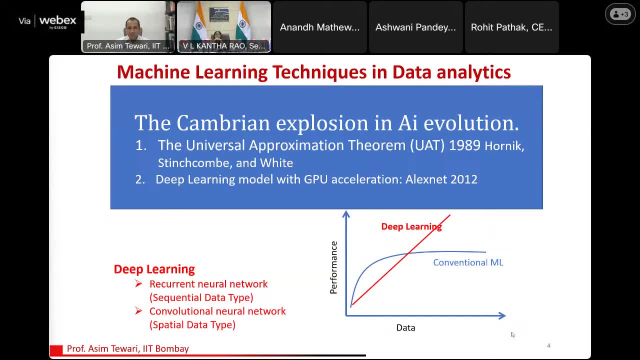 neural network, recurrent neural network based architecture, But what essentially they were doing was that they were able to surpass human capabilities, provided they were given enough data. Now one needs to realize that in fields where you don't have a lot of data, conventional machine learning models are still better. So if you see, if you have less data, 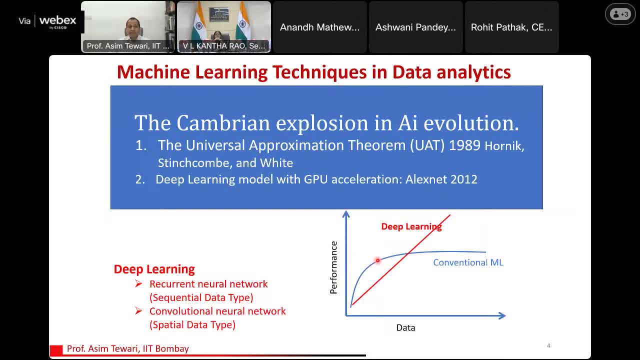 conventional machine learning models are far better than deep learning models, But wherever you have large data, deep learning models are far superior and they are- they are thought to to be- much better than humans themselves. And if you see, the convolutional neural network, which is for spatial data, is the kind of data which we have in geology. 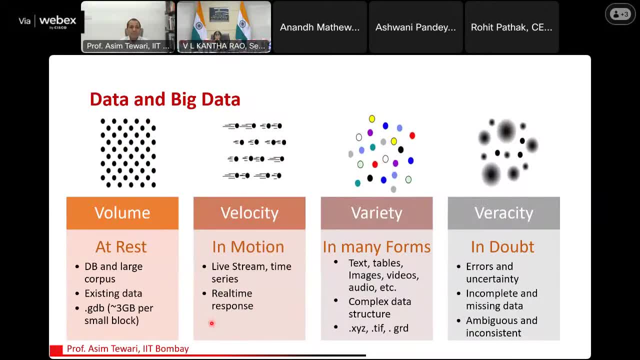 Now there is something which we have a lot of, which is data. My team has been done bytes and gigabytes of data for small, small blocks from the website, from the data repository which has now been made available, And that really is a huge challenge, because you 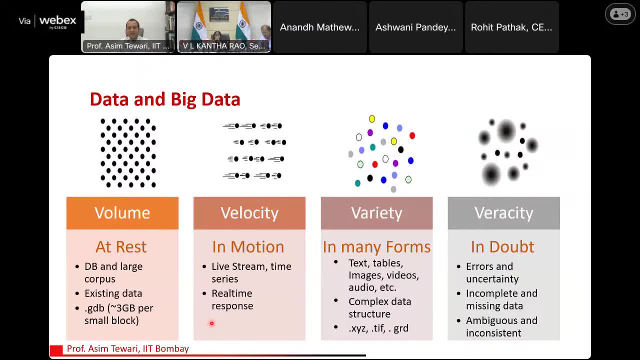 have so much of data that you do not know how to handle it. As a matter of fact, we expect more than four petabytes of data to be to be used for our- our eventual models. I wonder how bigger data center would be requiring. So we have just done some basic estimates. 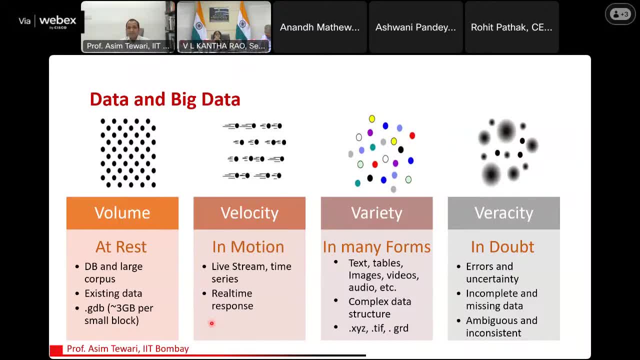 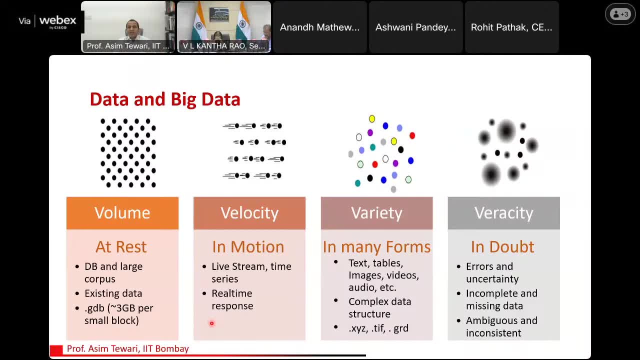 Anyway, nonetheless, we essentially are coming face to face with the problem of big data. Big data is when you have very large volumes of data, For instance, the dot, GBD files, GDB files which you can download from the, from the repository of of uh, our geological data. 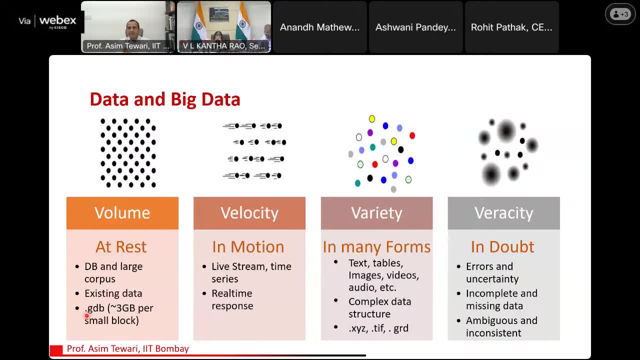 a small block would be would be at a lower resolution or a medium resolution. We have about three GB, three gigabytes. Now, just imagine if you have to use your network to download such an amount of information. it would be about three gigabytes. Now, just imagine if you have to use your network to download such an amount of information. 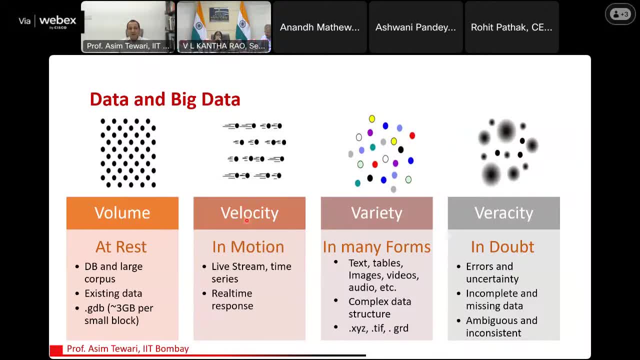 That itself could take a very long time. Then, of course, there is not much velocity. Things are not changing every day that fast. However, they do have a huge variety. So we have text data, We have data which is digital, We have data which is in X, Y, Z format, images, stiff format, dot, grid format. 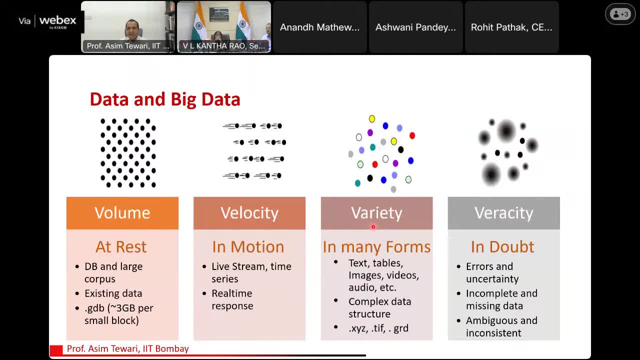 So there are multiple different kinds of data which is available. Large volume and variety makes the data very, very, I would say, challenging in some sense. But the biggest challenge comes to from veracity, as you would know that the data is very sparse and discreet and also sometimes 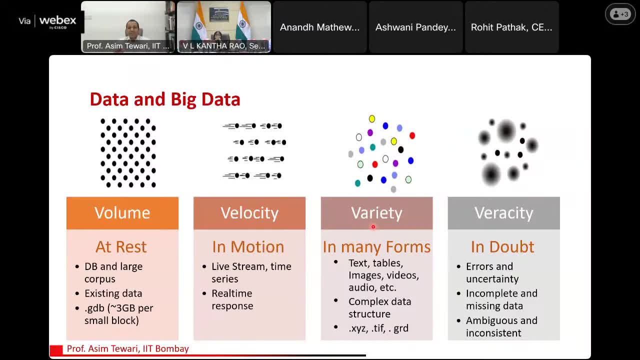 error prone. Now, in this specific case, we have a specific solutions which we have come up with, which can handle veracity in a very structured manner And, as a matter of fact, can use it. So what I'll do is I'll show you some of the examples of how the world has been using this. 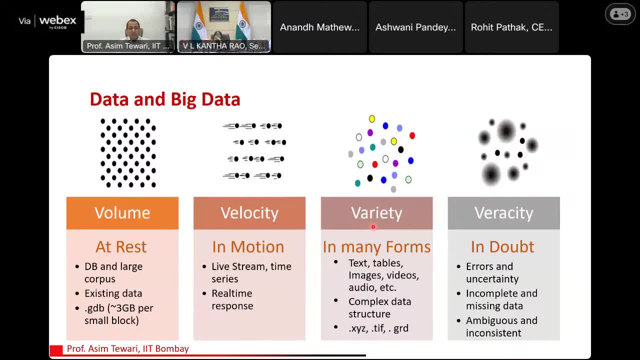 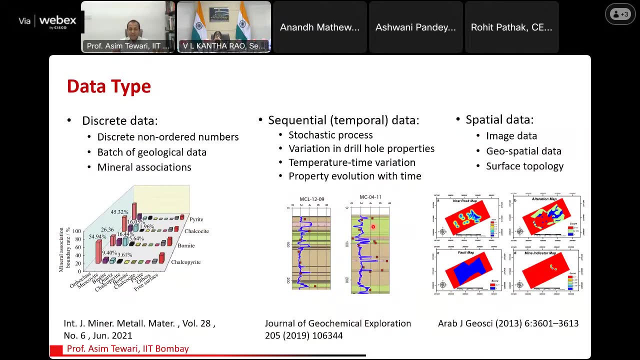 big data for their individual mineral explorations, And then I will give you the framework. I won't show you the real data. I'll show you the real data. I would not. I would not show you the real outputs of the data. So so, this is how the world has been looking at the data: discreet data. 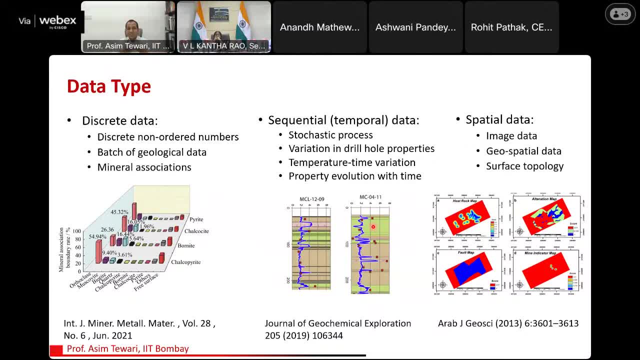 spatio, temporal data and spatial data. So these are the three basic kinds of data sets which are primarily used in our mineral exploration. Discrete data are data which which are a specific geological information coming from texts and literature. 00.07.33. 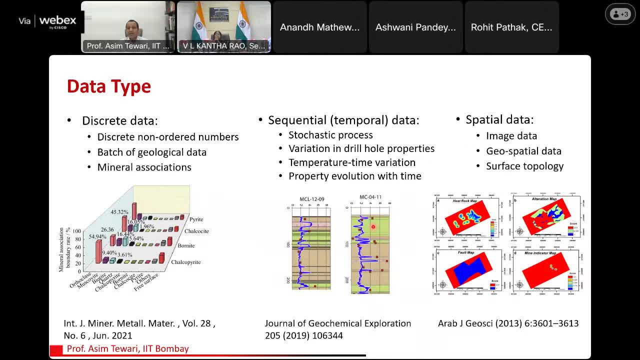 and other aspects of laboratory experiments. sequential data, in this specific case, comes primarily from drill holes, because you have now deep holes where the data is is, you know, available. it's not that you have mines, which are surface mines, and that is a very important aspect, because to be able to extract deep drill hole data, you have to learn and adapt to sequential 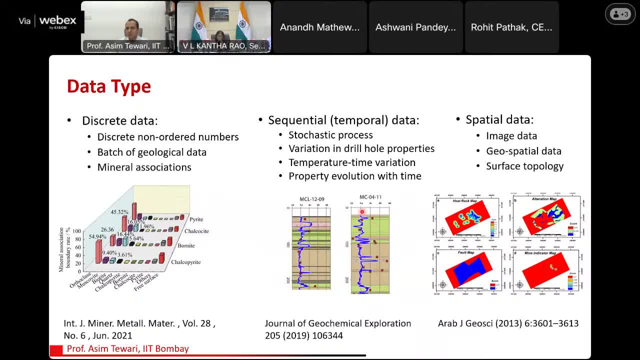 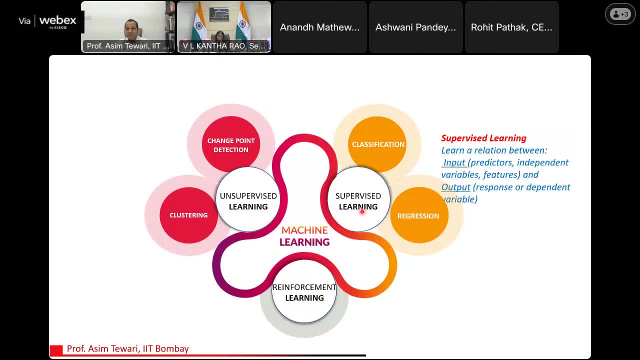 data coming from that and the spatial data i just talked about, images and all the geospatial data which we have. and in this now what is happening is that we have been, in the beginning, looking at supervised learning in machine learning. there are three basic aspects: supervised learning and 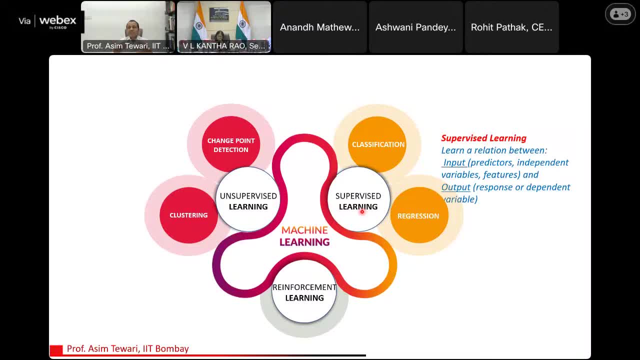 unsupervised learning and reinforcement learning. supervised learning is when we train the data set based on known mineral exploration successes. so if we know there has been successful exploration and we have been able to mine these, these locations for these, these minerals, we use that input and output. the input is all the spatial data. 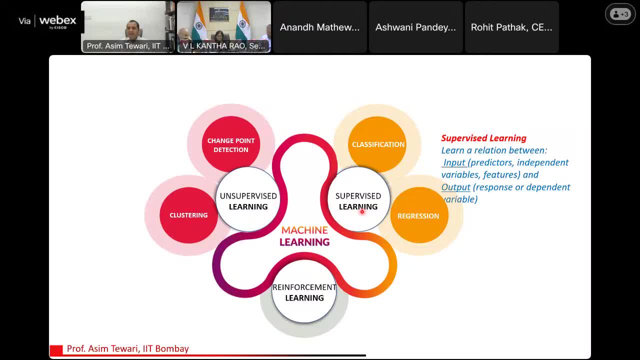 geological data and other data which i'll just talk about a little bit in, and then the output is where we have been able to successfully explore things. however, as you know, we have very few places where we have been able to explore. thus, we also use a lot of unsupervised methodologies, and these 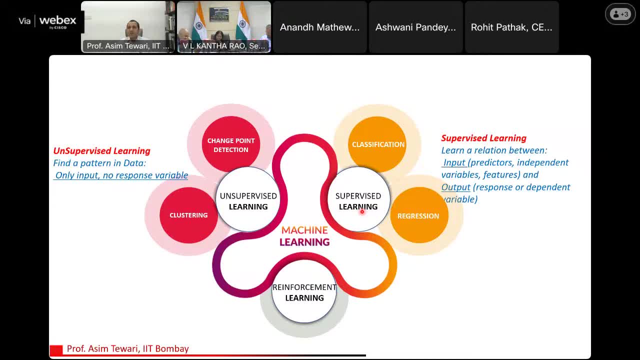 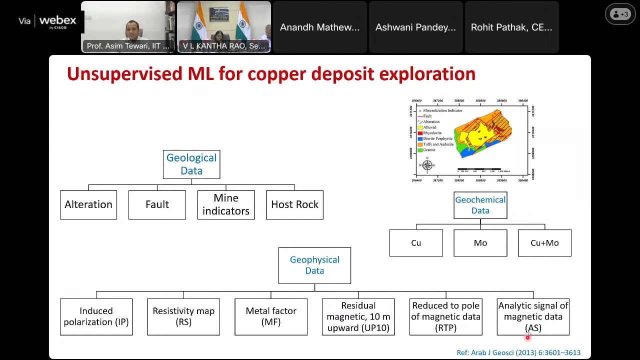 are really powerful. they are very, i would say, green field, because you really don't need any past data over there. however, there are, there are possibilities of they- they identifying large sets of uh possible sites, much bigger sites than what a supervised learning could do, just to give you an unsupervised model which was very successfully uh, you know, used. this is: 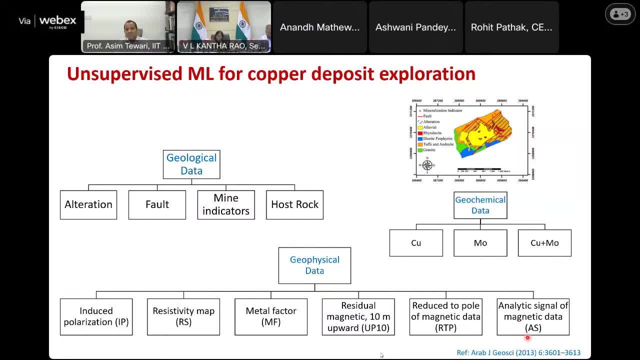 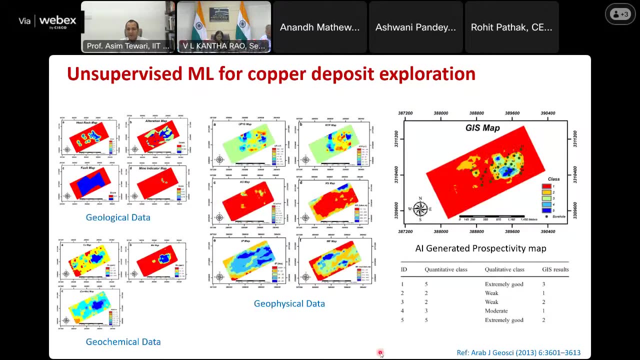 the one which was used by combining geological data, geochemical data and geophysical data, and it was able to look at copper deposits without necessarily having any output labels of copper deposits. so this was a very unique methodology which was used and based on that one could classify extremely good areas, weak areas and moderate areas on a physical map. 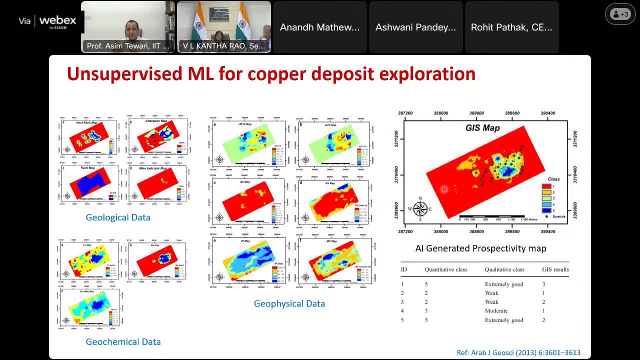 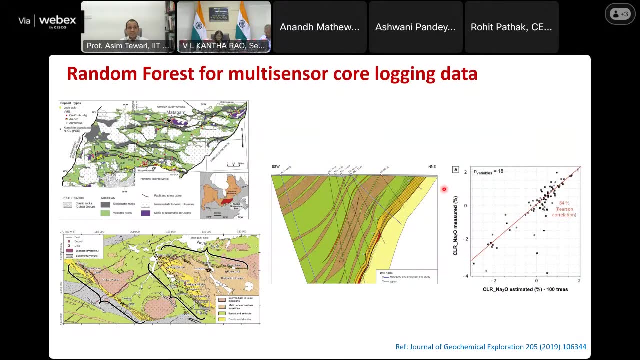 this can narrow down your exploration to a very, very small, targeted regions where one can then finally do do ground exploration and figure out what it is. it is expected that these explorations could range anywhere from 50 to 70 percent success. now, this is coming from the, the aspects of deep hole sequential data, where aspects of 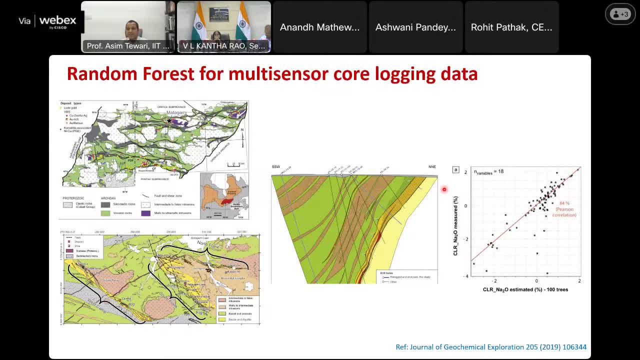 and xg boosts were used, where the right side image shows that the estimate versus the actual value seems to show a pretty good correlation between them. now this is where you need to realize there is an underlining geological structure which need not be known beforehand, and thus your deep holes. 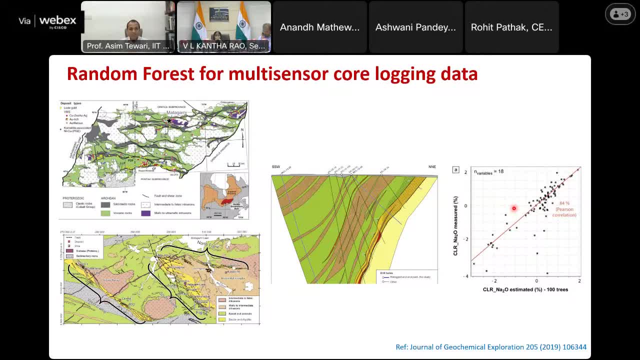 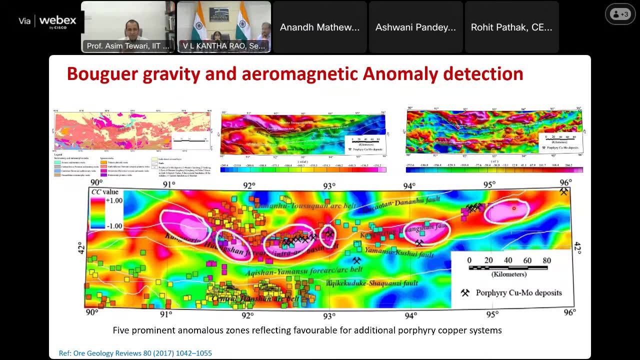 are only giving you sequential data, but you could use that along with the spatial data and come up with a model to figure out how the base will be changing. this is probably one of the most celebrated- uh, you know, i would say- thing coming from the gobi desert, from chinese publications. 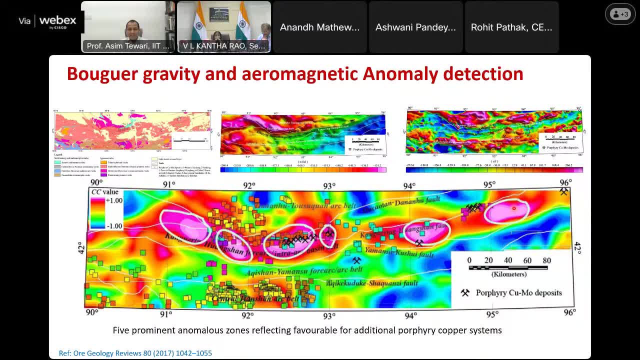 in which they were able to identify five prominent sites for copper systems. this was supervised, however, because they had several mines already known to them, and that really helped them identify five other locations which they found might be even better than what they currently have. these bad black crosses which you see are where the deposits have already been found, and these white 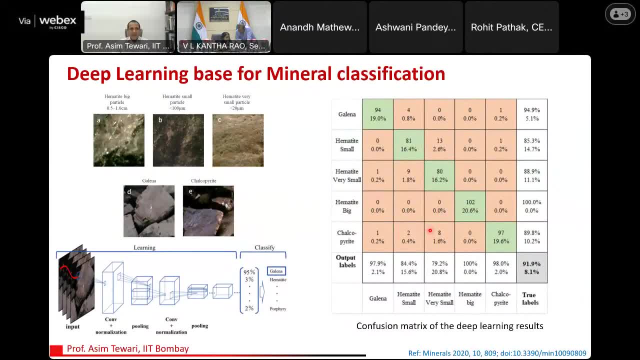 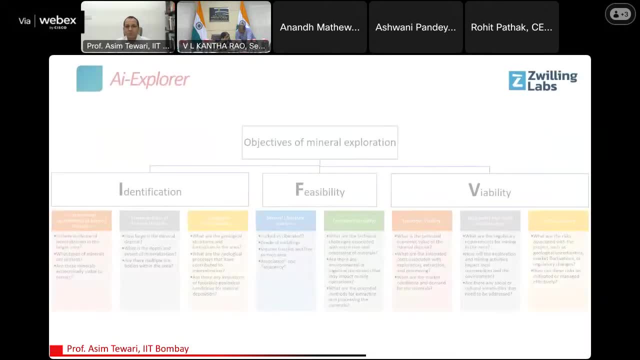 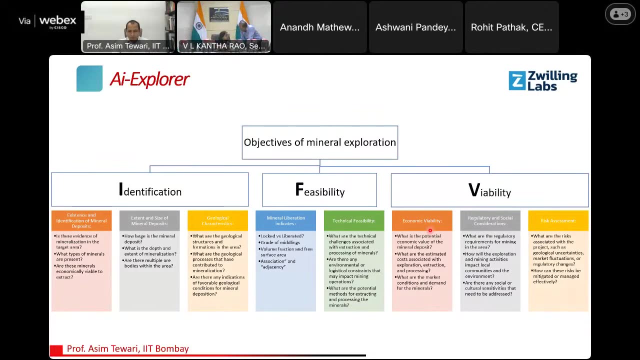 circles are where they were able to find that, and similarly deep, deep learning based mineral classifications and aspects of how easily it could be explored. so, just coming to what really is the objective, so this is a startup company in in iit, bombay- and i'm now last slides, i think. so this is where, uh, this company has been. 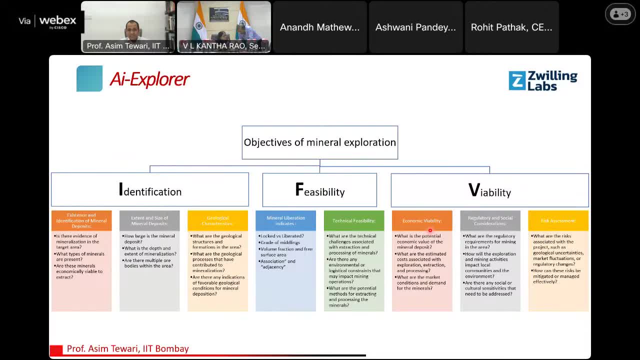 looking at objectives of identification, feasibility and viability. this is a a technique which they have developed, which they are clubbing under ai explorer, where it identifies existence of deposits. it looks at extent and size of mineral deposits and geological characteristics. that is under the identification. for feasibility, it looks at mineral liberation indicators. can you predict? 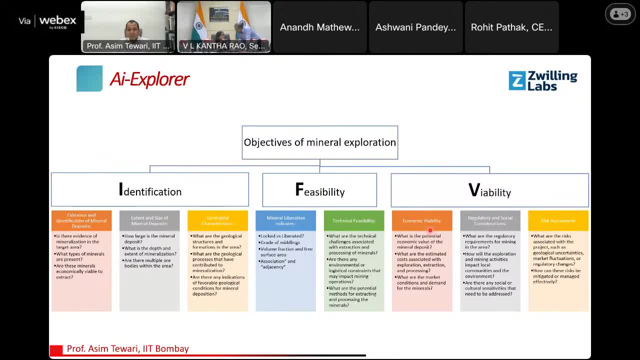 that. can you look at the technical feasibility and and how you would be able to beneficiate the minerals? and finally, the viability: is it economically viable? is it compliance? are the compliance requirements? are the compliance requirements? are the compliance requirements with respect to regulatory and social considerations, economically as well as? 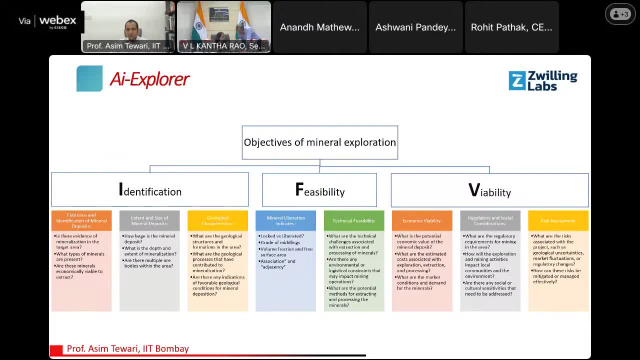 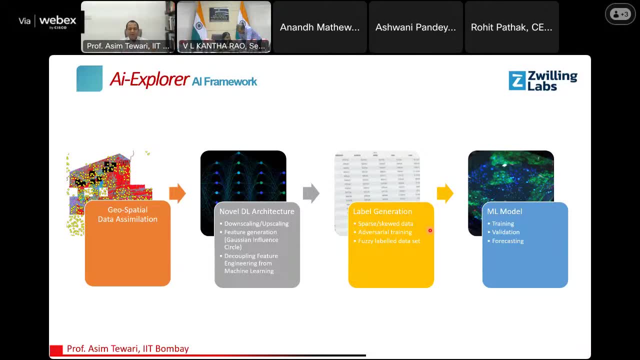 environmental considerations and, finally, risk assessment. so the way this ai explorer works is that it has a very unique framework where they're using a combination of deep learning networks along with conventional machine learning models. so what it does is that it takes geological spatial data and, just to say, give you a sense of what kind of geological spatial data is being used. 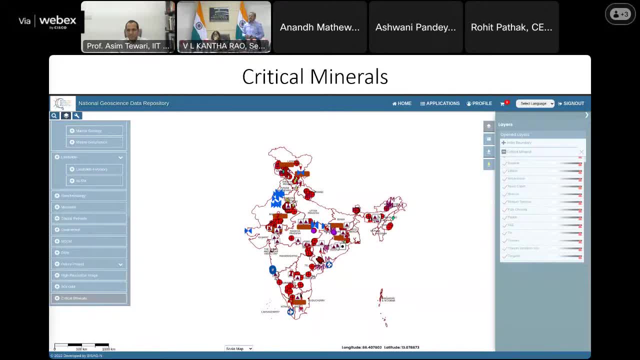 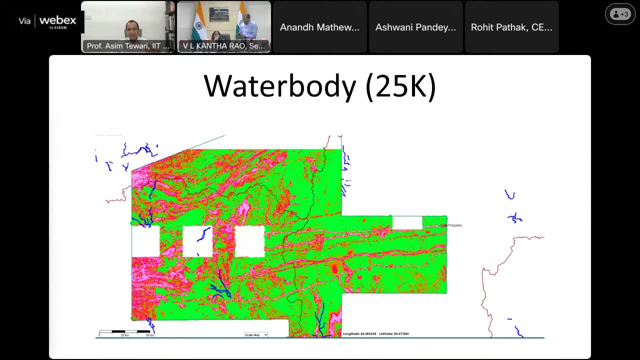 so this is, of course, coming from our national geological science data report repository and, as you can see, you could have multiple different kinds of data coming from it. so i'm just skipping very quickly. but what i'm trying to say is that all of this data and this 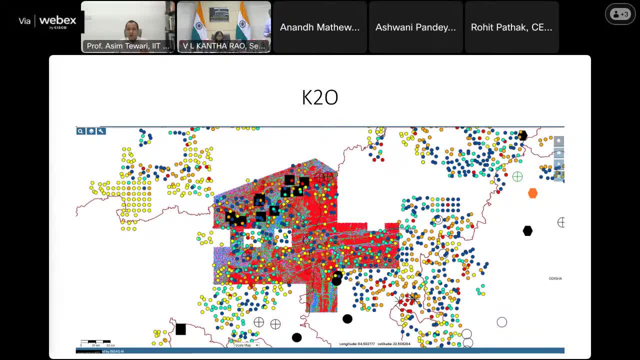 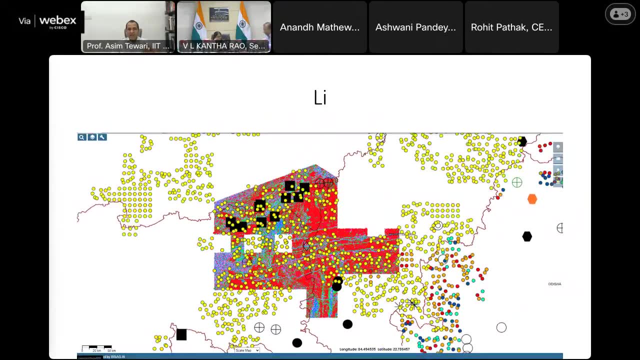 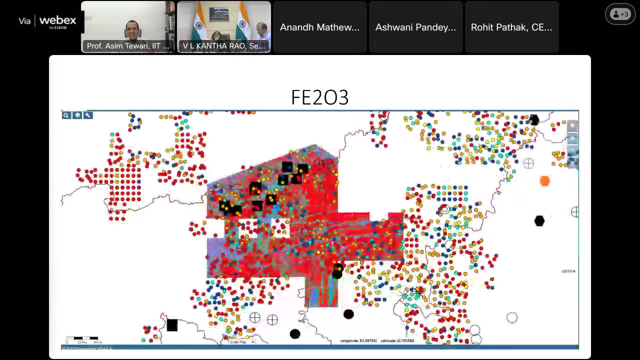 is just for one block. i'm just showing a case study for one block, which is block four, and we are superimposing various kinds of geophysical, geochemical, soil, geological and other features and i'm just switching through this to just second give you a sense of what size of data is being used. 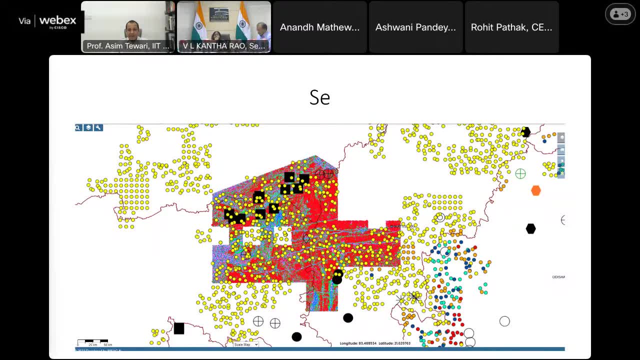 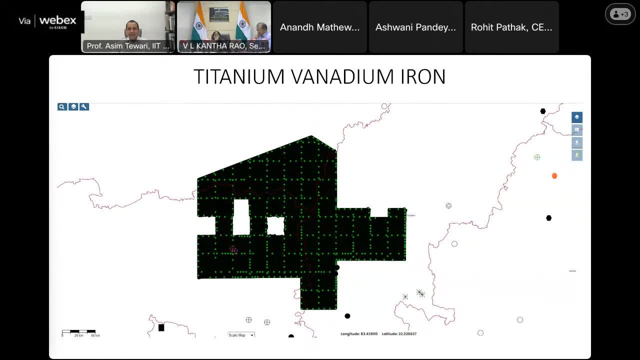 and this is at a scale of about 50 kilometers. we can, of course, go even finer, because the data at many locations is much finer than this- and you start looking at this data and you start looking at various elements at the same time, and and then you, you are able to superimpose all of them. 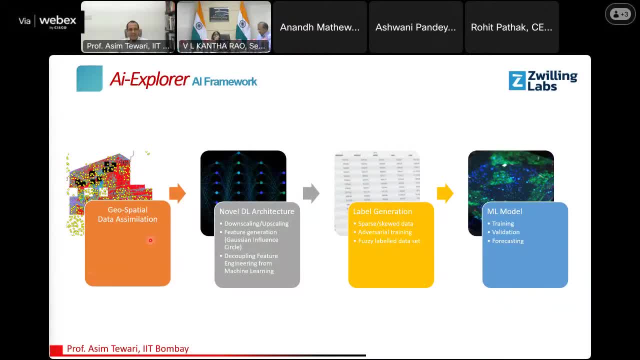 and to create that, you start by data assimilation and then we have a novel deep learning architecture to extract features from it. so here the deep learning is being used in a different manner, and this is a very novel way of using deep learning, because we are not 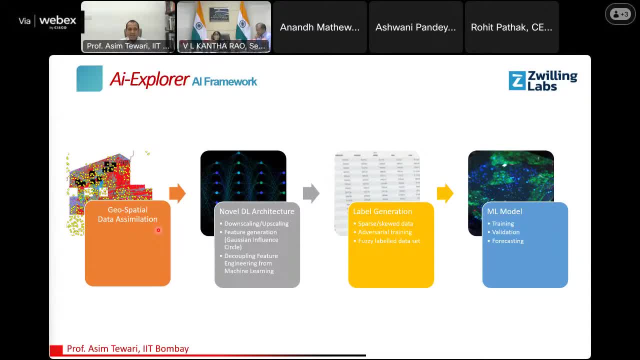 using deep learning for classification of regions which are high in mineral deposit or not. we are actually using deep learning to create features. these features are then used for machine learning models, and here there are two aspects. new features are being created using a deep learning architecture. they primarily do downscaling or upscaling, depending upon what data they have. then they use 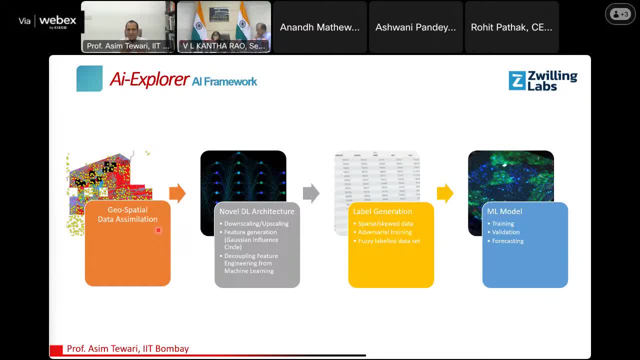 something known as a gaussian influence circle, because what you are looking at is that it's a grid. you have data points on a specific grid, whereas the mines could be at different locations, and you need to couple the two together, and by doing this we are able to decouple the feature engineering part from machine learning part. 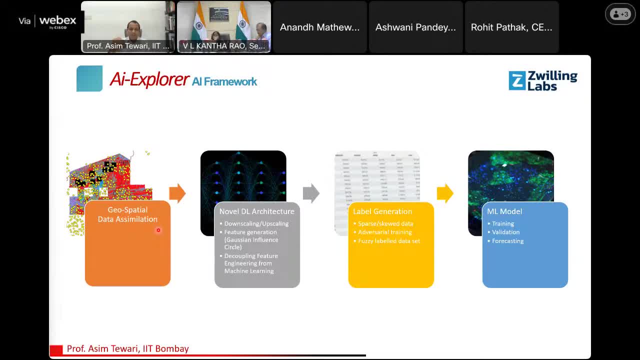 these features. once they are engineered, they could be labeled for. they could be used for any training, and thus we have a different labeling generation step in the in the ai architecture. the biggest challenge i would say with the data is that the labels are not enough. it's very sparse and skewed. you only have successes where you have. 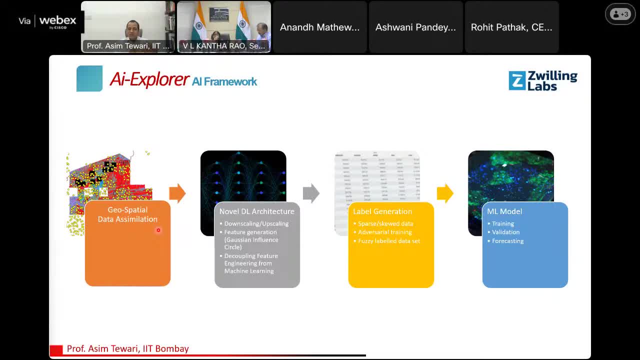 been able to find minerals, if we are able to also create data set of regions where we did exploration on the ground but did not receive any any mineral of a specific kind, if that data is put, it becomes very powerful for machine learning to figure out, because machine learning doesn't want to only know. 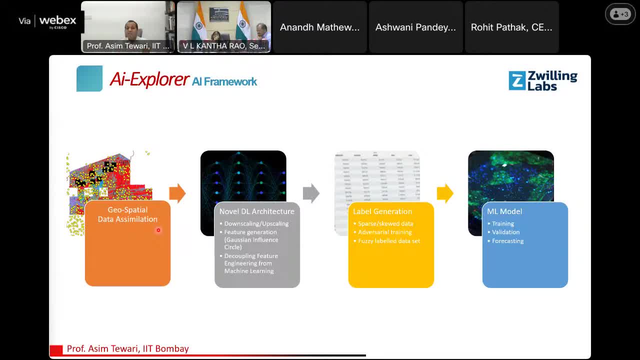 where you can find something. what also does not work is very important, and that is not really right there. right now, however, we have a methodology to do what we call as adversarial training, so we create a label data which is adversarial data, and we also create fuzzy label data. we don't. 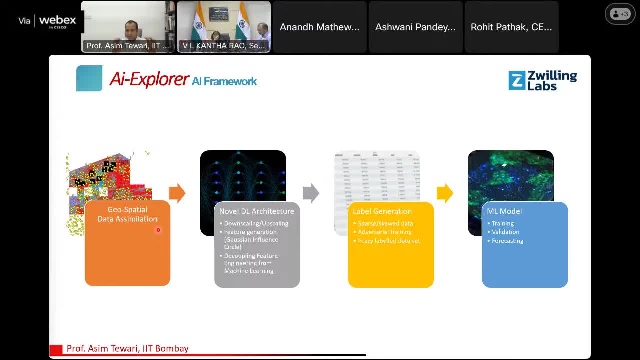 take a black and white data. using this, we create features and labels, and then we use machine learning- conventional machine learning- for training, validation and forecasting. eventually, this will provide you a forecasting which will tell you on the spatial map what element at what level is possible at what region. 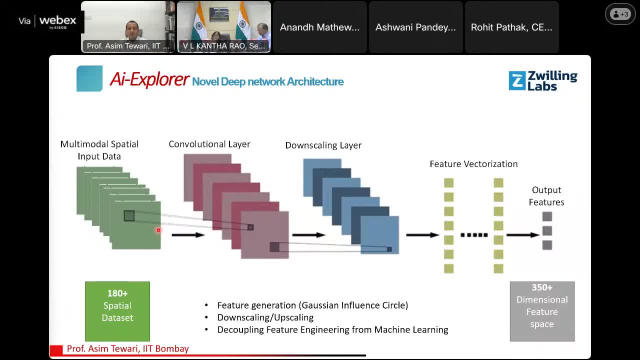 this is a a high level overview of our deep network architecture. we are having over 180 spatial data sets for a single block, which is 180 high resolution images, which is showing the xy variation. and then we perform multi-modal spatial input data convolution, which is using the gaussian 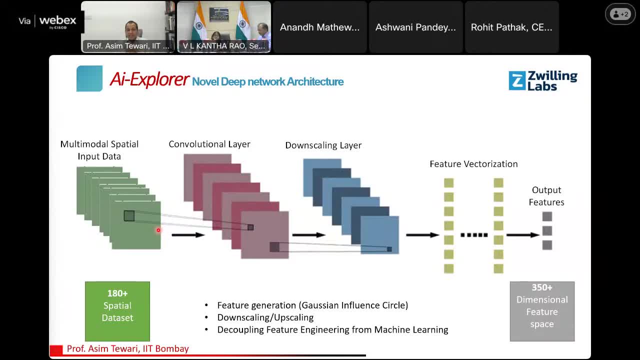 influence circle, and then we perform downscaling or upscaling as the need be, and then we create decoupled features. we have over 350 dimensional data set coming out of this. now this data set has been already trained to be features which are most relevant. this is the most computationally intensive process. 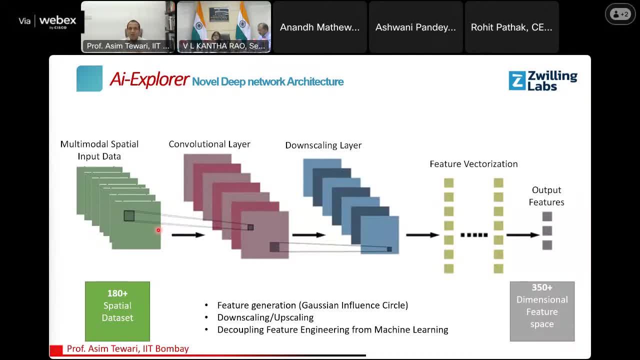 a small sized region could take about 80 hours on. you know two, two, let's say rtx 40, 90, uh, 24 gb trinity gpus. but once you have these features, you can use this again and again for doing all your machine learning on top of it, which means that you don't have to go back and spend that much time. 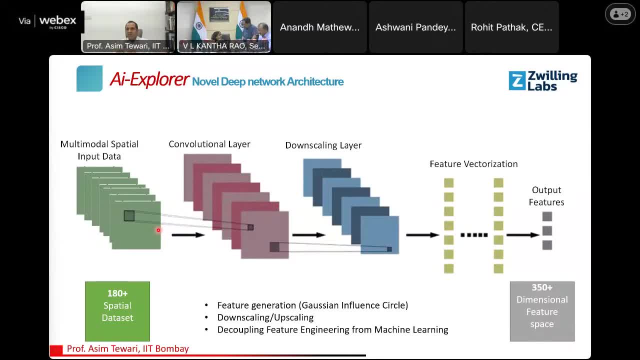 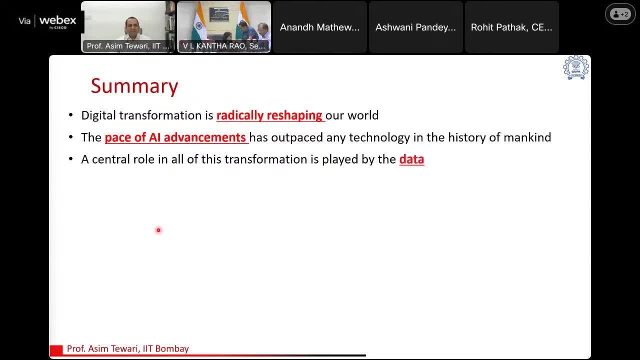 you want to now use these features and the label data separately. the commercial machine learning models are much faster that the digital transformation is radically reshaping our world. the pace of ai advancement has literally outpaced any technology, and the central role is being played by data, and thus there has to be a fundamental shift from our traditional technology. 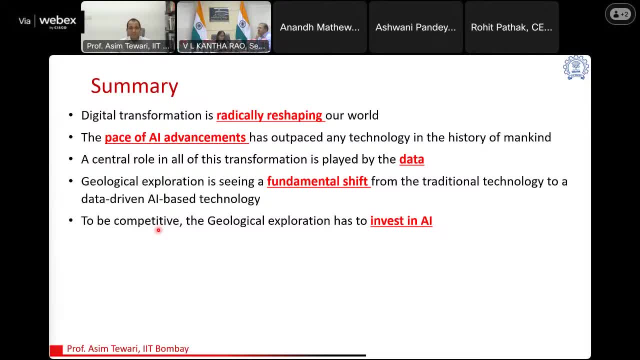 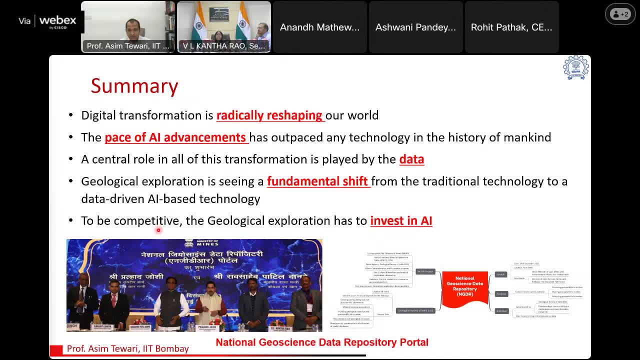 technology to an AI driven data technology, and that really is. is there a fact for geological exploration? so we have to invest in the geological exploration and I think this is a fabulous step which the ministry has taken moving forward, and I see AI can transform the way we have. 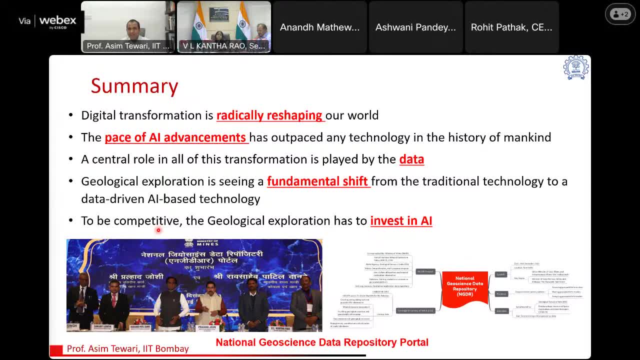 been. we have been exploring for minerals and India is an unexplored, large, vast majority vast area and not just land. we are looking at sea as well. so we have huge maps from the sea and all the Indian Ocean and the Arabian Sea and we really would be able to perform. 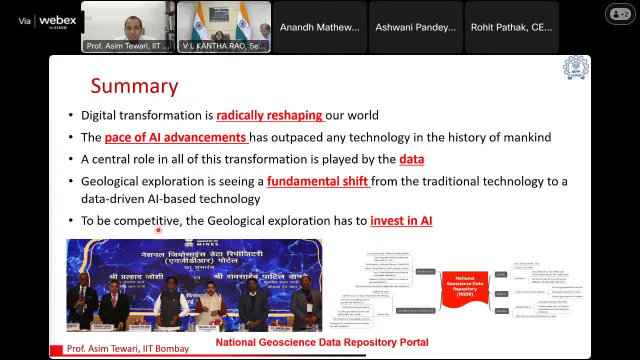 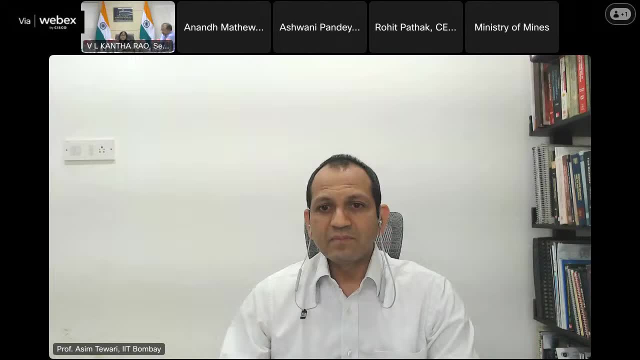 the deep exploration and see as well using AI. so with that I'll stop and I want to thank ministry and and for you, madam, to give me this opportunity, thank you. thank you, professor Tiwari, and for your detailed description about the AI in the mining sector, and thank you. 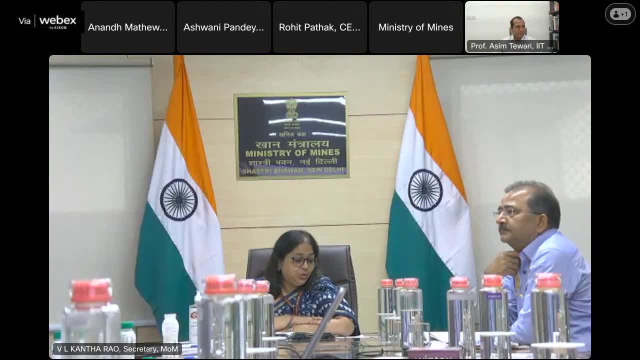 for your time and thank you for your time. thank you, thank you, you're welcome. thank you and thank you for your time and thank you for your time and thank you. thank you for your. we would like to connect with you in the future also and would like to use your ai in data analysis. 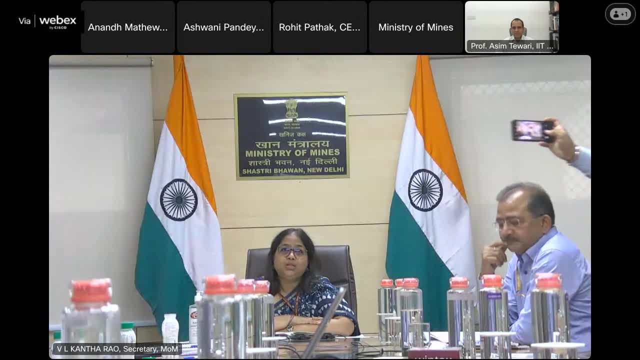 and mapping of our data. i will get back to you on this, uh separately, thank you. move now to move forward. there is a question and answer session, but this being webinar and the large number of participants uh joining the webinar, uh, maybe giving the option to speak to all is difficult. 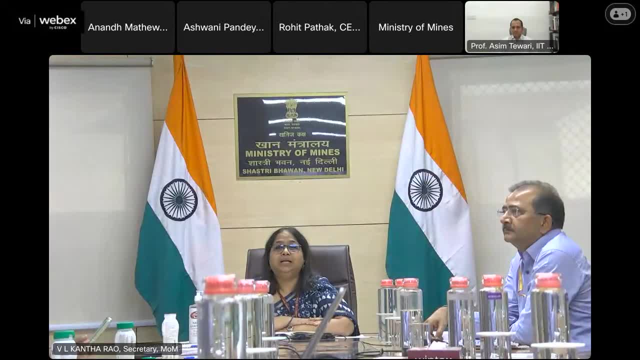 so we have made it available through the chat box and i request all the participants to give their, leave their questions in the chat box and we'll get back to you on this uh with the email ids. we will on the email ids uh from which you have connected uh to this uh webinar, we'll get. 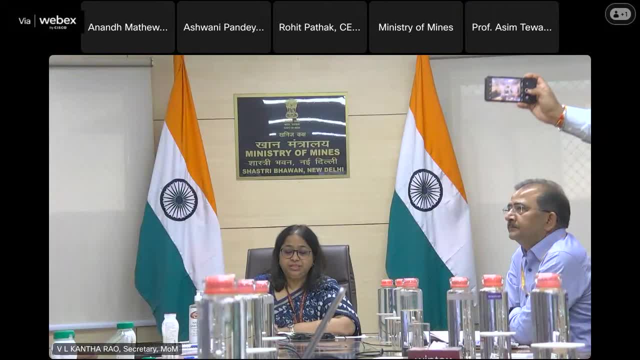 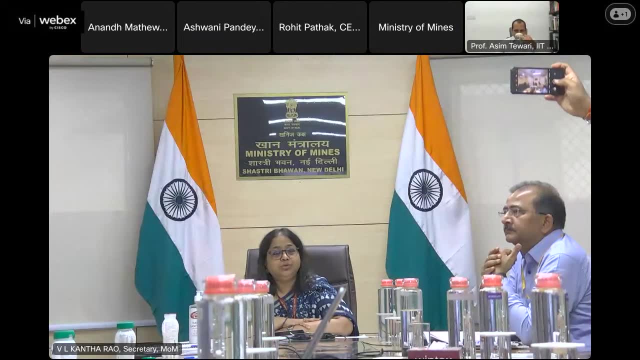 back to you on on all this. just to sum up the session uh quickly, because, uh, there's another meeting to be held here. uh, i would just like to thank all the participants. i personally feel that this is a very uh good uh session. uh, i'm sure that all of you must have learned from this uh experiences of all the. 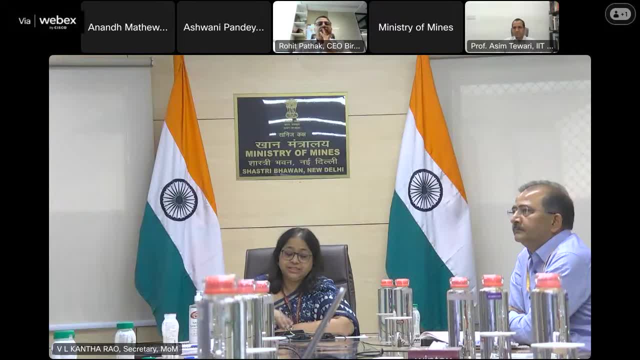 speakers who have spoken here. we have just given the uh poll also in this webinar and the results. i'm very happy to see that some of the- i mean it gives us a satisfaction that we are moving in the right direction- like very heartening. what i felt is 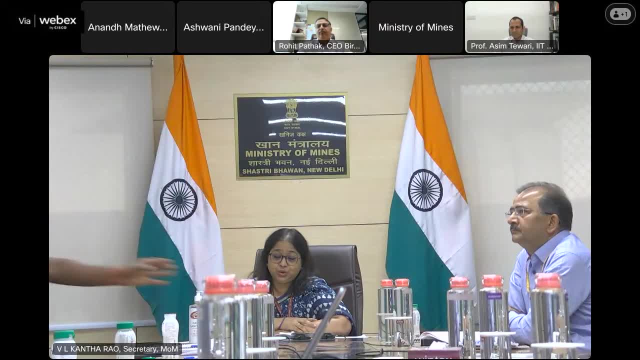 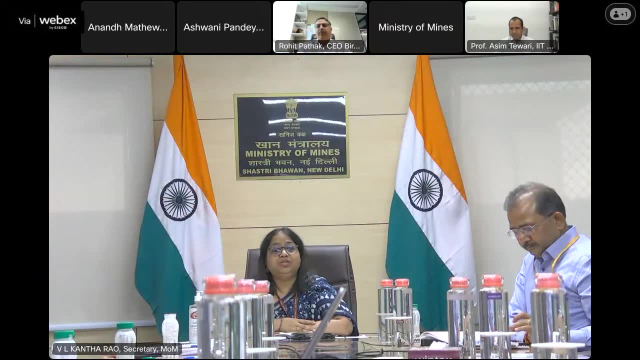 that the people have said that what motivates them is the creativity and innovation that drives startups to for the entrepreneurship and uh funding is one of the aspects which almost all majority have said that is a stumbling block in the scenario. so we uh are happy and we ensure that. 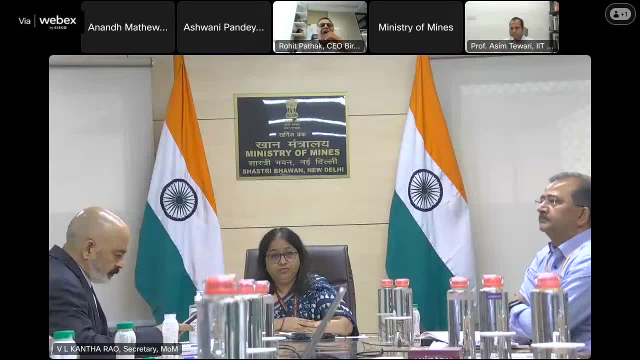 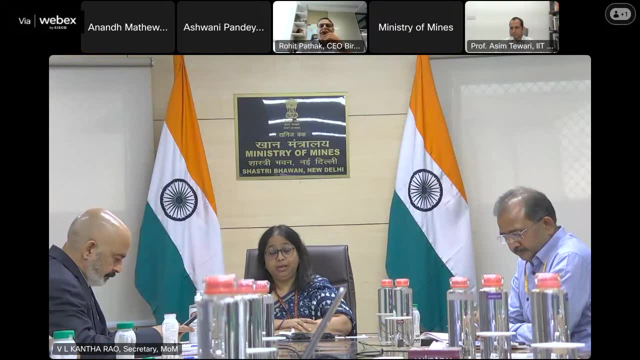 uh. we are here to take care of this uh funding aspect of the startups, and my request to all the incubator centers and the people who are manage these incubators centers is to encourage your uh uh students and the startups connected with uh the incubation centers to apply for this. 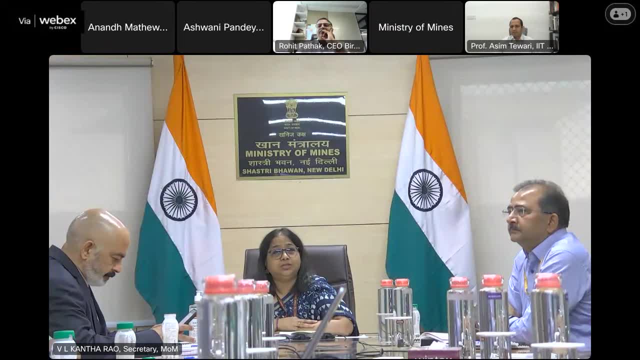 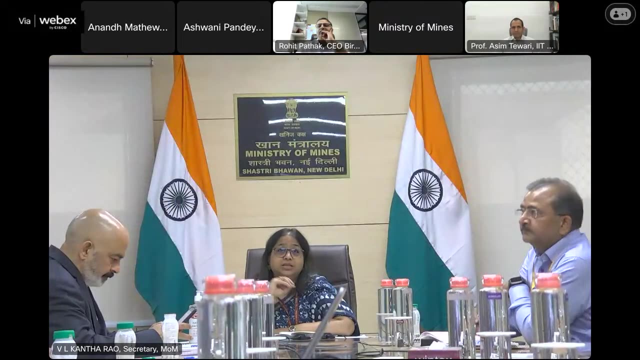 our efforts will be. we have already have a trust area on the uh satyabama portal and but uh we will be working with the a group of academysh here to find out and the industry to find out the uh specific problem areas for which uh the industry. 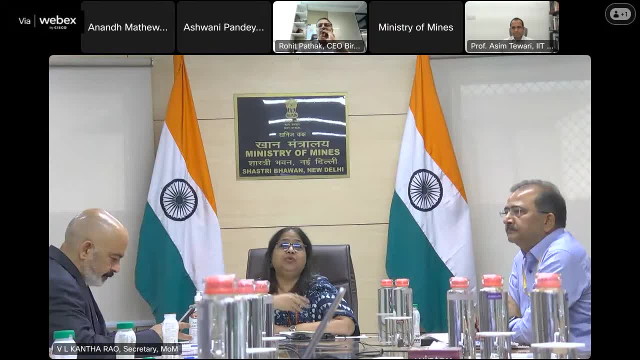 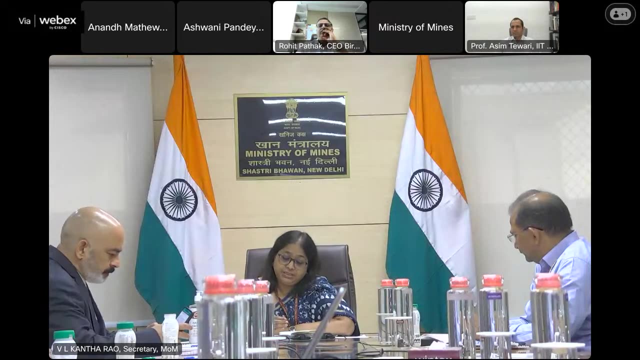 is looking for a solution so that it becomes easier for uh the people, the innovators, to provide solution in that direction. and i would also like to inform you all that uh, this present uh, uh crunch, the uh date is till 30th april, but this is not the only uh time that we will be doing. 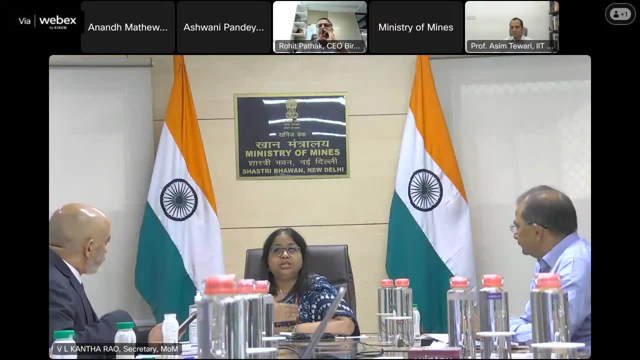 this. we have decided that we'll be doing it every quarterly or six months basis. six months basis so that, uh, people who are not able to submit the proposal right now will be able to submit the proposal two, three months later. so it all depends upon the, uh the amount of proposals we receive. 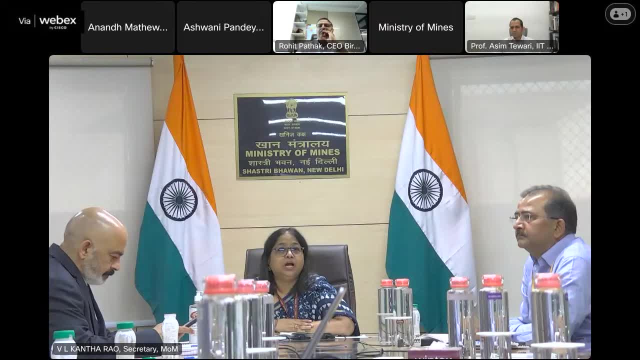 we will be doing our best to accommodate and accept the proposals which are promising in nature. and, uh, do it quickly, as we have done it in snt prison first. thank you very much. if anybody would like to say from the speaker anything else, otherwise we'll close the session. 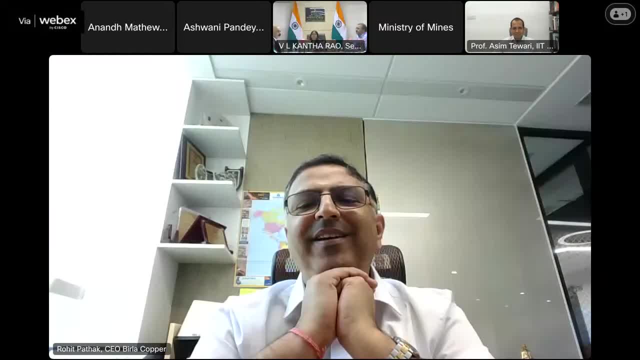 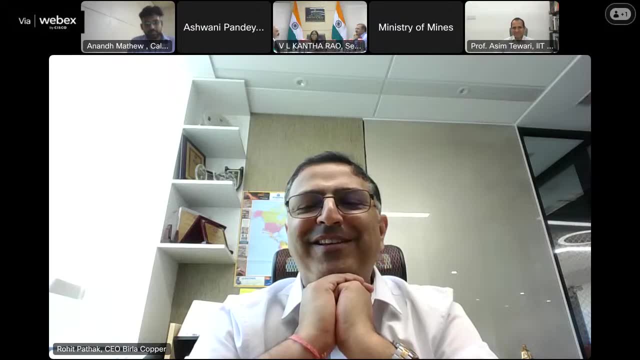 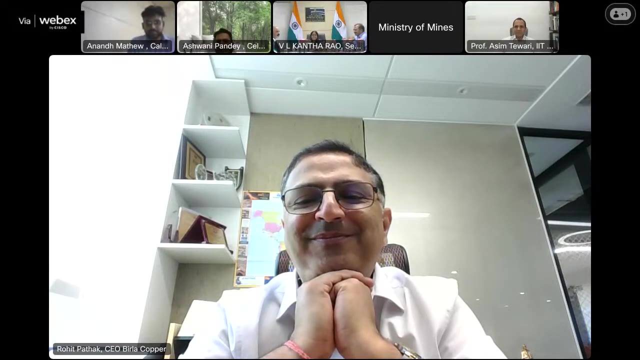 thank you so much and i think really, uh, i must say this is one of those areas where i'm saved, because it is a very small area, feeling the government is becoming faster than the industry. so good to be in that position and you know we'll fully support you as you drive this. thank you, because, see, it is we are doing.